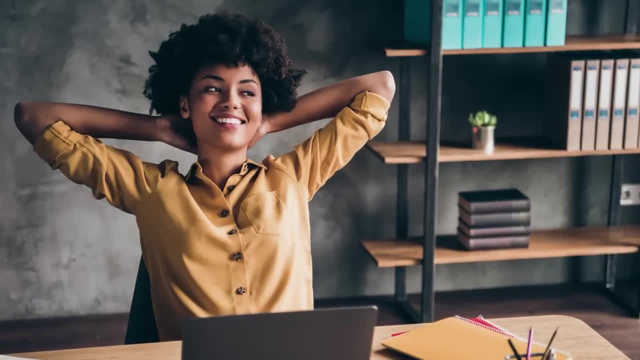 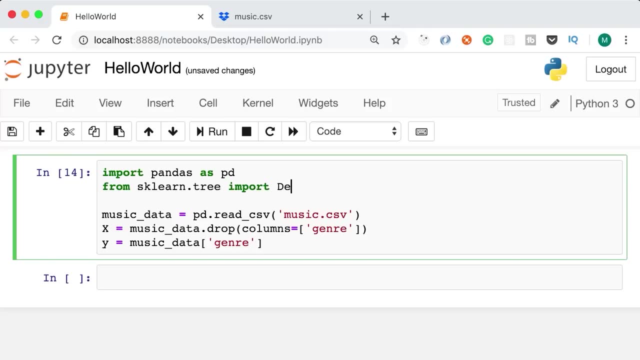 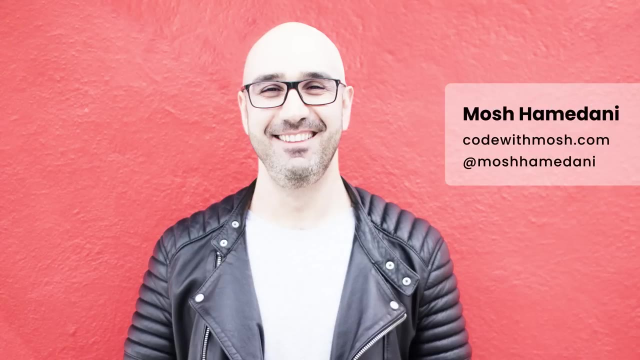 learn more intermediate to advanced level concepts. You don't need any prior knowledge in machine learning, but you need to know Python fairly well. If you don't, I've got a couple of tutorials for you here on my channel. The links are below this video. I'm Mosh Hamedani and I'm super excited to be your instructor On this channel. I have tons of programming tutorials that you might find helpful, So be sure to subscribe, as I upload new tutorials every week. Now let's jump in and get started. 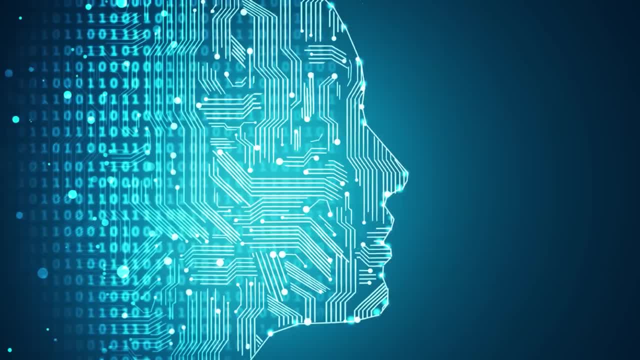 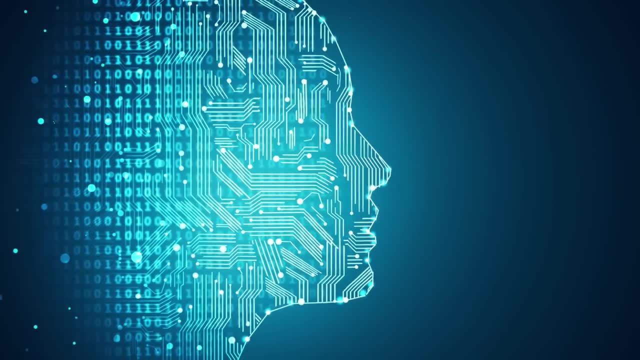 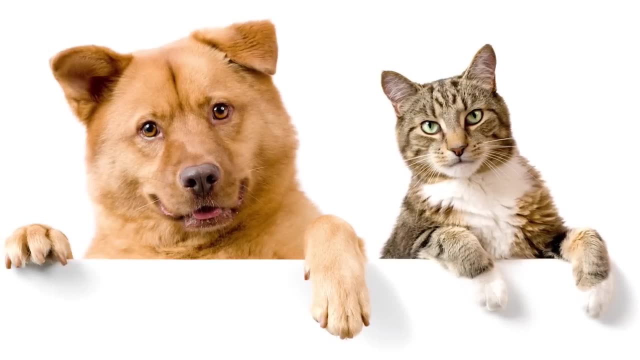 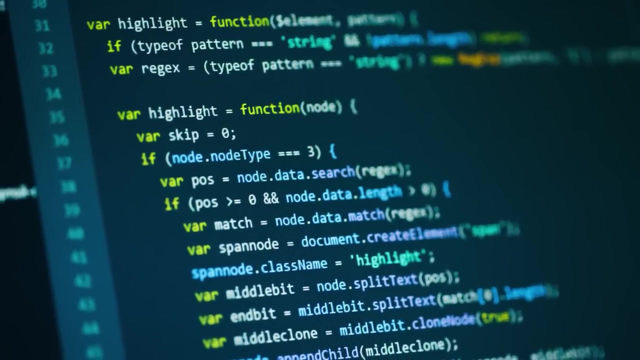 In this section you're going to learn about machine learning, which is a subset of AI or artificial intelligence. It's one of the trending topics in the world these days and it's going to have a lot of applications in the future. Here's an example. Imagine I ask you to write a program to scan an image and tell if it's a cat or a dog. If you want to build this program using traditional programming techniques, your program is going to get overly complex. You will have to come up with lots of rules to look for a specific program. 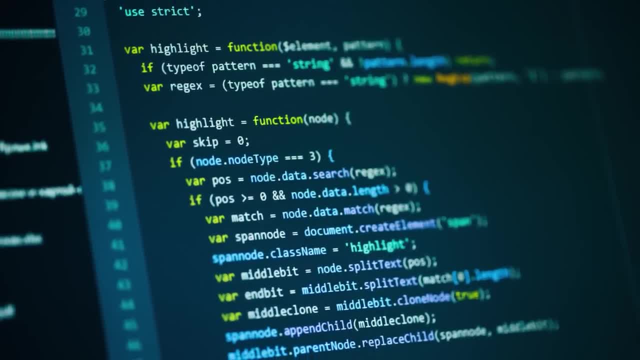 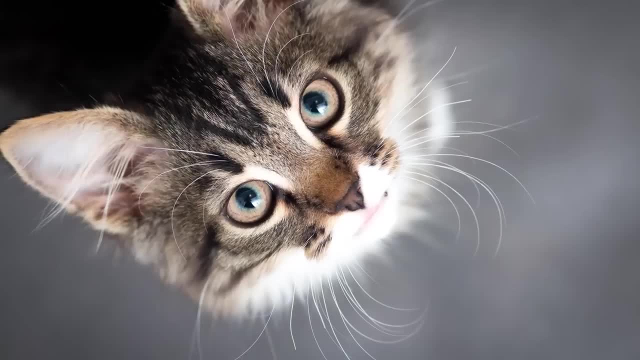 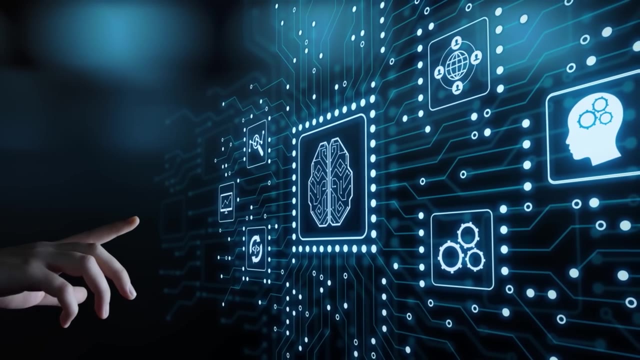 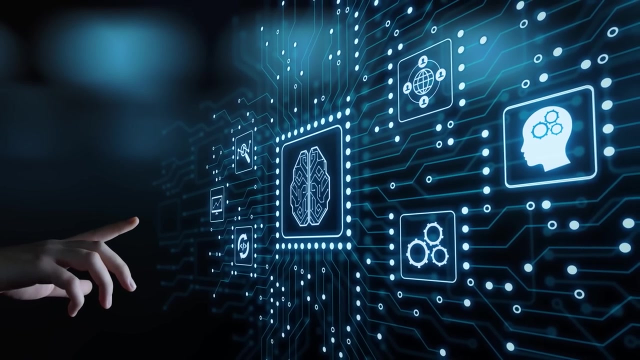 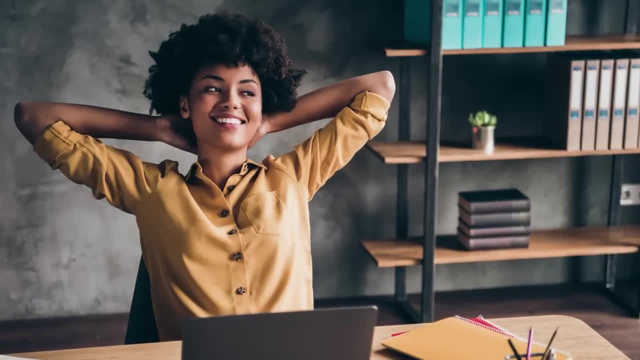 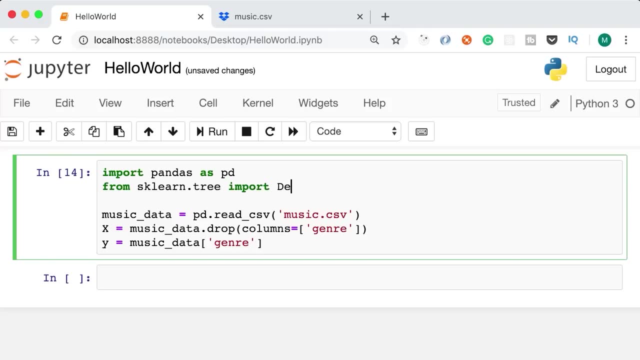 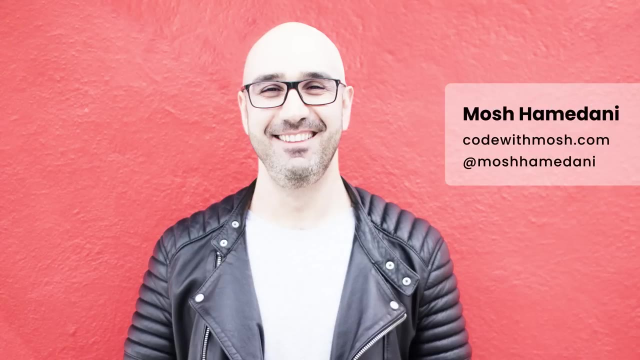 learn more intermediate to advanced level concepts. You don't need any prior knowledge in machine learning, but you need to know Python fairly well. If you don't, I've got a couple of tutorials for you here on my channel. The links are below this video. I'm Mosh Hamedani and I'm super excited to be your instructor On this channel. I have tons of programming tutorials that you might find helpful, So be sure to subscribe, as I upload new tutorials every week. Now let's jump in and get started. 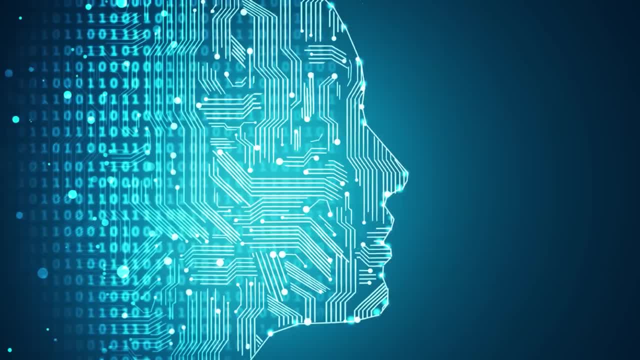 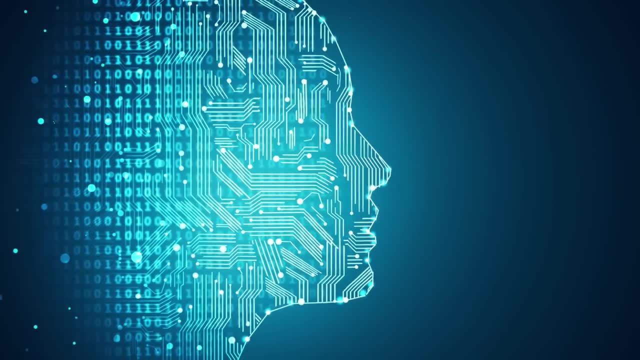 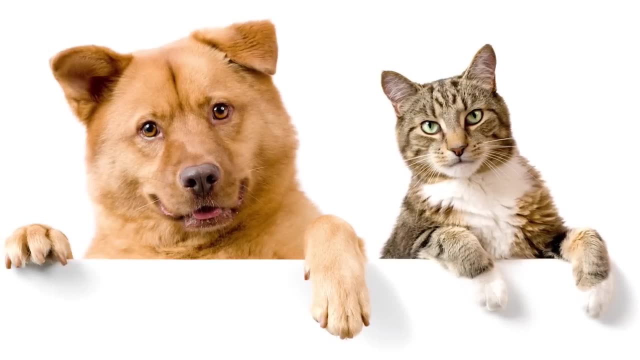 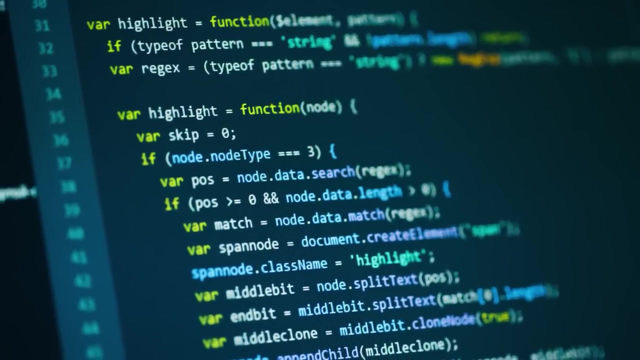 In this section you're going to learn about machine learning, which is a subset of AI or artificial intelligence. It's one of the trending topics in the world these days and it's going to have a lot of applications in the future. Here's an example. Imagine I ask you to write a program to scan an image and tell if it's a cat or a dog. If you want to build this program using traditional programming techniques, your program is going to get overly complex. You will have to come up with lots of rules to look for a specific program. 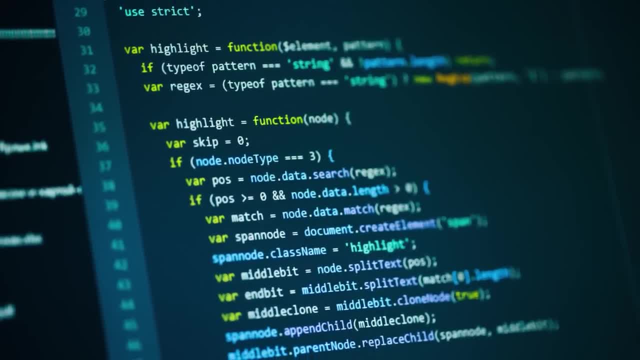 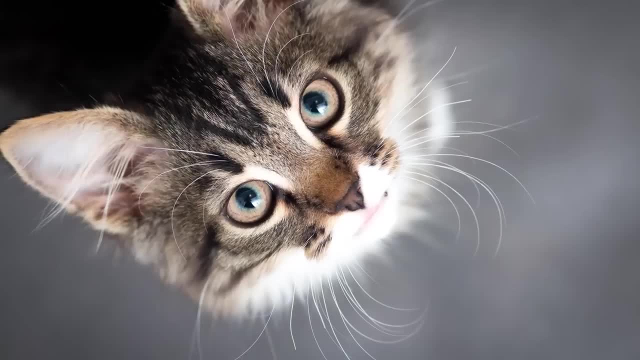 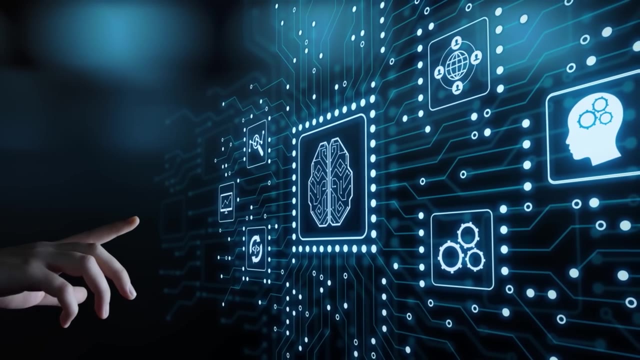 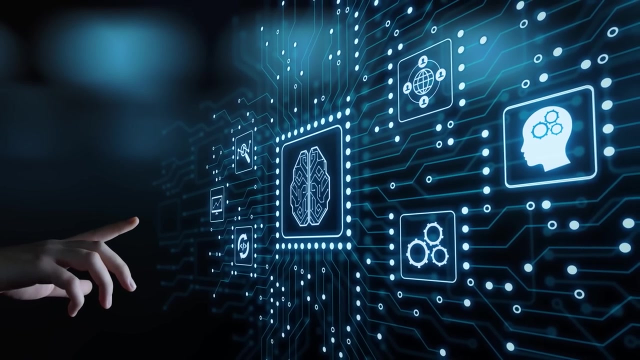 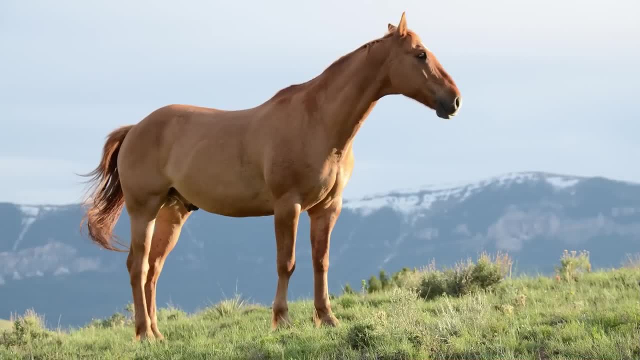 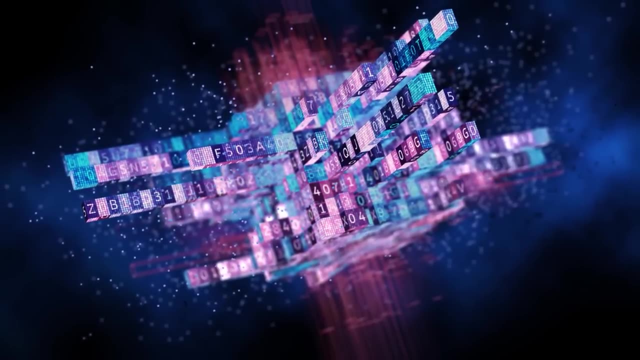 dogs and horses. Once again, you'll have to rewrite all those rules. That's not going to work. So machine learning is a technique to solve these kind of problems, and this is how it works. We build a model or an engine and give it lots and lots of data. For example, we give 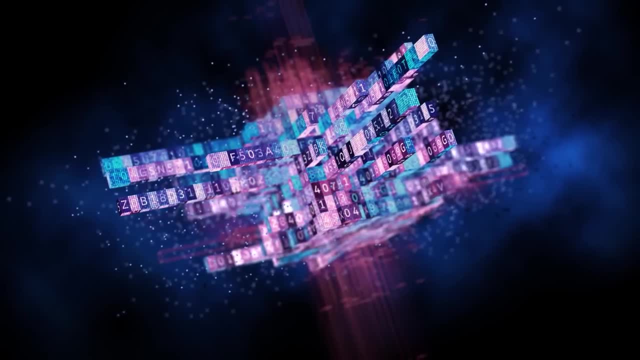 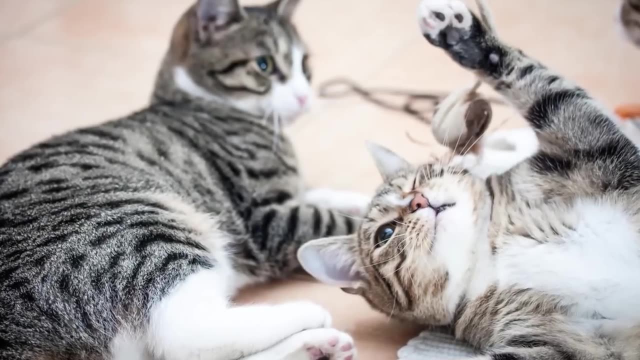 it thousands or tens of thousands of pictures of cats and dogs. Our model will then find and learn patterns in the input data so we can give it a new picture of a cat that it hasn't seen before and ask it: is it a cat or a dog or a horse? And it will tell us, with a certain level of 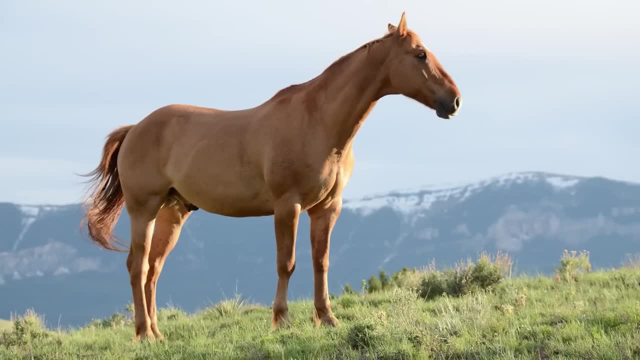 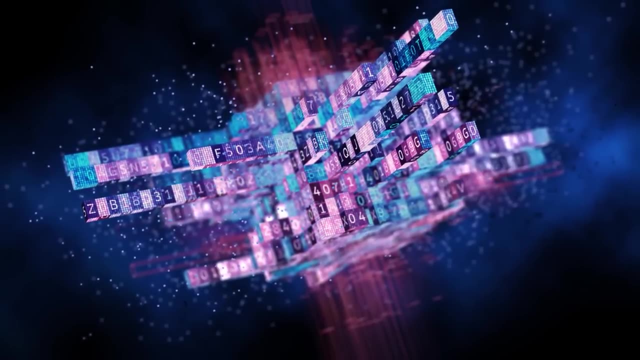 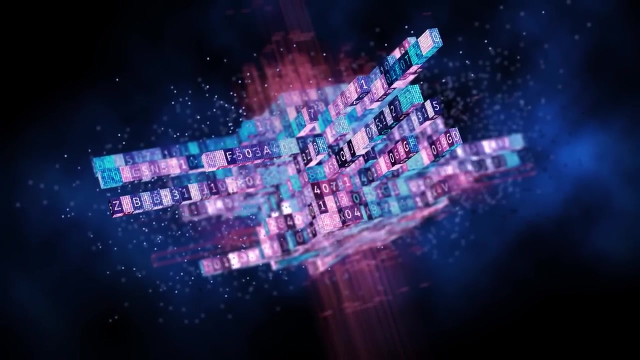 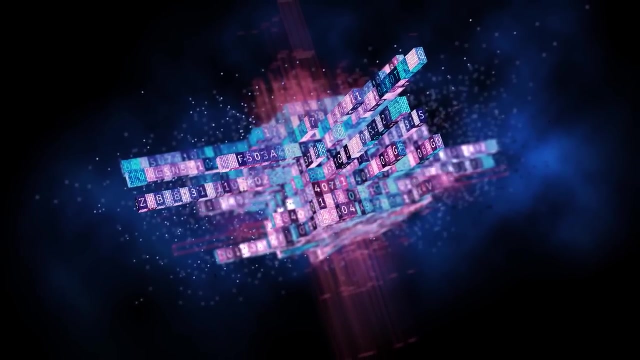 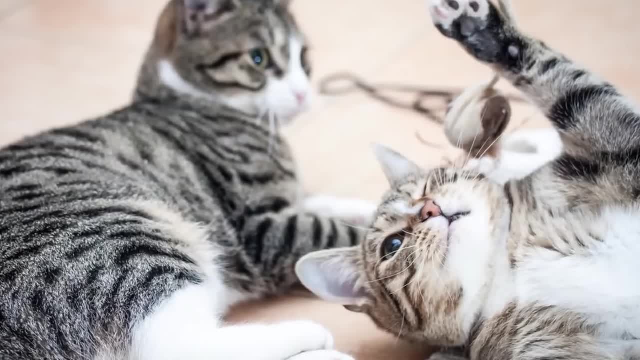 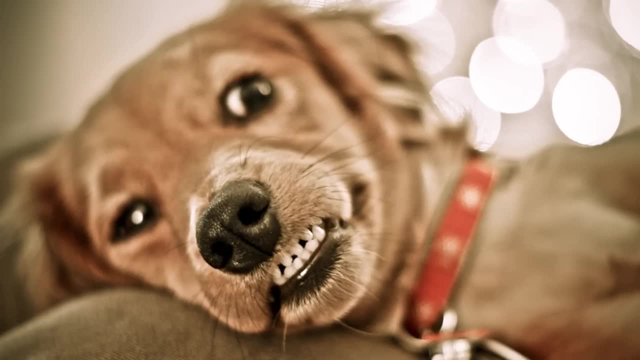 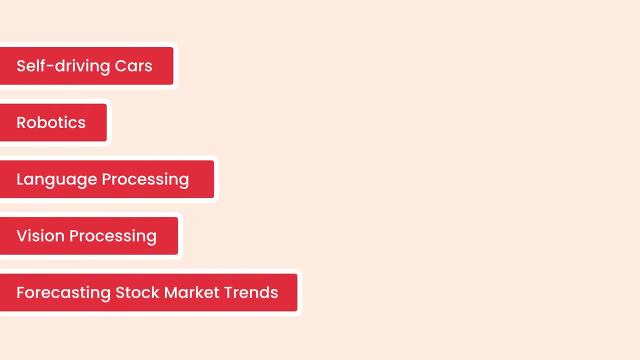 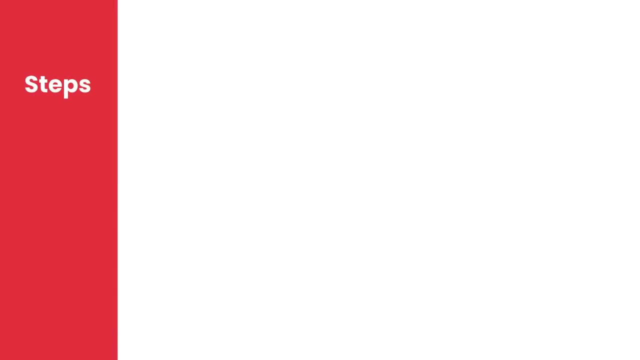 A machine learning project involves a number of steps. The first step is to import our data, which often comes in the form of a CSV file. You might have a database with lots of data. we can simply export that data and store it in a CSV file for the. 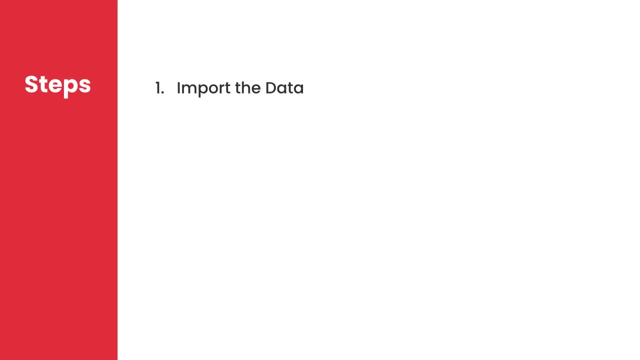 purpose of our machine learning project. So we import our data. next we need to clean it, And this involves tasks such as removing duplicated data. If you have duplicates in the data, we don't want to feed this to our model, because 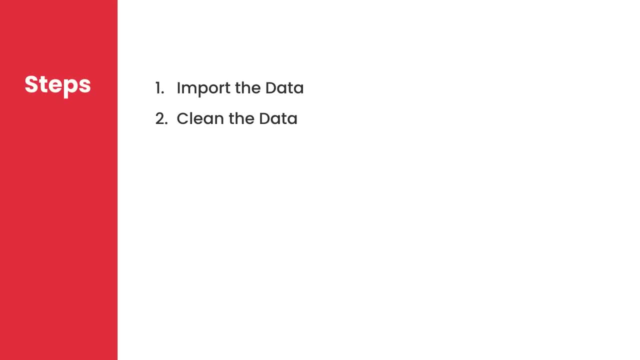 otherwise our model will learn bad patterns in the data and it will produce the wrong result. So we should make sure that our input data is in a good and clean shape. If there are data that is irrelevant, we should remove them. If they're duplicated. 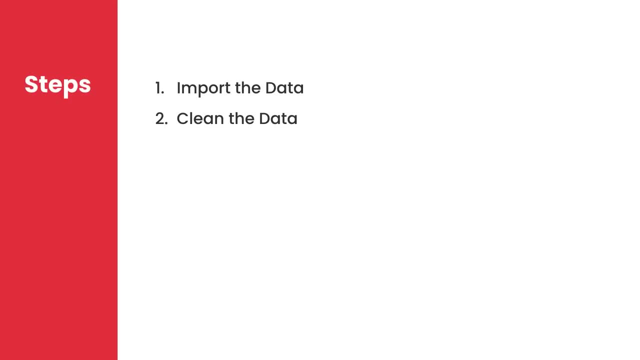 or incomplete, we can remove or modify them. If our data is text-based, like the name of countries or genres of music or cats and dogs, we need to convert them to numerical values. So this step really depends on the kind of data we are working with. 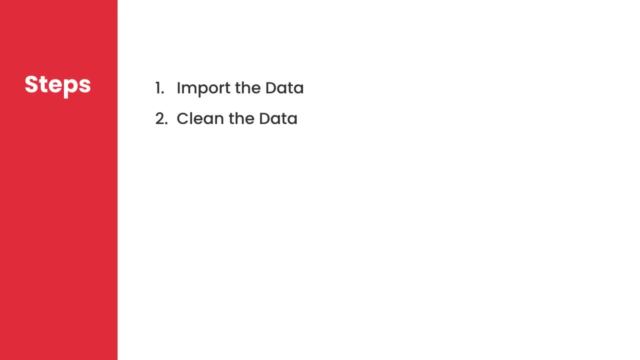 Every project is different. Now that we have a clean data set, we need to split it into two segments: One for training our model and the other for testing it to make sure that our model produces the right result. For example, if you have a thousand pictures of cats and dogs, 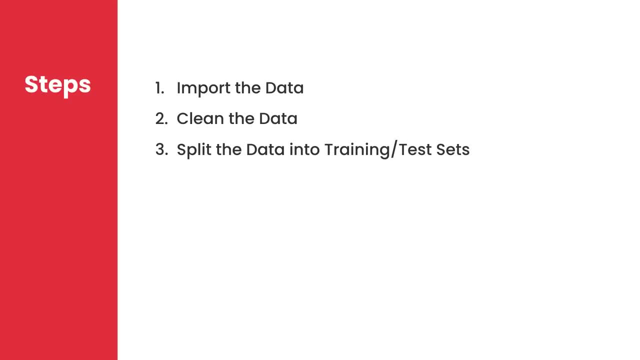 we can reserve 80% for training and the other 20% for testing. The next step is to create a model, and this involves selecting an algorithm to analyze the data. There are so many different machine learning algorithms out there, such as: 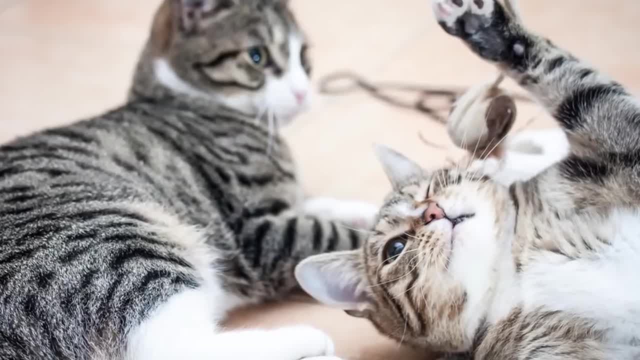 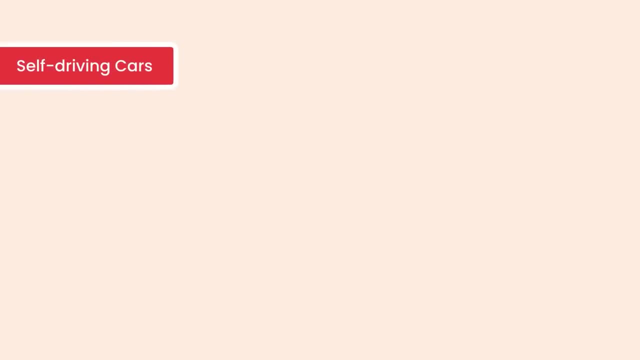 accuracy. The more input data we give it, the more accurate our model is going to be. So that was a very basic example, But machine learning has other applications: in self-driving cars, robotics, language processing, vision processing, forecasting, things like stock market trends and the weather games, and so on. 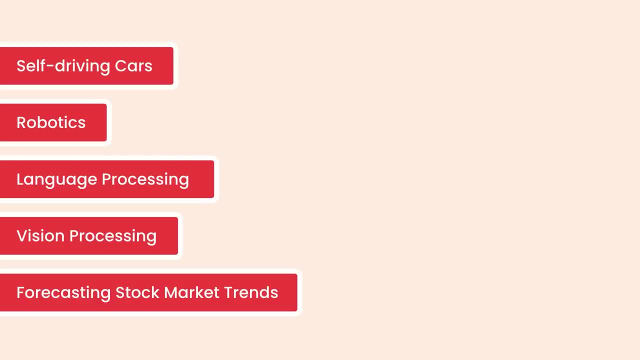 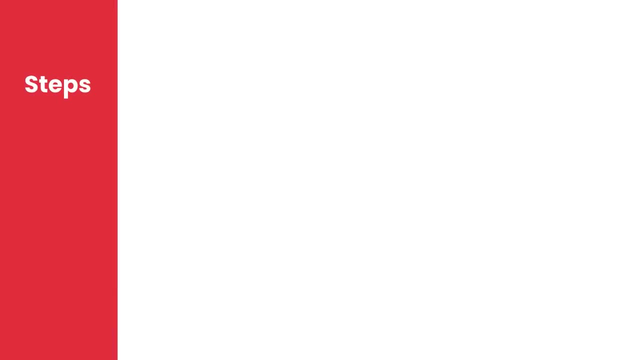 So that's the basic idea about machine learning. Next we'll look at machine learning in action. A machine learning project involves a number of steps. The first step is to import our data, which often comes in the form of a CSV file. You might have a database with lots of data. 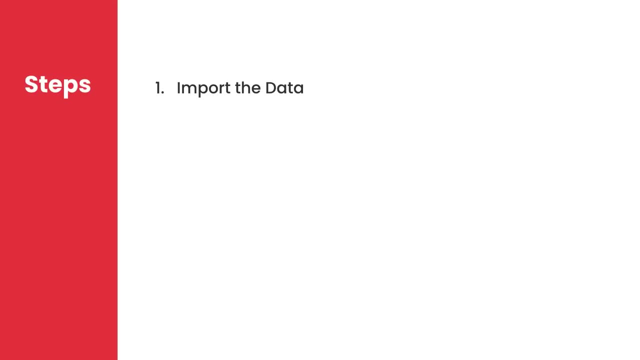 We can simply export that data and store it in a CSV file for the purpose of our machine learning project. So we import our data. next we need to clean it, And this involves tasks such as removing duplicated data. If you have duplicates in the data, we don't want to feed this to our model because otherwise, 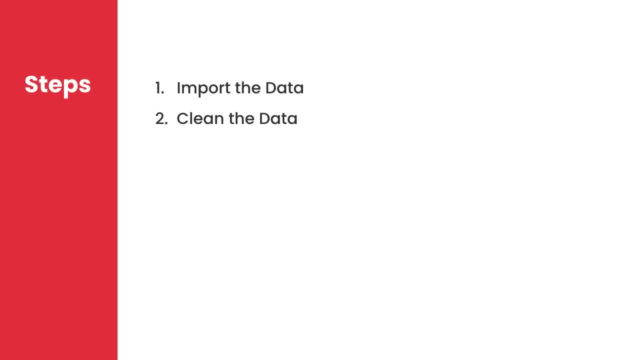 our model will learn bad patterns in the data and it will produce the wrong result. So we should make sure that our input data is in a good and clean shape. If there are data that is irrelevant, we should remove them. If they're duplicated. 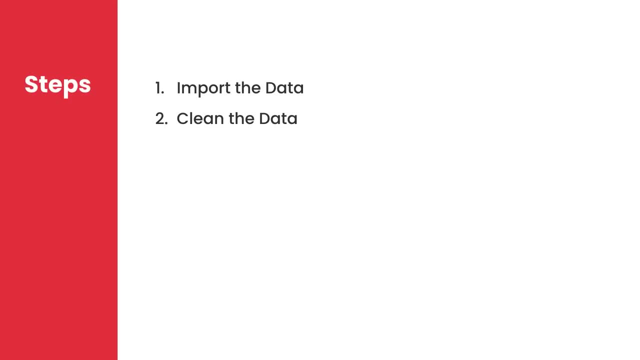 or incomplete, we can remove or modify them. If our data is text-based, like the name of countries or genres of music or cats and dogs, we need to convert them to numerical values. So this step really depends on the kind of data we are working with. Every 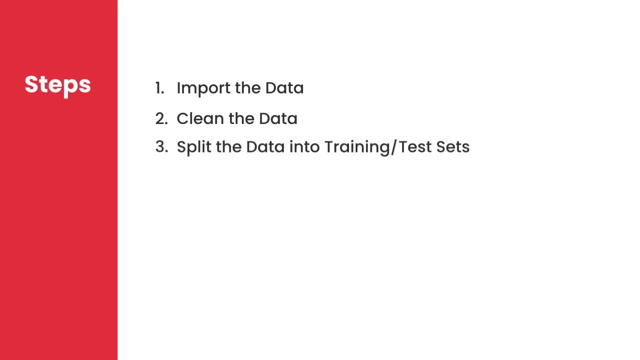 project is different. Now that we have a clean data set, we need to split it into two segments: One for training our model and the other for testing it to make sure that our model produces the right result. For example, if you have a thousand pictures, 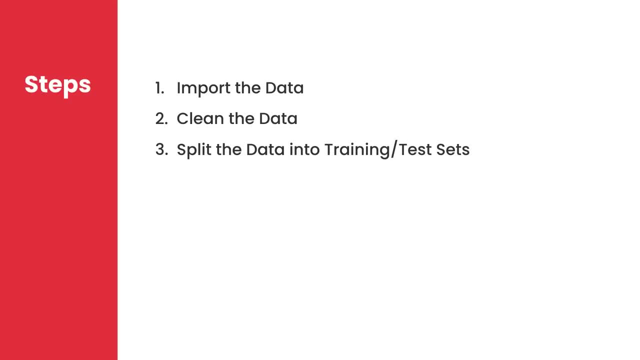 of cats and dogs. we can reserve 80% for training and the other 20% for testing. The next step is to create a model, And this involves selecting an algorithm to analyze the data. There are so many different machine learning algorithms out there, such as decision trees. 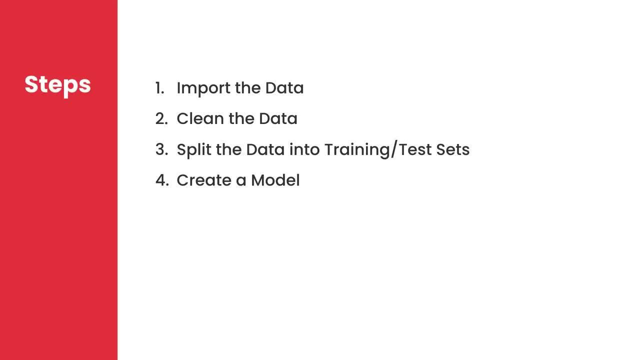 neural networks and so on. Each algorithm has pros and cons in terms of accuracy and performance, So the algorithm you choose depends on the kind of problem you're trying to solve and your input data. Now, the good news is that we don't have to explicitly 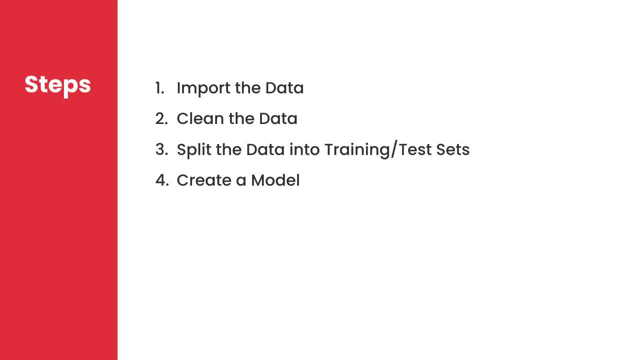 decision trees, neural networks and so on. Each algorithm has pros and cons in terms of accuracy and performance, So the algorithm you choose depends on the kind of problem you're trying to solve and your input data. Now, the good news is that we don't have to explicitly program an 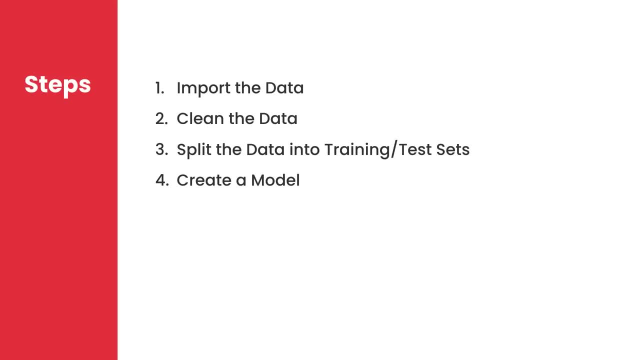 algorithm. There are libraries out there that provide these algorithms. One of the most popular ones, which we are going to look at in this tutorial, is scikit-learn. So we build a model using an algorithm. Next we need to. 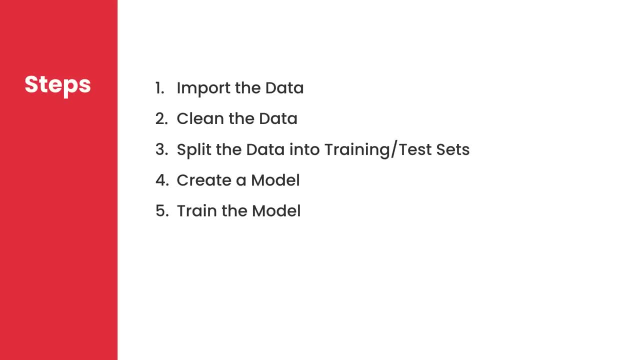 train our model, So we feed our training data. Our model will then look for the patterns in the data. So next we can ask it to make predictions. Back to our example of cats and dogs. we can ask our model: is this a cat or a dog? 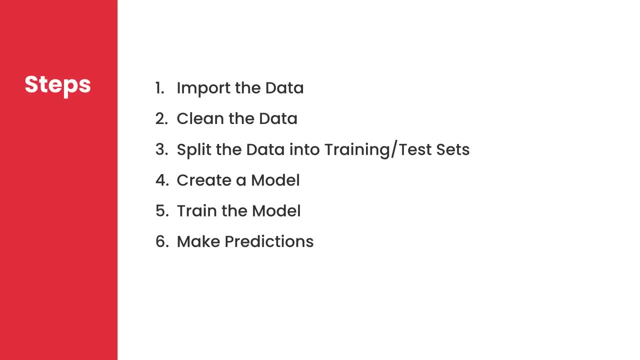 And our model will make a prediction. Now, the prediction is not always accurate. In fact, when you start out, it's very likely that your predictions are inaccurate. So we need to evaluate the predictions and measure their accuracy. Then we need to get back to our model and either select: 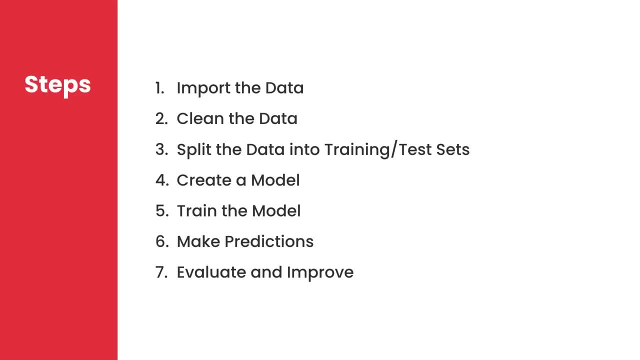 a different algorithm that is going to produce a more accurate result for the kind of problem we're trying to solve, or fine-tune the parameters of our model. So each algorithm has parameters that we can modify to optimize the accuracy. So these are the high-level steps that you follow in a machine learning project. 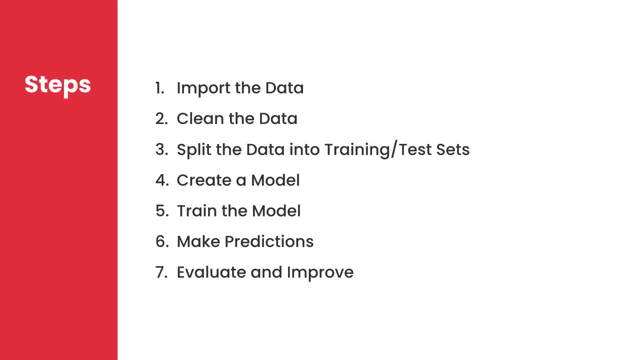 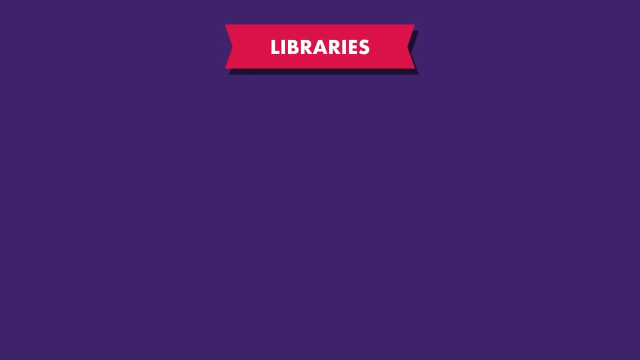 Next we'll look at the libraries and tools for machine learning. In this lecture we're going to look at the popular Python libraries that we use in machine learning projects. The first one is NumPy, which provides a multi-dimensional array- Very, very popular library. The second one is Pandas, which is a data 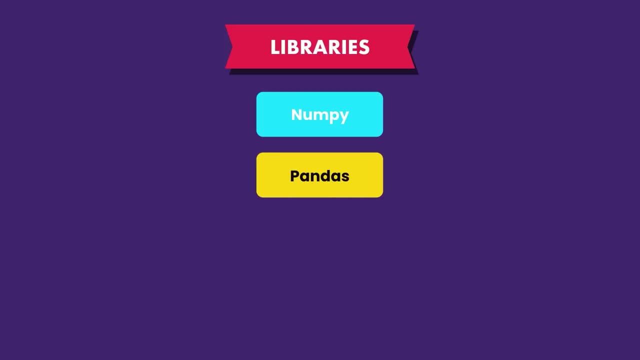 analysis library that provides a concept called DataFrame. A DataFrame is a two-dimensional data structure similar to an Excel spreadsheet, So we have rows and columns. we can select data in a row or a column, or a range of rows and columns- Again very, very popular in machine learning and data science projects. 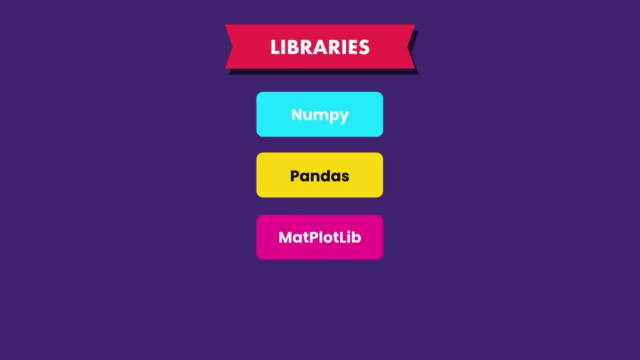 The third library is Matplotlib, which is a two-dimensional plotting library for creating graphs and plots. The next library is Scikit-learn, which is one of the most popular machine learning libraries that provides all these common algorithms like decision trees, neural. 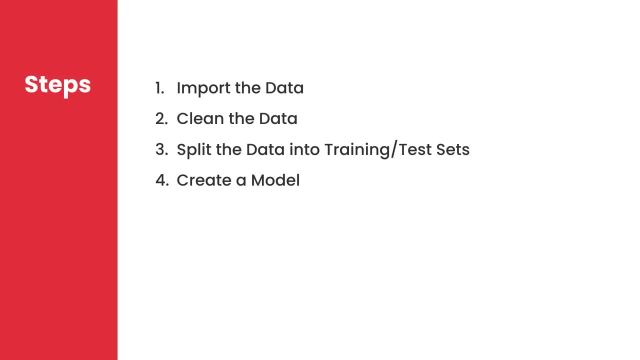 program an algorithm. There are libraries out there that provide these algorithms. One of the most popular ones, which we are going to look at in this tutorial, is scikit-learn. So we build a model using an algorithm. Next, we need to train our model, So we fitted our training data. 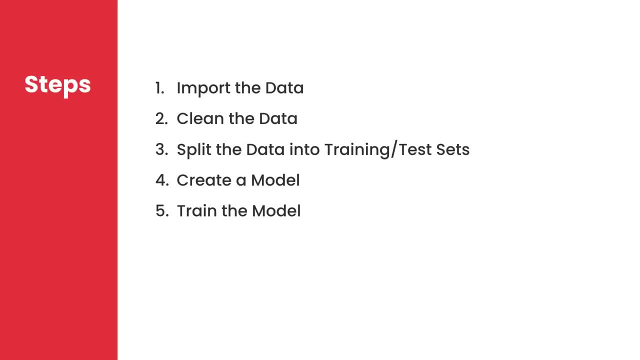 Our model will then look for the patterns in the data. So next we can ask it to make predictions. Back to our example of cats and dogs. we can ask our model: is this a cat or a dog? And our model will make a prediction. Now the prediction. 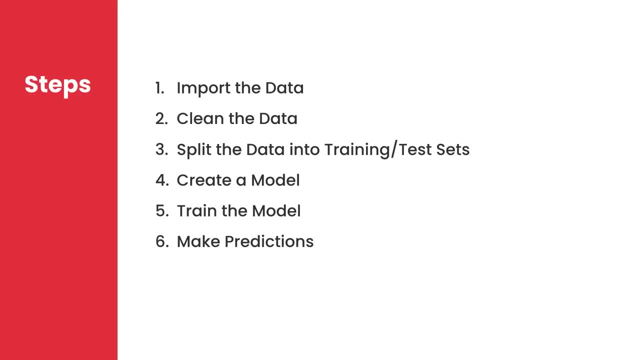 is not always accurate. In fact, when you start out, it's very likely that your predictions are inaccurate. So we need to evaluate the predictions and measure their accuracy. Then we need to get back to our model and either select a different algorithm that is going to produce a more accurate 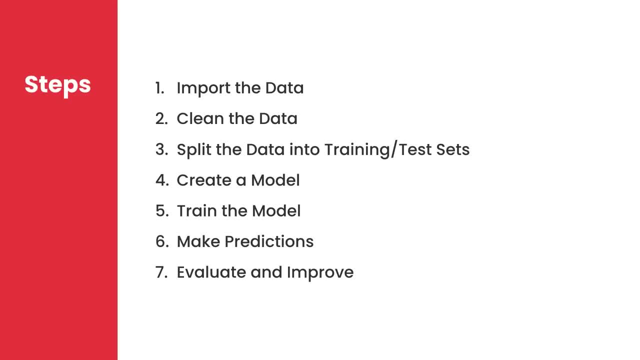 result for the kind of problem we're trying to solve, or we need to create a model that is going to produce a more accurate result for the kind of problem we're trying to solve, or we need to create a model that is going to produce a more accurate result for the kind of problem we're trying to solve, or fine-tune. 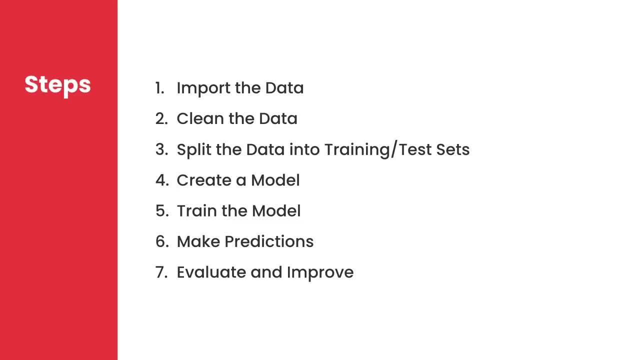 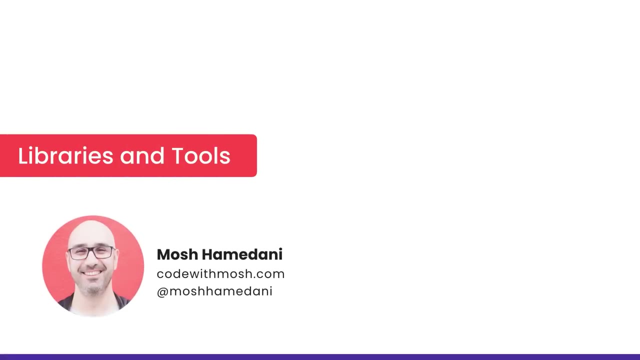 the parameters of our model. So each algorithm has parameters that we can modify to optimize the accuracy. So these are the high-level steps that you follow in a machine learning project. Next we'll look at the libraries and tools for machine learning. In this lecture we're going to look at the popular 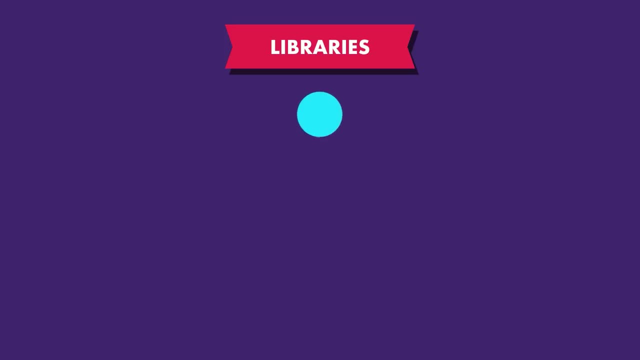 Python libraries that we use in machine learning projects. The first one is NumPy, which provides a multi-dimensional array- Very, very popular library. The second one is Pandas, which is a data analysis library that provides a concept called DataFrame. A DataFrame is a two-dimensional data structure, similar 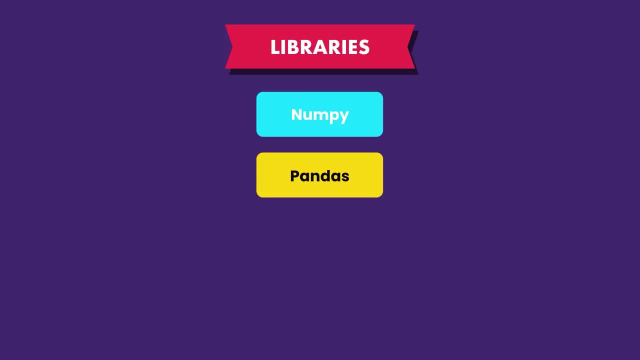 to an Excel spreadsheet. So we have rows and columns. We can select data in a row or a column or a range of rows and columns- Again very, very popular in machine learning and data science projects. The third library is MatPlotLib, which is a two-dimensional 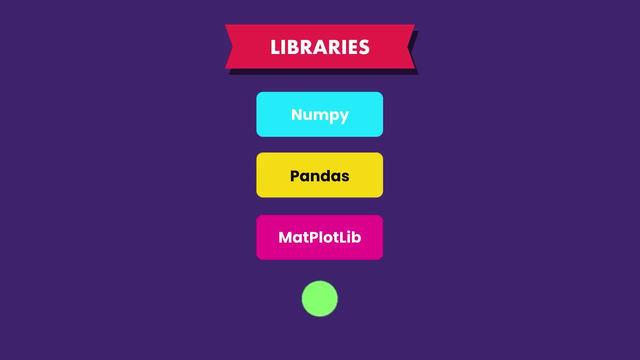 plotting library for creating graphs and plots. The next library is Scikit-learn, which is one of the most popular machine learning libraries that provides all these common algorithms like decision trees, neural networks and so on. Now, when working with machine learning projects, 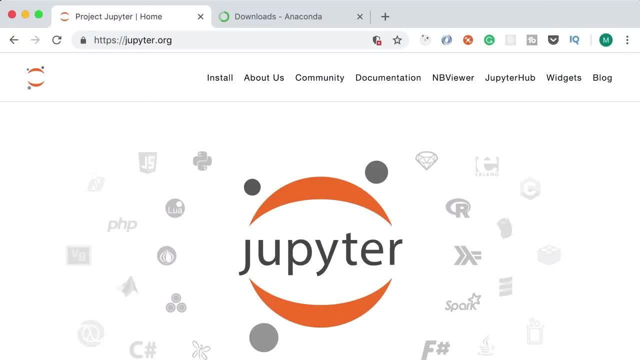 networks and so on. Now, when working with machine learning projects, we use an environment called Jupyter for writing our code. Technically, we can still use VS code or any other code editors, but these editors are not ideal for machine learning. 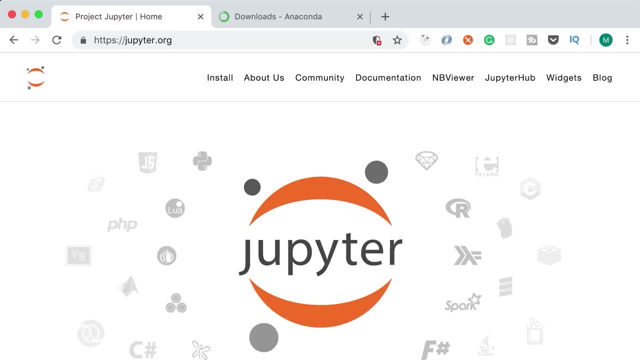 projects because we frequently need to inspect the data and that is really hard in environment-based projects. So we're going to look at the two-dimensional vscode and terminal If you're working with a table of 10 or 20 columns. 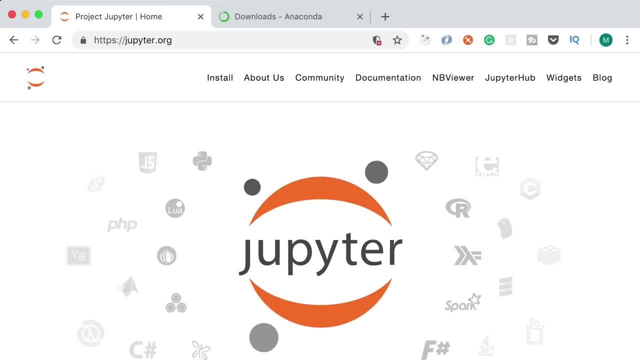 visualizing this data in a terminal window is really really difficult and messy, So that's why we use Jupyter. It makes it really easy to inspect our data. Now, to install Jupyter, we are going to use a platform called Anaconda, So head over to anacondacom. 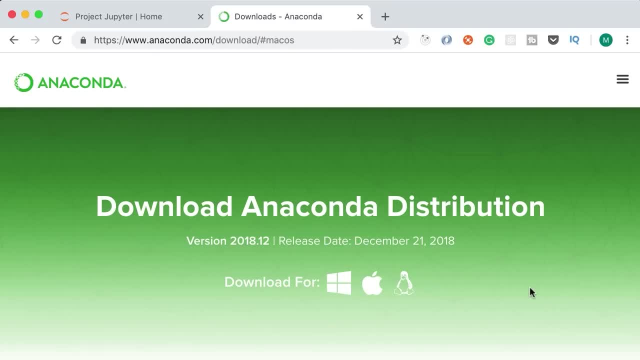 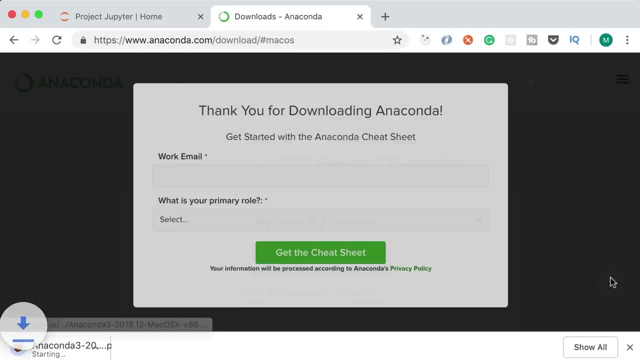 slash download. On this page you can download anaconda distribution for your operating system. So we have distributions for windows, mac and linux. So let's go ahead and install anaconda for python 3.7.. Download Alright. so here's anaconda downloaded on my machine. 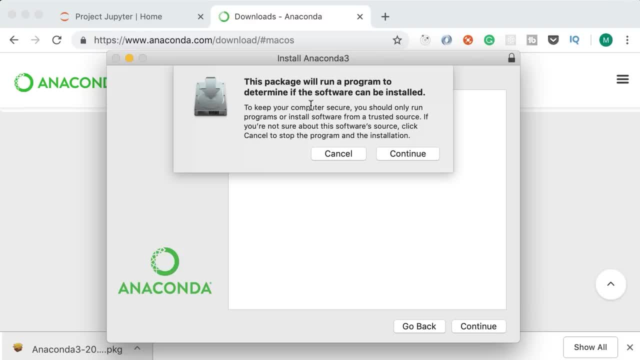 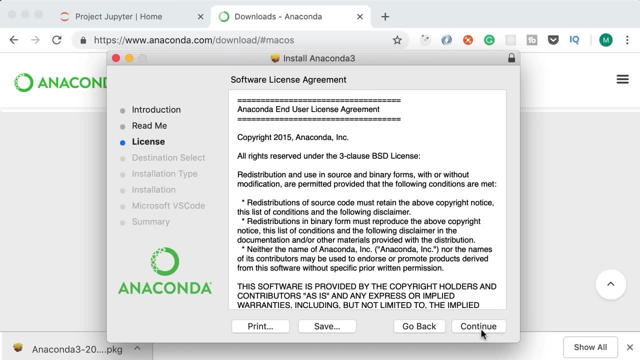 Let's double click this, Alright. first it's going to run a program to determine if the software can be installed. So let's continue and once again continue, continue, pretty easy, continue one more time. I agree with the language. 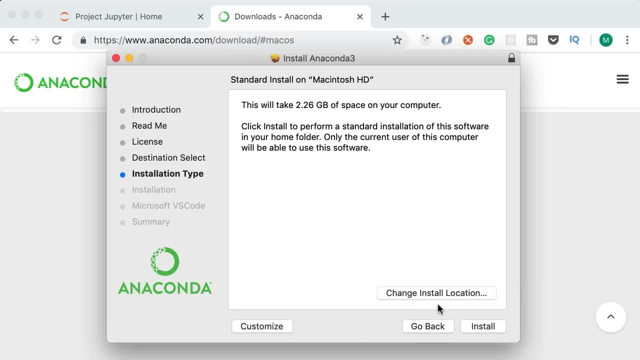 License agreement. okay, You can use the default installation location, so don't worry about that. Just click install. Give it a few seconds Now. the beautiful thing about anaconda is that it will install Jupyter, as well as all those popular data science libraries. 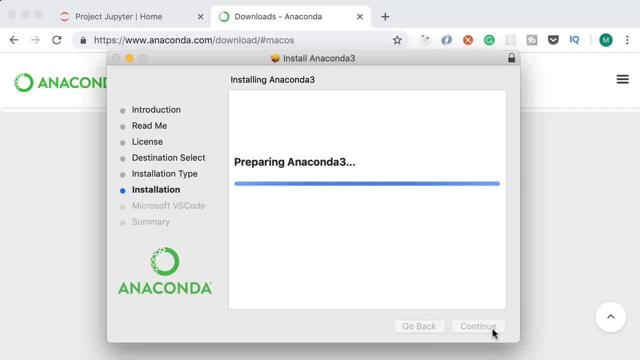 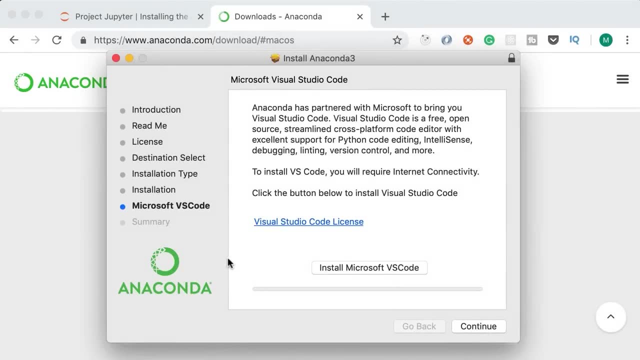 like NumPy, pandas and so on, So we don't have to manually install this using pip. Alright, now, as part of the next step, anaconda is suggesting to install Microsoft vs code. We already have this on our machine, so we don't have to install it. we can go with continue. 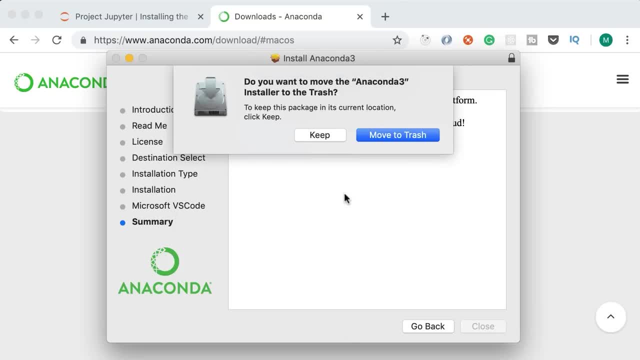 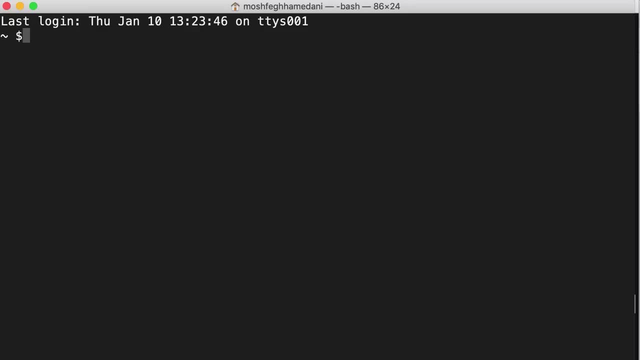 and close the installation Now. finally, we can move this to trash, because we don't need this installer in the future. Alright, now open up a terminal window and type Jupyter with a y space notebook. This will start the notebook server on your machine, So enter. 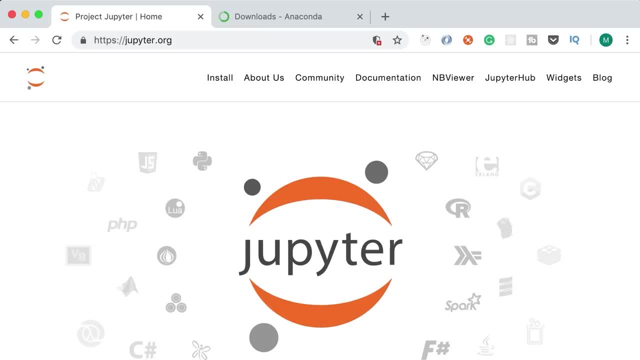 we use an environment called Jupyter for writing our code. Technically, we can still use VS Code or any other code editors, but these editors are not ideal for machine learning projects because we frequently need to inspect the data and that is really hard in environments like 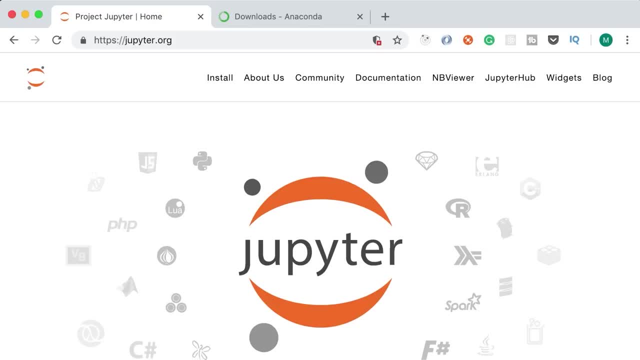 VS Code and Terminal. If you're working with a table of 10 or 20 columns, visualizing this data in a Terminal window is really really difficult and messy. So that's why we use Jupyter. It makes it really easy to inspect our 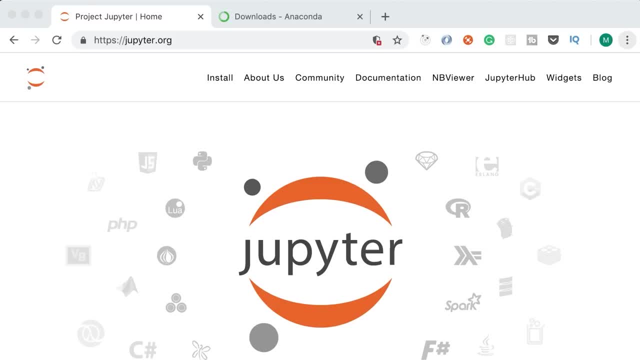 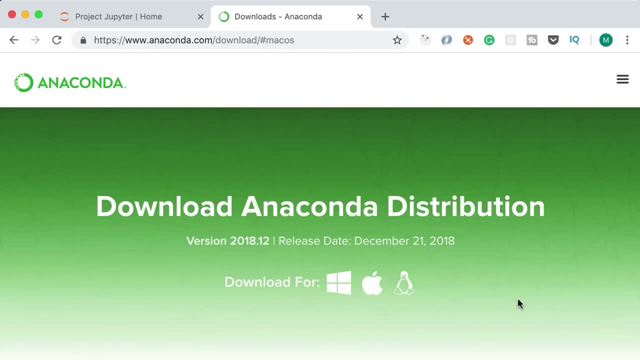 data. Now to install Jupyter, we're going to use a platform called Anaconda, So head over to anacondacom slash download. On this page you can download Anaconda distribution for your operating system. So we have distributions for Windows. 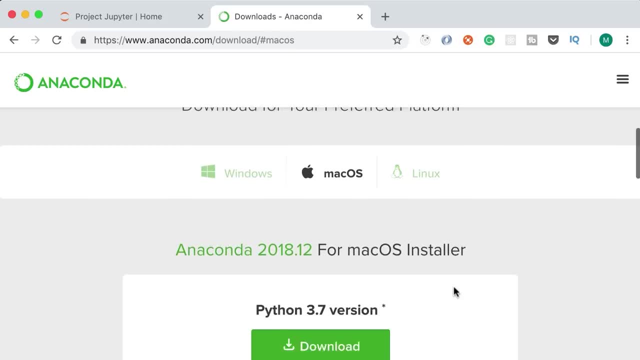 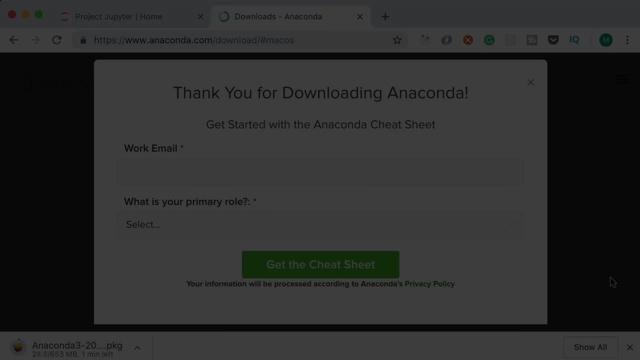 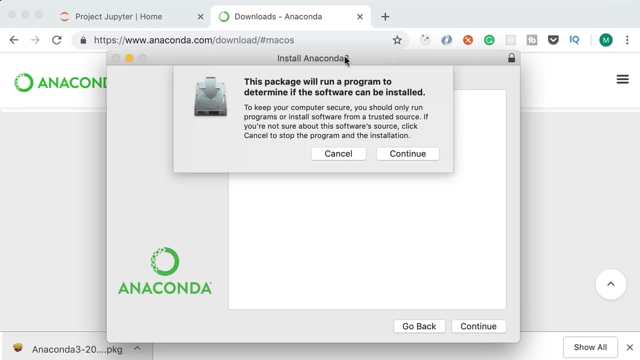 Mac and Linux. So let's go ahead and install Anaconda for Python 3.7.. Download Alright. so here's Anaconda downloaded on my machine. Let's double click this, Alright. first it's going to run a program to determine if 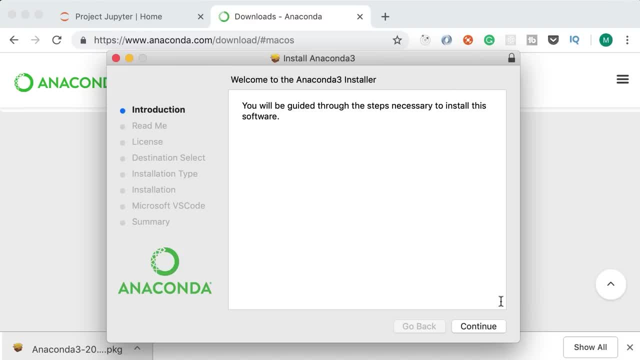 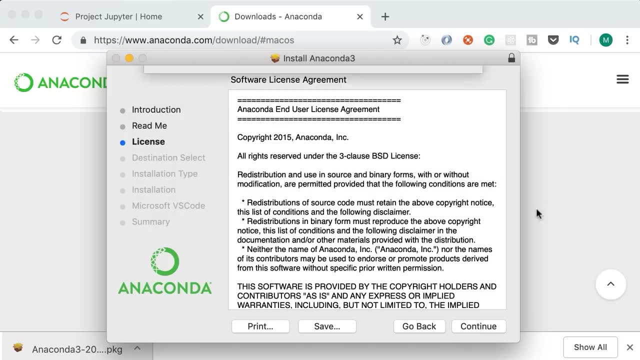 the software can be installed. So let's continue and once again, continue, continue. Pretty easy, Continue one more time. I agree with the license agreement. Okay, You can use the default installation location, so don't worry about that, Just click. 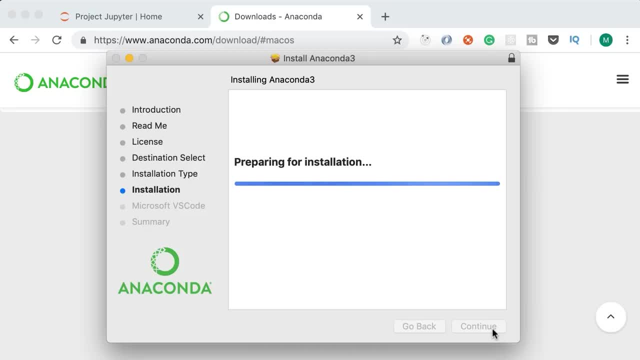 install. Give it a few seconds Now. the beautiful thing about Anaconda is that it will install Jupyter, as well as all those popular data science libraries like NumPy Pandas and so on, So we don't have to. 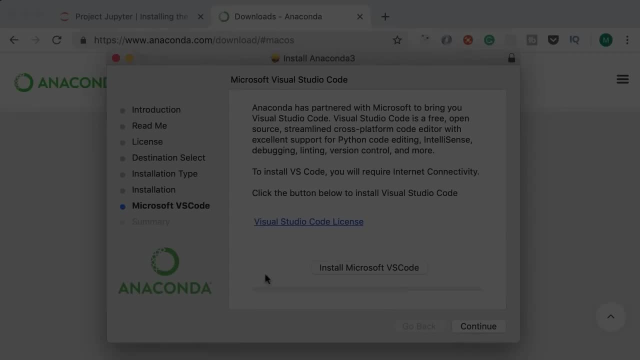 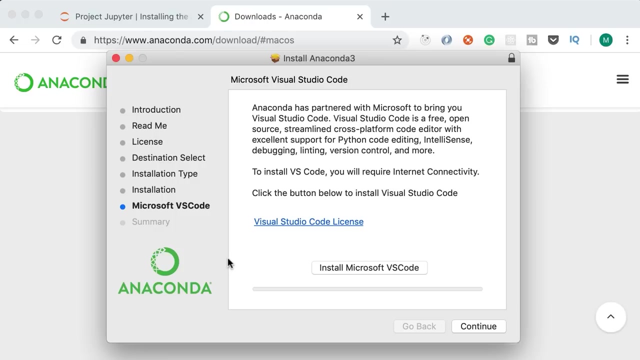 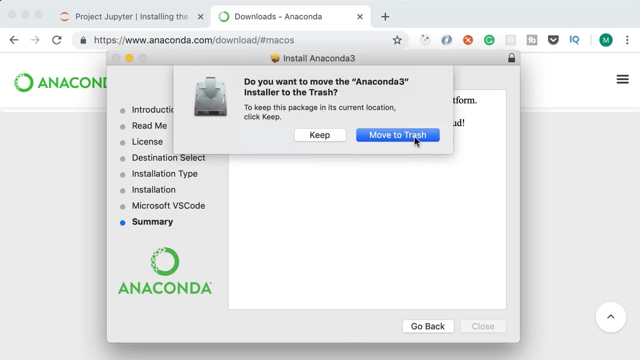 manually install this using pip. Alright. now, as part of the next step, Anaconda is suggesting to install Microsoft VS Code. We already have this on our machine, so we don't have to install it. We can go with, continue And close the installation. Now, finally, we can move this to trash. 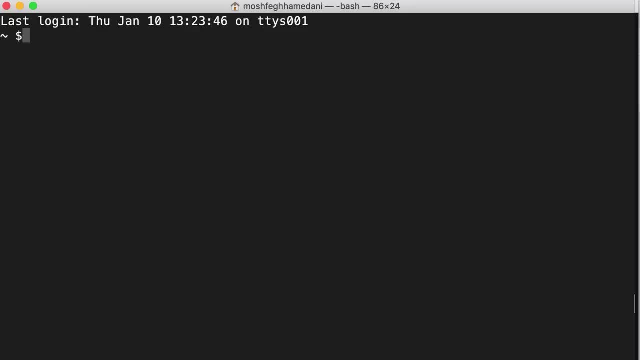 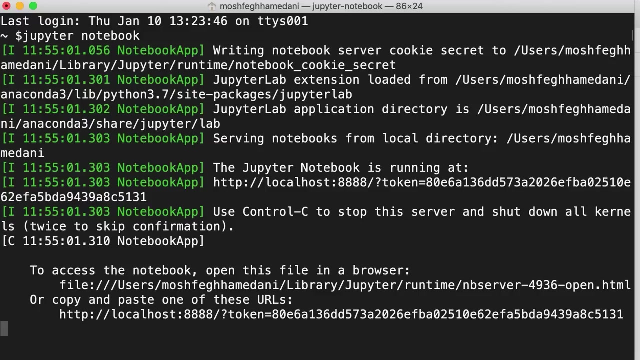 because we don't need this installer in the future. Alright, now open up a terminal window and type Jupyter with a y space notebook. This will start the notebook server on your machine. So enter, There you go. This will start the notebook server on your machine. 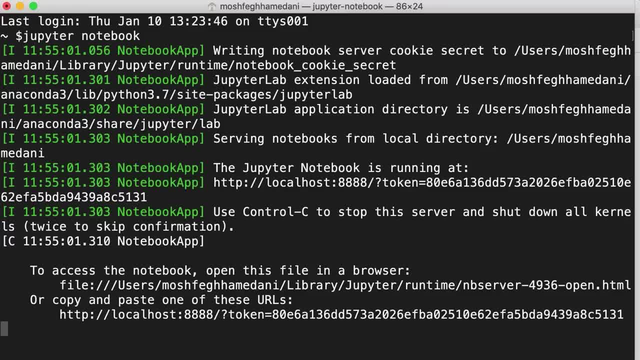 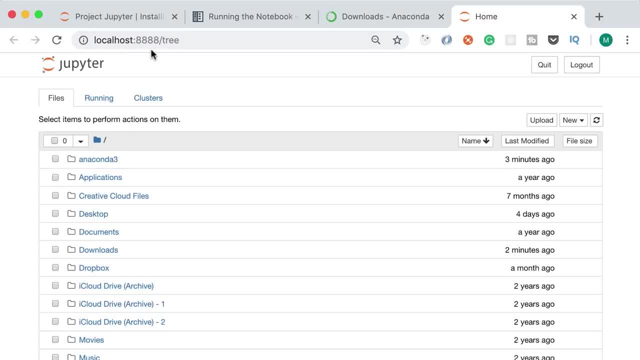 You can see these default messages here. Don't worry about them. Now it automatically opens a browser window Pointing to local host port 8888.. This is what we call Jupyter dashboard. On this dashboard we have a few tabs. 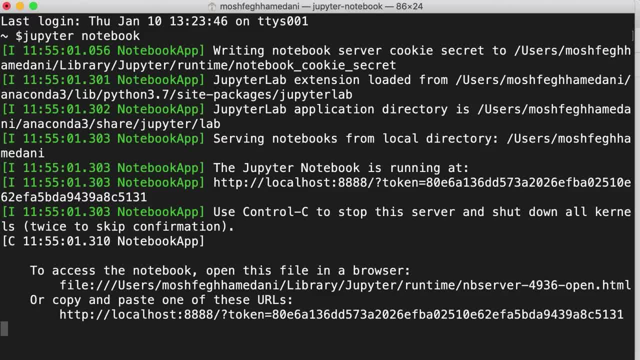 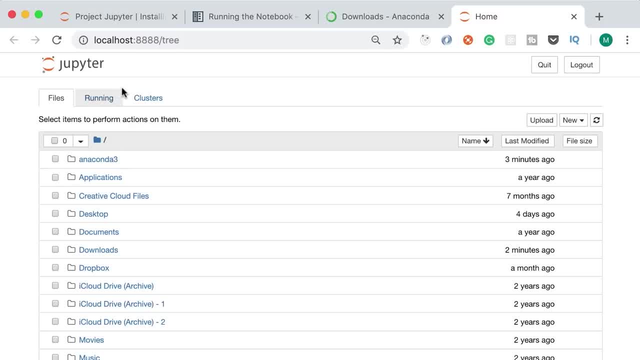 there you go. This will start the notebook server on your machine. you can see these default messages here. don't worry about them. Now it automatically opens a browser window pointing to local host port 8888. This is what we call Jupyter dashboard. On this dashboard we have a few tabs. the first tab: 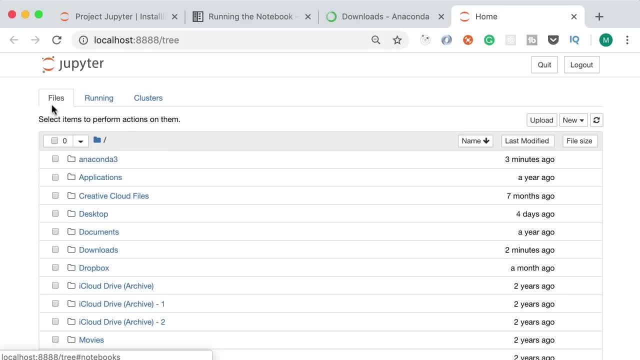 is the files tab and by default this points to your home directory. So every user on your machine has a home directory. this is my home directory on mac. you can see here we have a desktop folder as well as documents, downloads and so on On your machine. you're going to see different folders, So somewhere on your machine 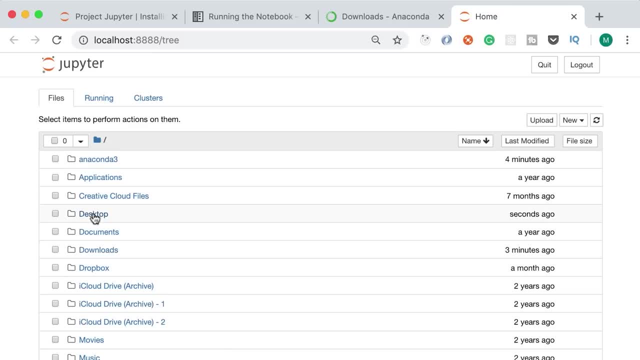 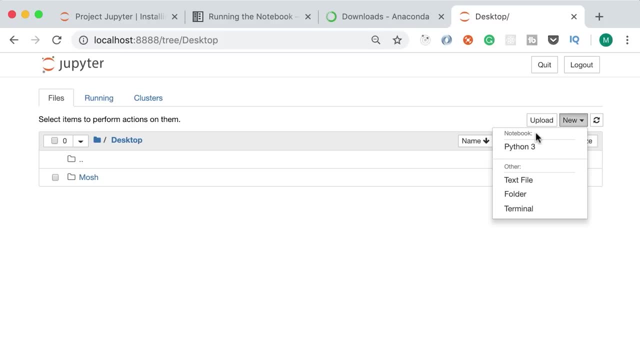 you need to create a Jupyter notebook. I'm going to go to desktop- here's my desktop, I don't have anything here- and then click new. I want to create a notebook for python 3.. In this notebook, we can write python code and execute it line by line. 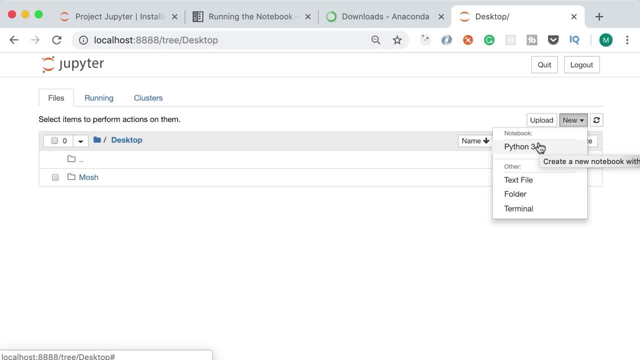 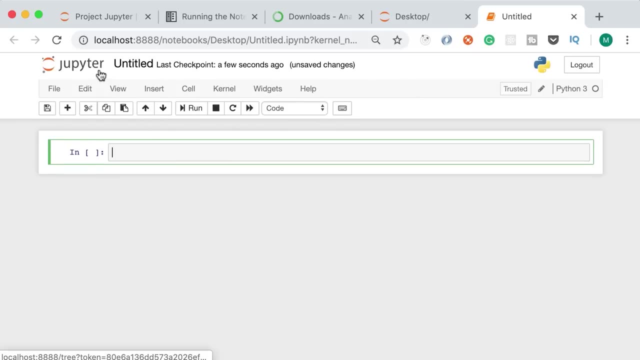 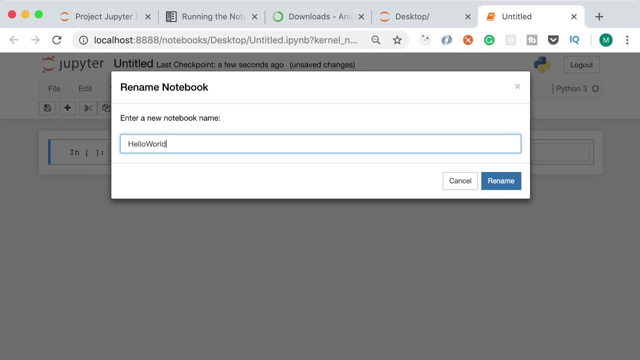 We can easily visualize our data, as you will see over the next few videos, So let's go ahead with this. alright, here's our first notebook You can see. by default, it's called untitled. let's change that to hello world. so this is going to be the hello world of our machine learning. 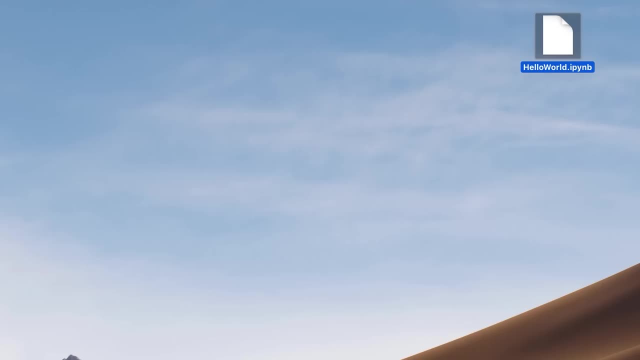 project. Let's rename this now. if you look at your desktop, you can see this file: hello worldipynb. this is a Jupyter notebook. It's kind of similar to our py files, where we write our python code, but it includes additional. 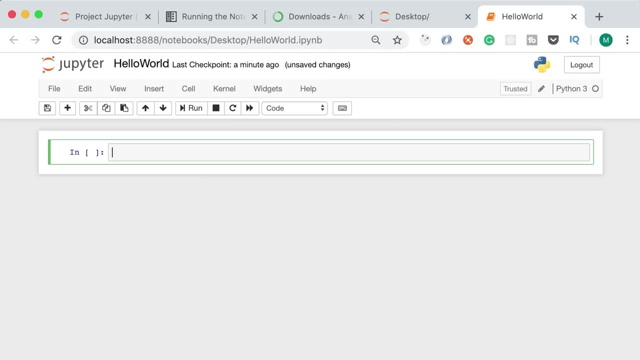 data that Jupyter uses to execute our code. So back to our notebook, let's do a print hello world and then click this run button here and here's the result printed in Jupyter. So we don't have to navigate back and forth between the terminal window. 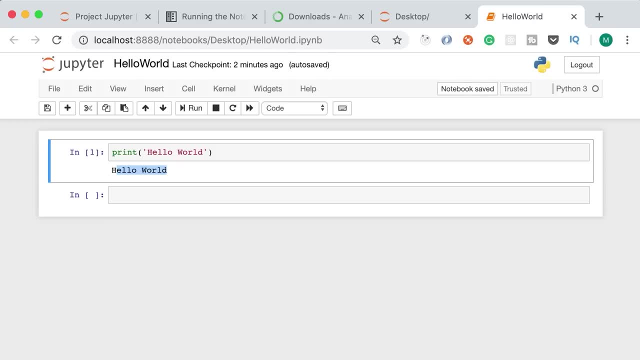 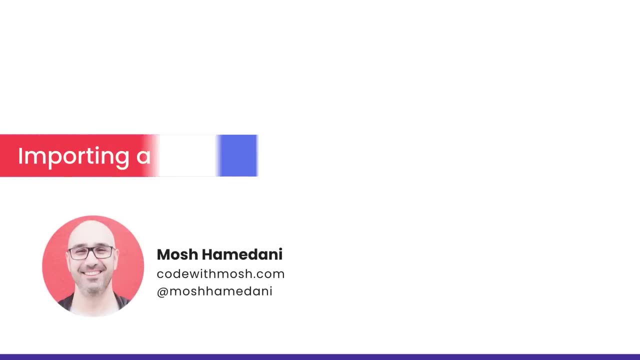 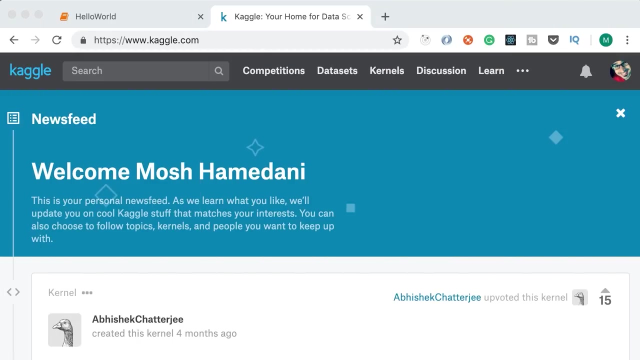 we can see all the results right here. Next, I'm going to show you how to load a data set from a csv file in Jupyter Music playing. Alright, in this lecture we're going to download a data set from a very popular website called Kagglecom- Kaggle. 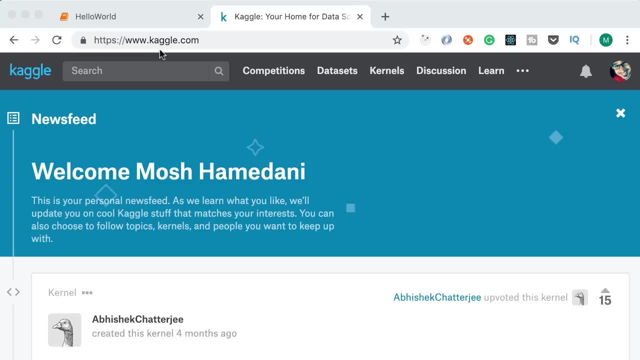 is basically a place to do data science projects, So the first thing you need to do is to create an account. you can sign up with Facebook, Google or using a custom email and password. Once you sign up, then come back here on Kagglecom. 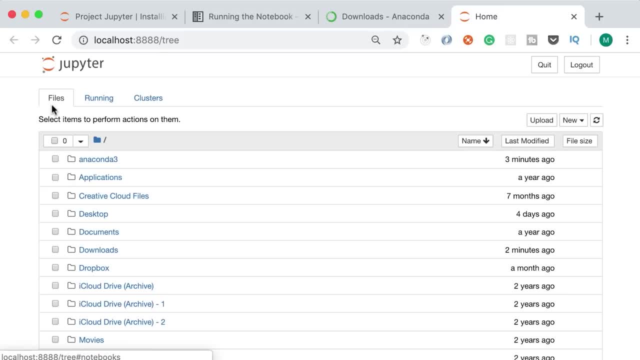 The first tab is the files tab and by default this points to your home directory. So every user on your machine has a home directory. This is my home directory on Mac. You can see here we have a desktop folder as well as. 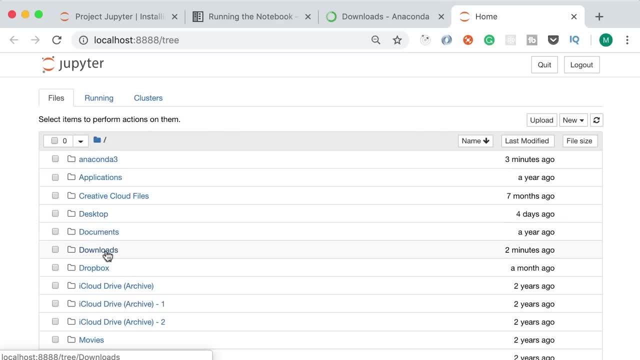 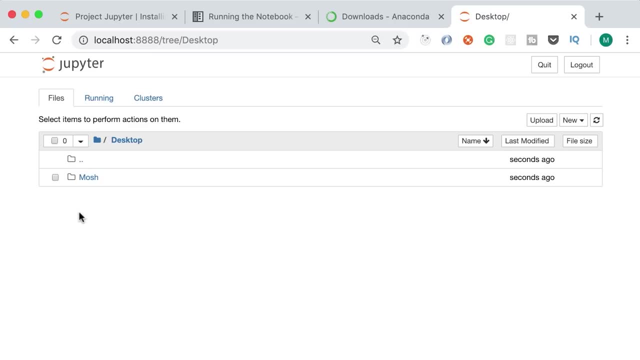 documents, downloads and so on. On your machine you're going to see different folders. So somewhere on your machine you need to create a Jupyter notebook. I'm going to go to desktop- Here's my desktop- I don't have anything here- And then click. 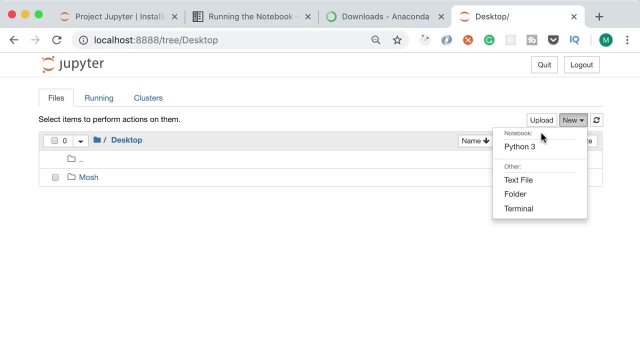 new. I want to create a notebook for Python 3.. In this notebook, we can write Python code and execute it line by line. We can easily visualize our data, as you will see over the next few videos. So let's go ahead with this. Alright, here's. 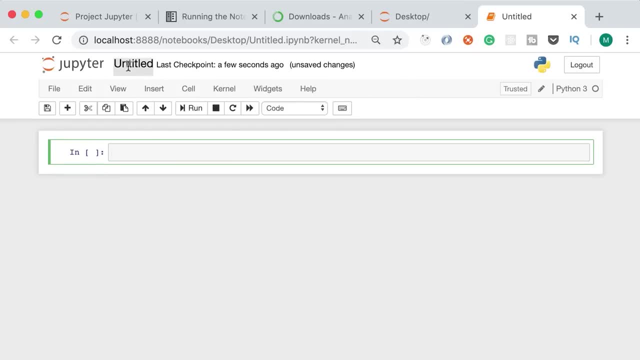 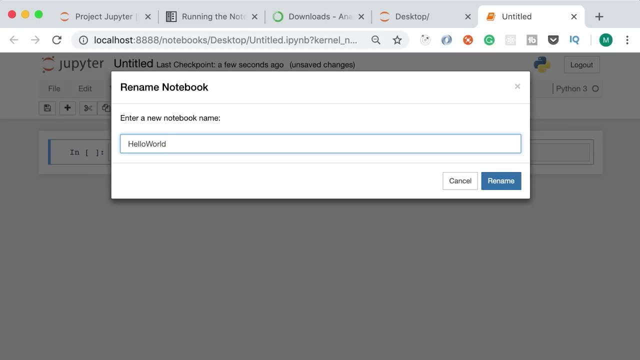 our first notebook. You can see by default it's called untitled. Let's change that to hello world. So this is going to be the hello world of our machine learning project. Let's rename this Now. if you look at your 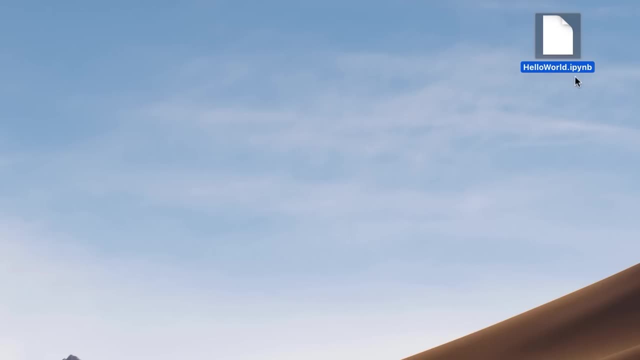 desktop you can see this file. hello worldipynb. This is a Jupyter notebook. It's kind of similar to our py files, where we write our Python code, but it includes additional data that Jupyter uses to execute our code. So back to our 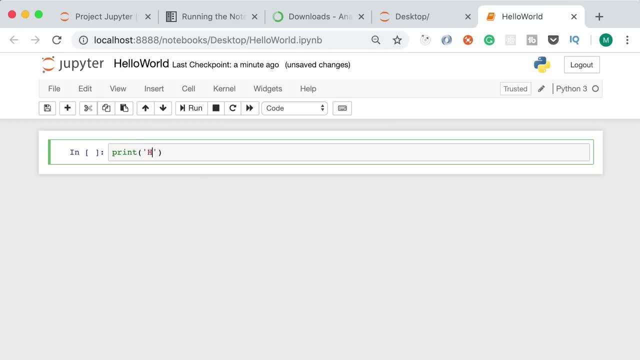 notebook. let's do a print hello world And then click this run button here. and here's the result printed in Jupyter. So we don't have to navigate back and forth between the terminal window. We can see all the results right here. 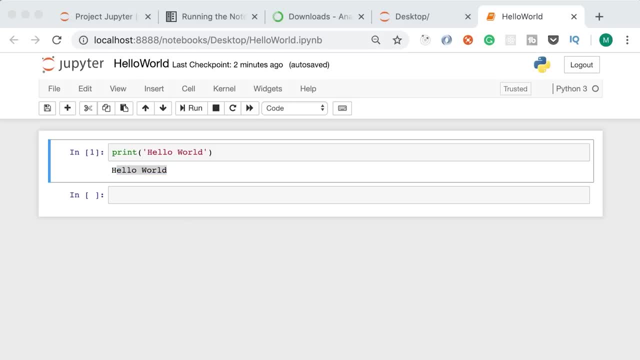 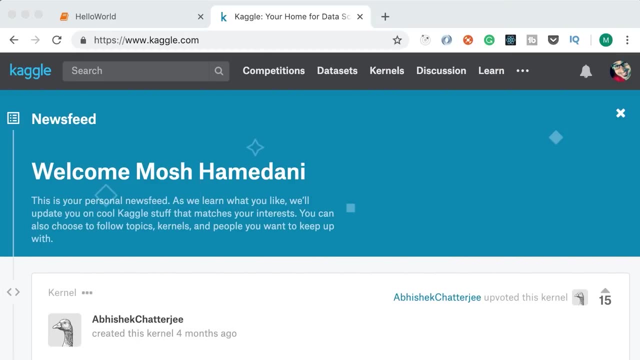 Next, I'm going to show you how to load a data set from a CSV file in Jupyter. Alright, in this lecture, we're going to download a data set from a very popular website called Kagglecom. Kaggle is basically a place to do data science projects, So the first thing you need to do is to create a data set. 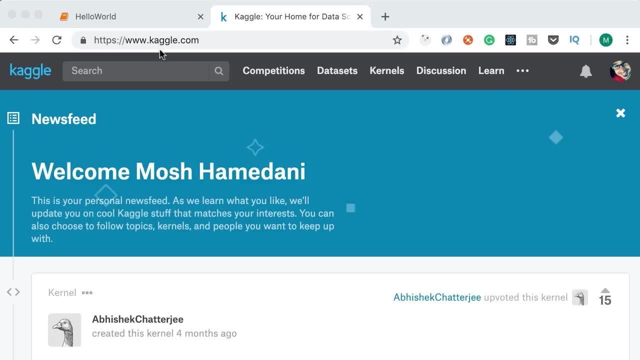 You need to create an account. you need to sign up with Facebook, Google or using a custom email and password. Once you sign up, then come back here on Kagglecom. here on the search bar, search for video game sales. This is the name of a very popular data set. 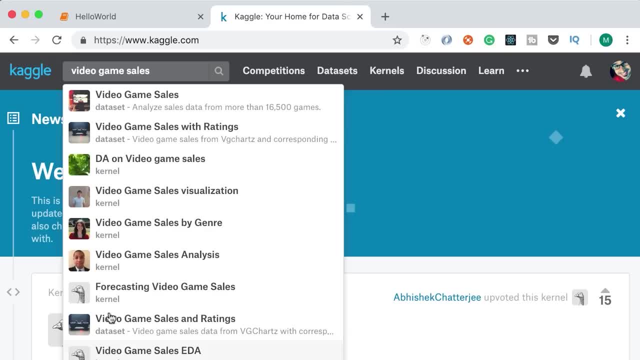 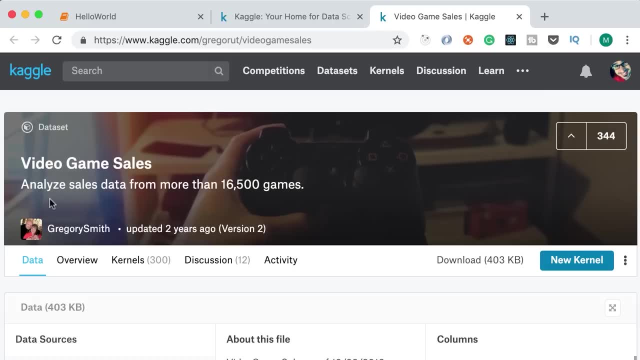 that we are going to use in this lecture. So here on this list, you can see the first item with this kind of reddish icon, so let's go with that. As you can see, this data set includes the sales data for more than. 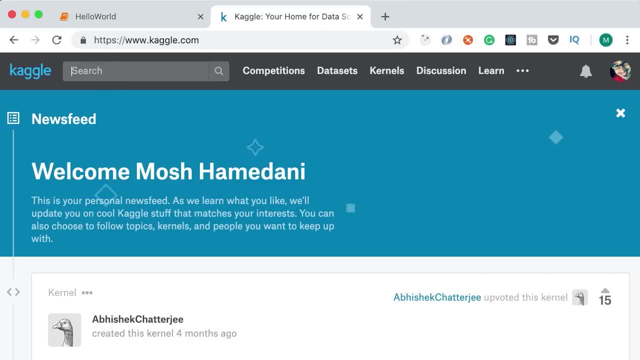 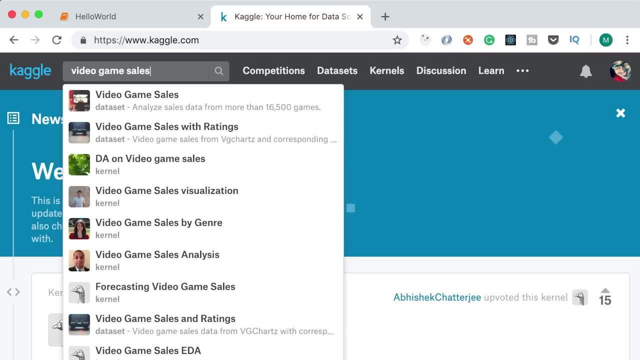 here in the search bar, search for video game sales. This is the name of a very popular data set that we're going to use in this lecture. So here in this list, you can see the first item with this kind of reddish icon. so 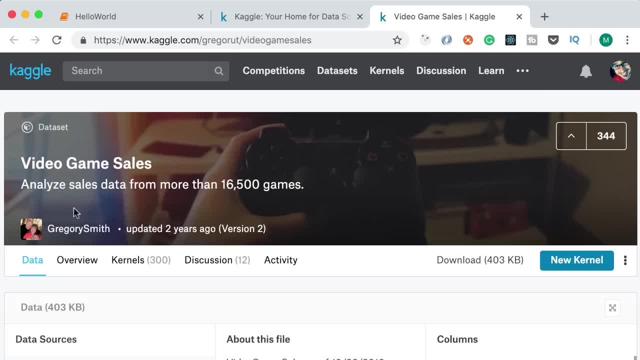 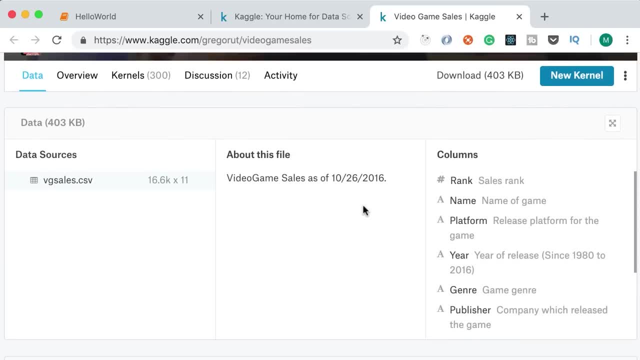 let's go with that. As you can see, this data set includes the sales data for more than 16,000 video games. On this page, you can see the description of various columns in this data set. we have rank, name, platform, year and so on. 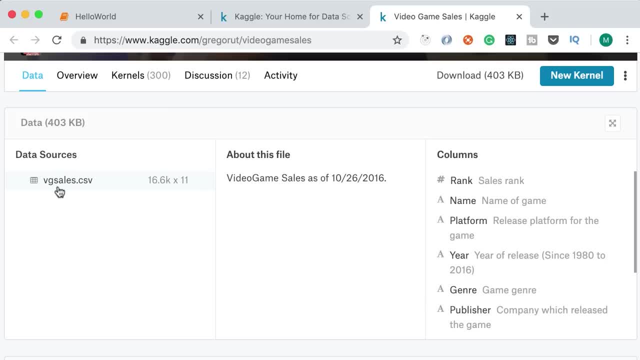 So here's our data source. it's a csv file called vgsalescsv. As you can see, there are a lot of different- over 16,000 rows and 11 columns in this data set. Right below that you can see the first few records of this data set. 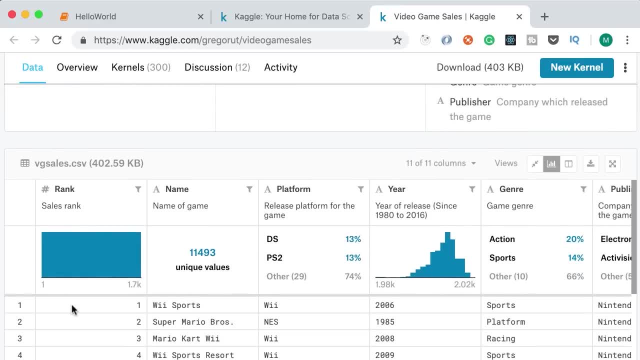 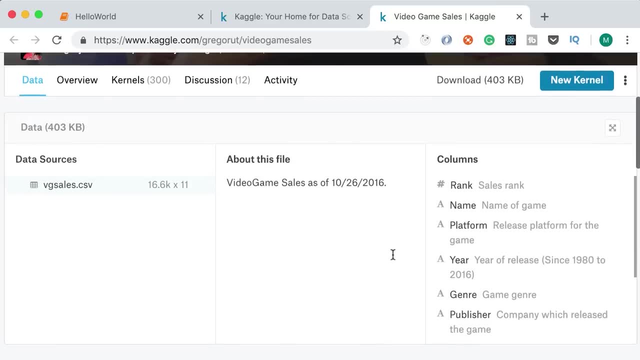 So here's our first record. the ranking for this game is 1,. it's the Wii sports game, for Wii as the platform, and it was released in year 2006.. Now what I want you to do is to go ahead. 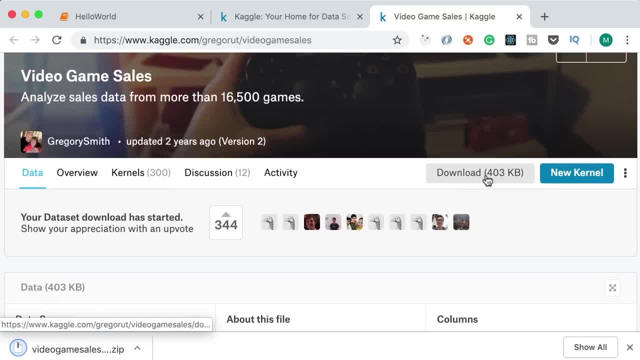 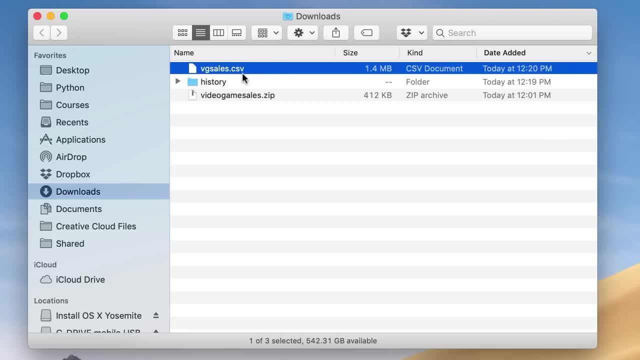 and download this data set and, as I told you before, you need to sign in before you can download this, So this will give you a zip file, as you can see here. Here's our csv file. now I want you to put this right next to your jupiter notebook on my machine, that is, on my 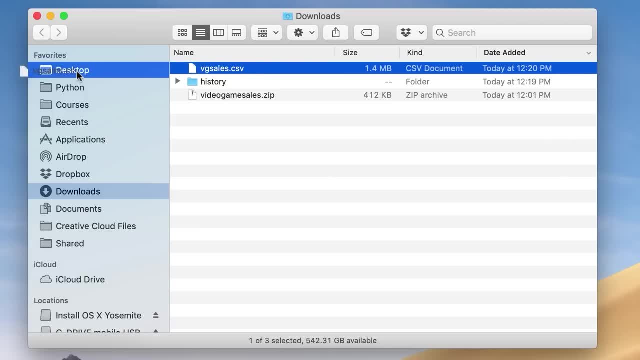 desktop. so I'm going to drag and drop this onto the desktop folder. Now, if you look at the desktop, you can see here's my jupiter hello world notebook, and right next to that we have vgsalescsv With that. 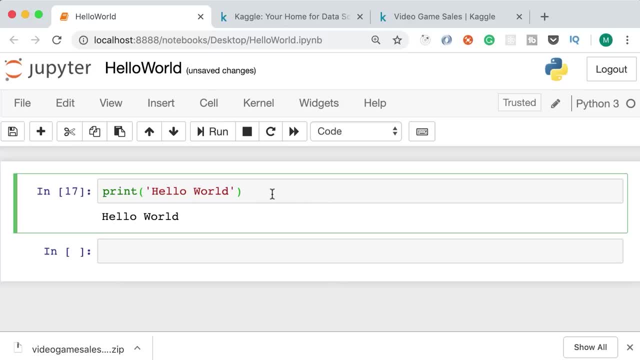 we go back to our jupiter notebook. let's remove the first line and instead import pandas as pd. With this, we're importing pandas module and renaming it to pd, so we don't have to type pandas dot several times in this code. Now let's type pd dot. 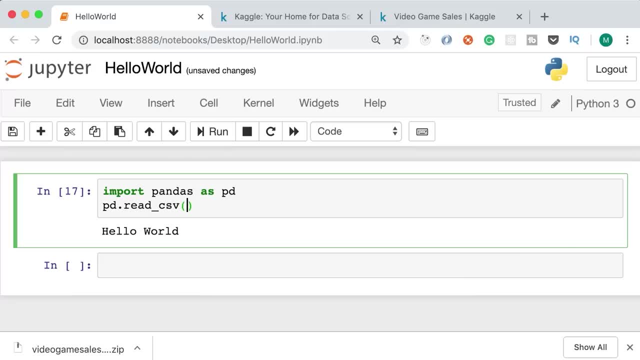 read, underline csv and pass the name of our csv file, that is, vg, salescsv. Now, because this csv file is in the current folder right next to our jupiter notebook, we can easily load it. otherwise we'll have to supply the full. 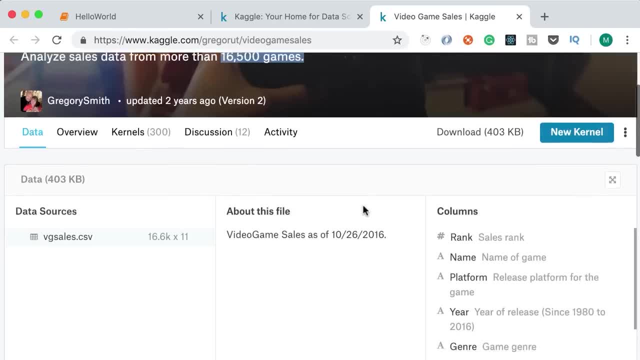 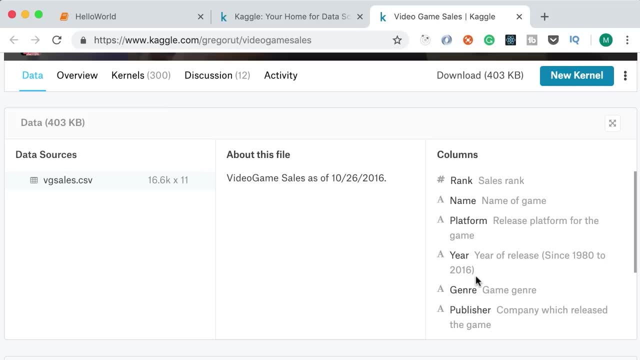 more than 16,000 video games. On this page. you can see the description of various columns. in this dataset. we have rank, name, platform, year and so on. So here's our data source. it's a csv file called vgsalescsv, as you can see. 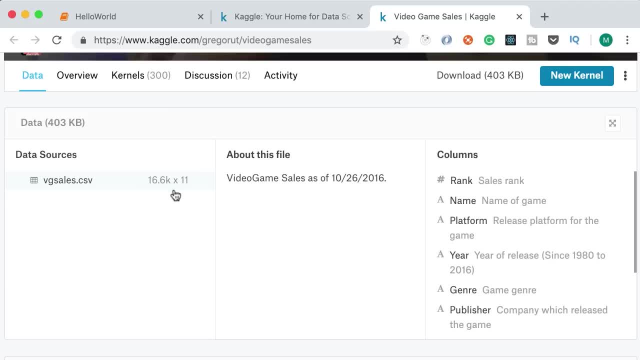 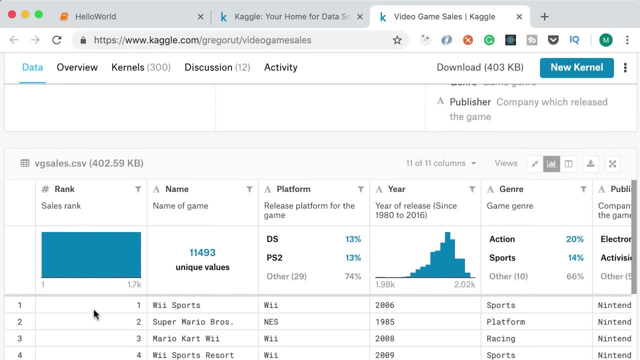 there are over 16,000 rows and 11 columns in this dataset. Right below that you can see the first few records of this dataset. so here's our first record. the ranking for this game is one. it's the Wii sports game for Wii as the platform, and it was released. 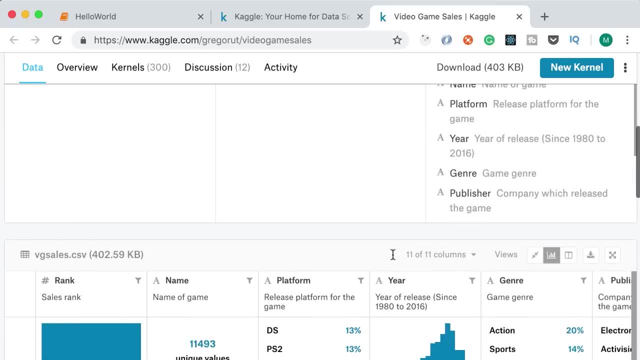 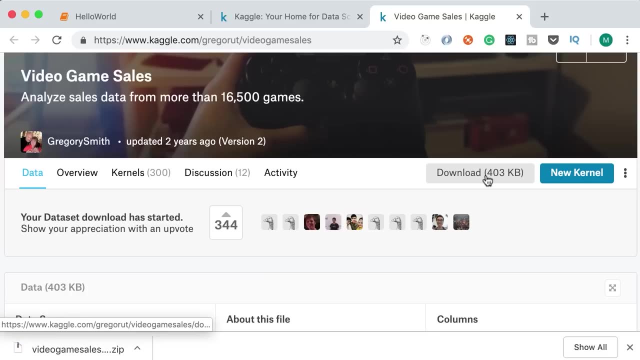 in the year 2006.. Now, what I want you to do is to go ahead and download this dataset and, as I told you before, you need to sign in before you can download this. So this will give you a zip file, as you can see here. here's our csv file. 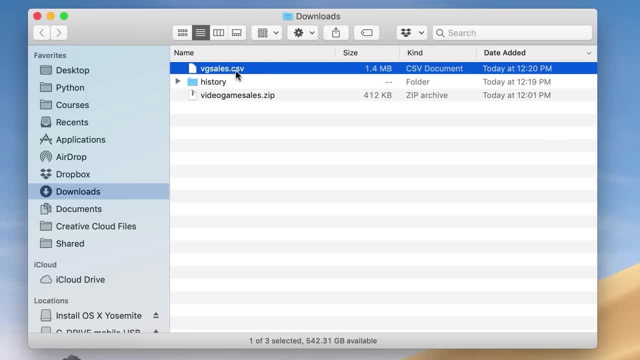 now I want you to put this right next to your jupiter notebook On my machine. that is, on my desktop. so I'm going to drag and drop this onto the desktop folder Now. if you look at the desktop, you can see. here's my jupiter. 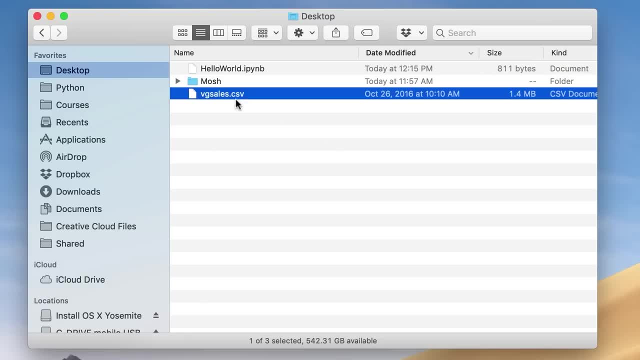 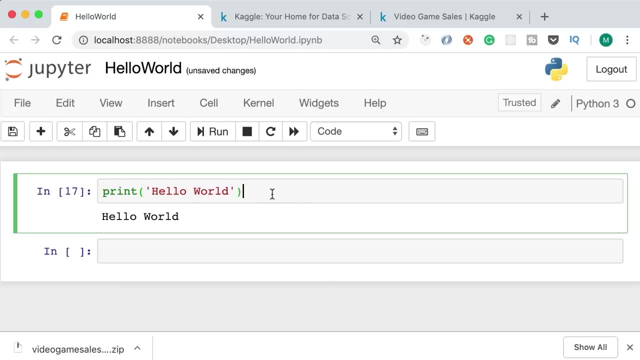 hello world notebook and right next to that we have vgsalescsv. With that we go back to our jupiter notebook. let's remove the first line and instead import pandas as pd. With this we're importing pandas module and renaming it to 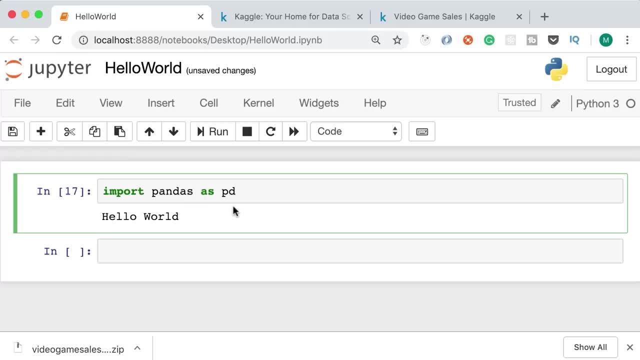 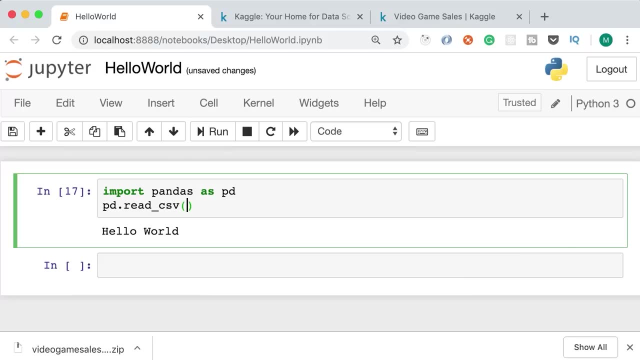 pd, so we don't have to type pandas dot several times in this code. Now let's type pd dot, read, underline csv and pass the name of our csv file, that is, vg sales dot, csv. Now, because this csv file is in the current folder right next to our jupiter notebook. 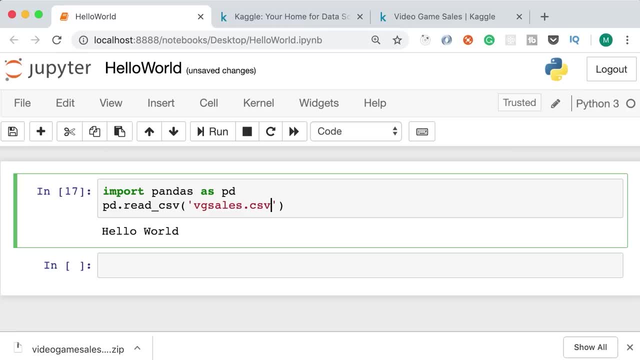 we can easily load it, otherwise we'll have to supply the full path to this file. So this returns a data frame object which is like an excel spreadsheet. let me show you. so we store it here and then we can simply type. 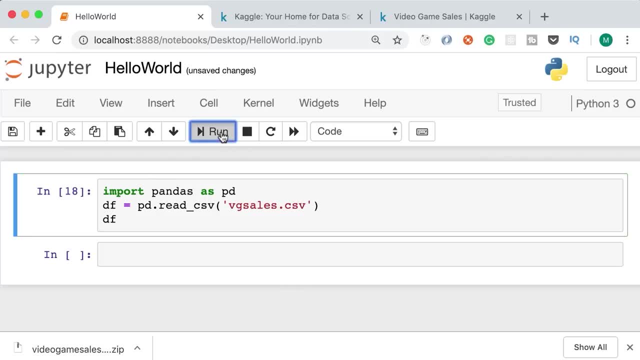 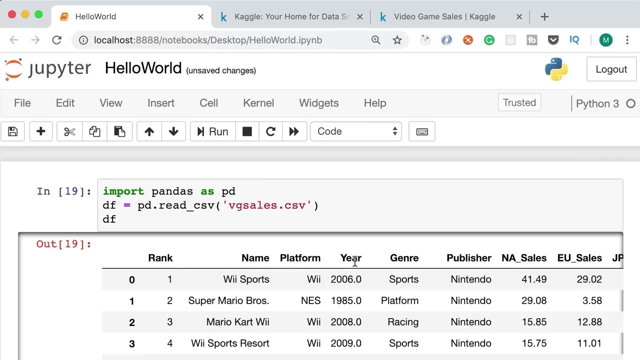 df to inspect it. So one more time, let's run this program. here's our data frame with these rows and columns, so we have rank, name, platform and so on. Now this data frame object has lots of attributes and methods that we're not going to cover in this tutorial. 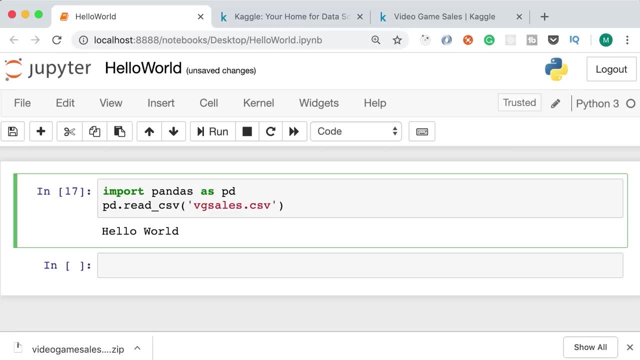 path to this file. So this returns a data frame object which is like an excel spreadsheet. Let me show you. So we store it here and then we can simply type df to inspect it. So one more time, let's run this program. 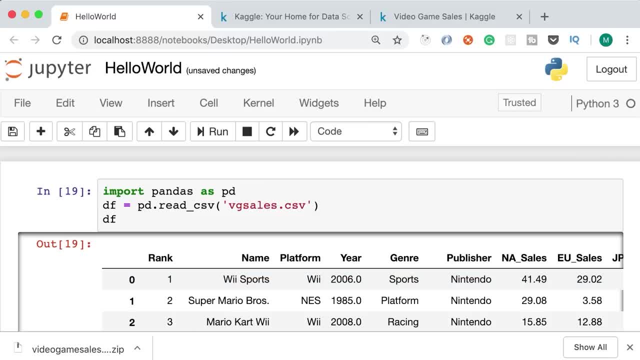 here's our data frame with these rows and columns, so we have rank, name, platform and so on. Now this data frame object has lots of attributes and methods that we're not going to cover in this tutorial. that's really beyond the scope of what we're going to do, So I leave it up to you to read. 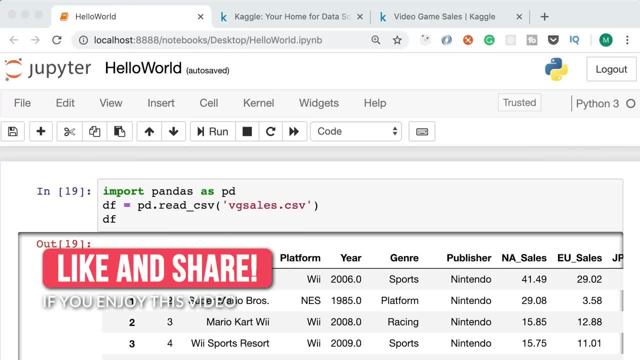 pandas documentation or follow other tutorials to learn about pandas data frames. But in this lecture I'm going to show you some of the most useful methods and attributes. The first one is shape, So shape. let's run this one more time. So here's the shape of this data set We have. 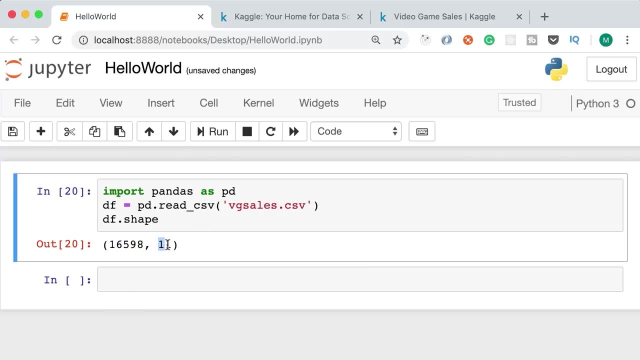 over 16,000 records and 11 columns. Technically, this is a two dimensional array of 16,000 and 11.. Okay, Now you can see. here we have another segment for writing code, so we don't have to write all the code in the first segment. 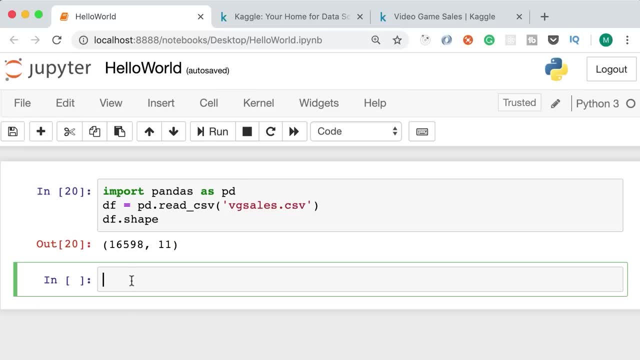 So here in the second segment we can call one of the methods of the data frame, that is, dfdescribe. Now when we run this program we can see the output for each segment right next to it. So here's our first segment. 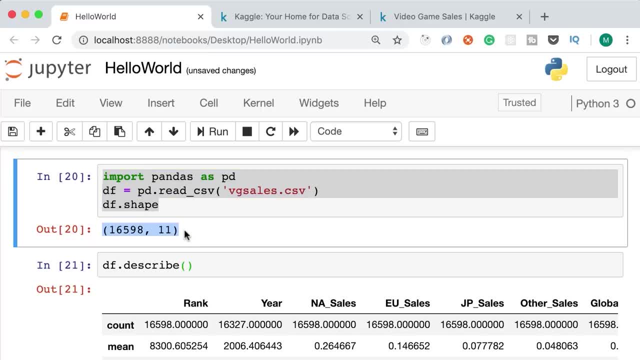 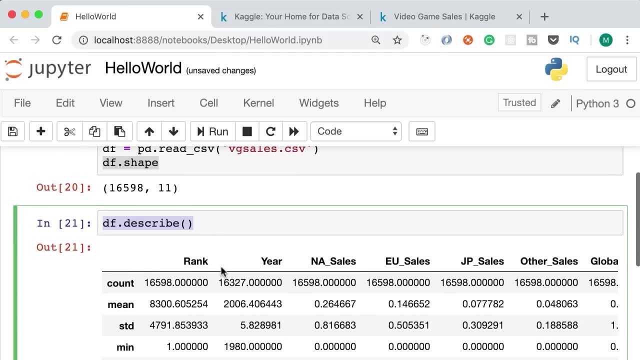 here we have these three lines, and this is the output of the last line. Below that we have our second segment, here we're calling the describe method, and right below that we have the output of this segment. So this is the beauty of jupiter: we can easily 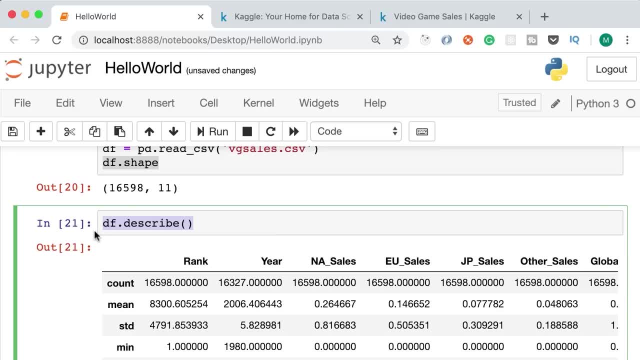 visualize our data. Doing this with vs code and terminal windows is really tedious and clunky. So what is this describe method returning? Basically, it's returning some basic information about each column in this data set. So, as you saw earlier, we have columns like rank, year and so on. 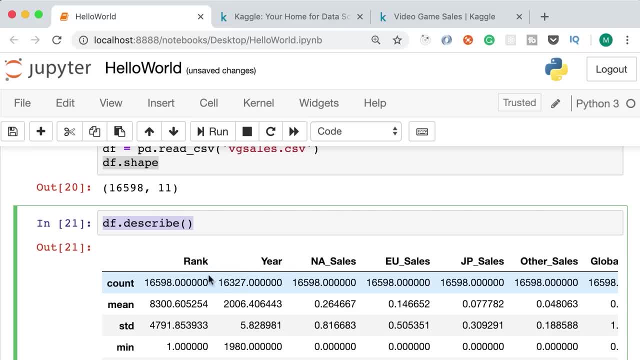 These are the columns with numerical values. Now for each column we have the count, which is the number of records in that column. you can see: our rank column has 16,598 records, whereas the year column has 16,327 records. So this shows that some of our records 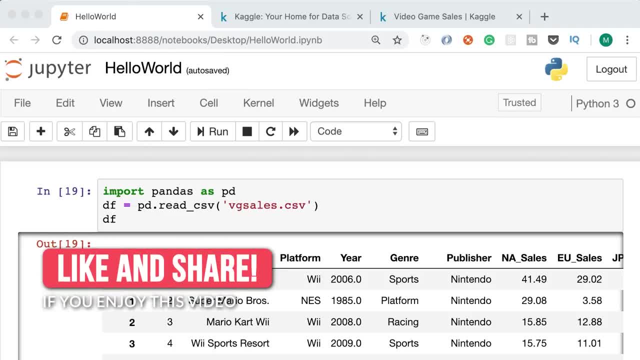 that's really beyond the scope of what we're going to do. So I leave it up to you to read pandas documentation or follow other tutorials to learn about pandas data frames, But in this lecture I'm going to show you some of the more. 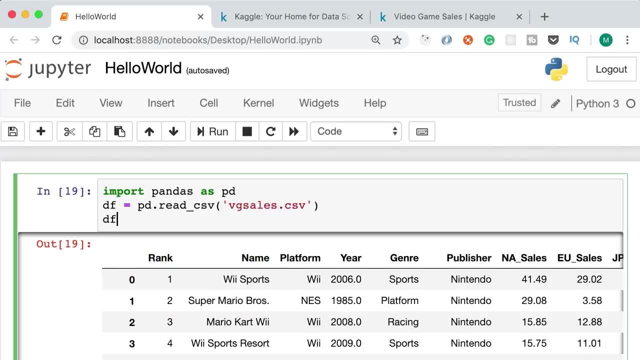 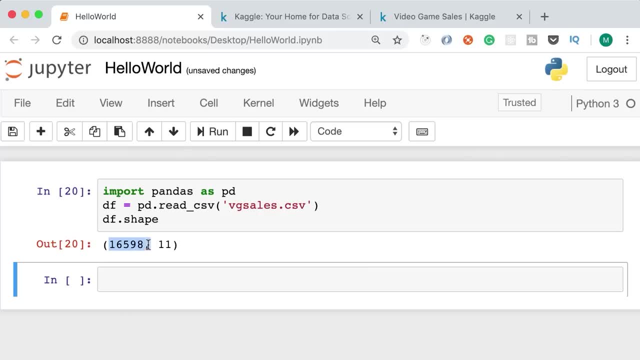 useful methods and attributes. The first one is shape. So shape. let's run this one more time. so here's the shape of this data set. we have over 16,000 records and 11 columns. Technically, this is a two dimensional array. 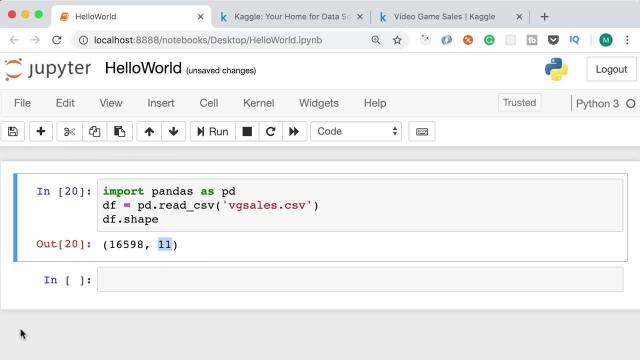 of 16,000 and 11.. Okay, Now you can see, here we have another segment for writing code, so we don't have to write all the code in the first segment. so here in the second segment we can call one of the methods of the data frame, that is, dfdescribe. 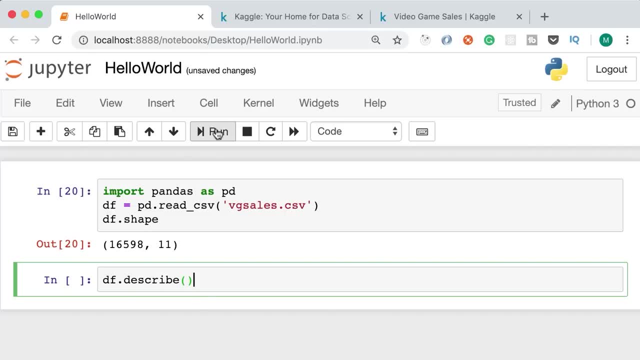 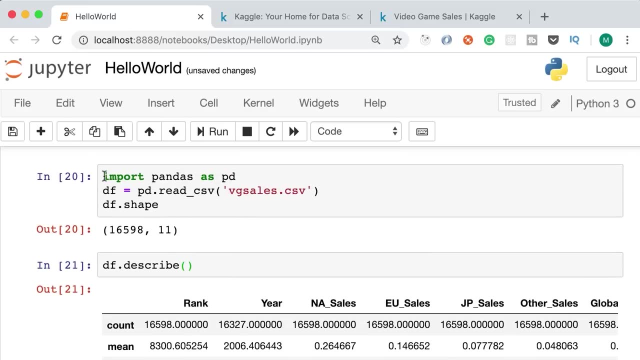 Now, when we run this program, we can see the output for each segment right next to it. So here's our first segment. here we have these three lines and this is the output of the last line. Below that we have our second segment. here we're calling the describe method, and right below that we have 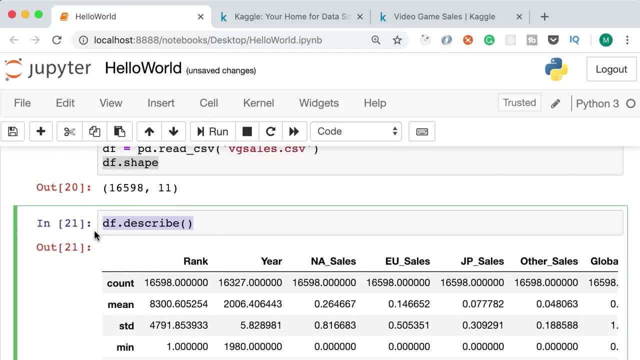 the output of this segment. So this is the beauty of Jupiter: we can easily visualize our data. Doing this with vs code and terminal windows is really tedious and clunky. So what is this describe method returning? Basically, it's returning some basic information about each column. 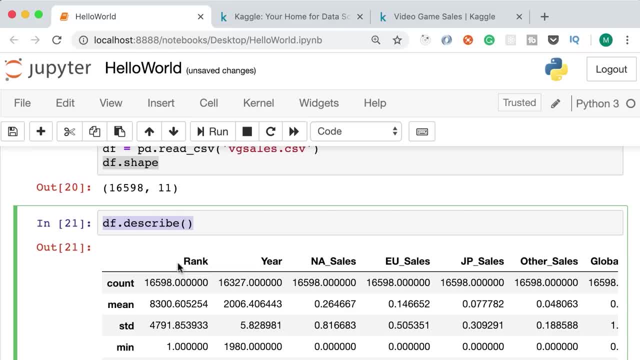 in this data set. So, as you saw earlier, we have columns like rank, year and so on. These are the columns with numerical values. Now, for each column we have the count, which is the number of records in that column. you can see: our rank column has 16,000,. 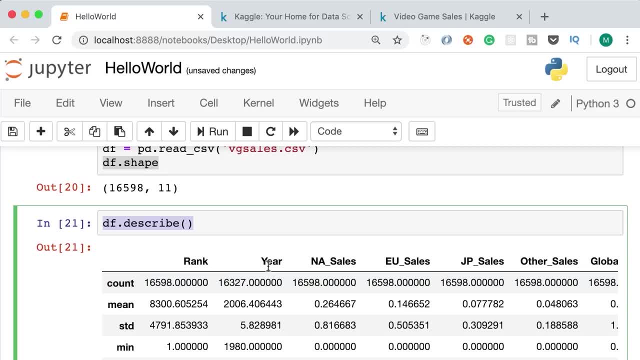 500, and 9080. Whereas the year column has 16,000, 327 records. So this shows that some of our records don't have the value. for the year column We have no values. So in a real data science or machine learning project we'll have to use some techniques to 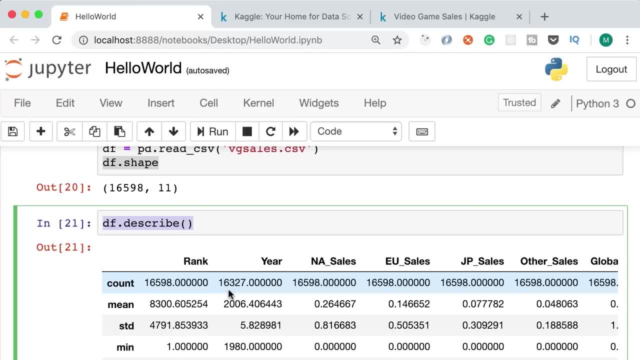 don't have the value for the year column. We have no values, So in a real data science or machine learning project we'll have to use some techniques to clean up our data set. One option is to remove the records that don't have a value for the year column, or we can assign them a default. 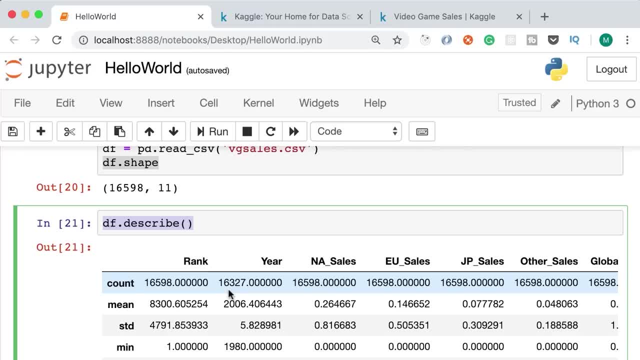 value. That really depends on the project. Now, another attribute for each column is mean. so this is the average of all the values. Now, in the case of the rank column, this value doesn't really matter. but look at the year, So the average year for all these video games in our data set. 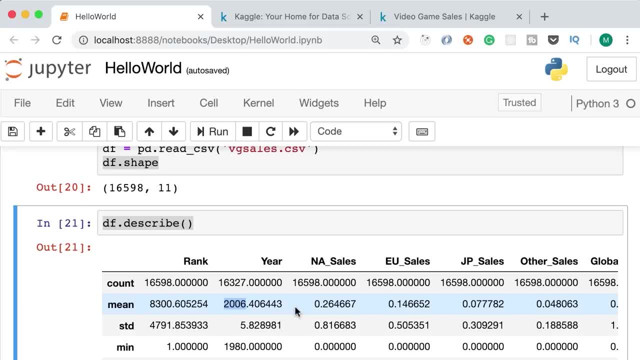 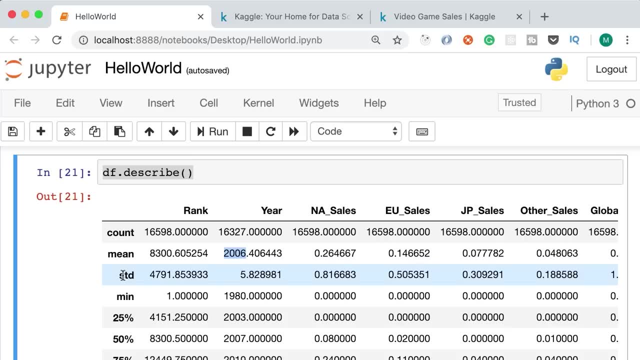 is 2006, and this might be important in the problem we're trying to solve. We also have standard deviation, which is a measure to quantify the amount of variation in our set of values. Below that we have min as an example, the minimum value for the year. 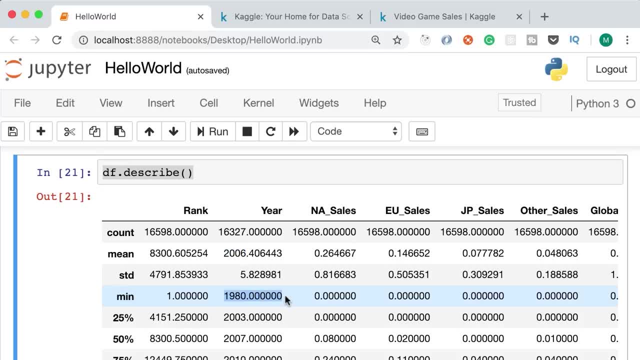 column is 1980.. So quite often when we work with a new data set, we call the describe method to get some basic statistics about our data. Let me show you another useful attribute. So in the next segment let's type dfvalues. 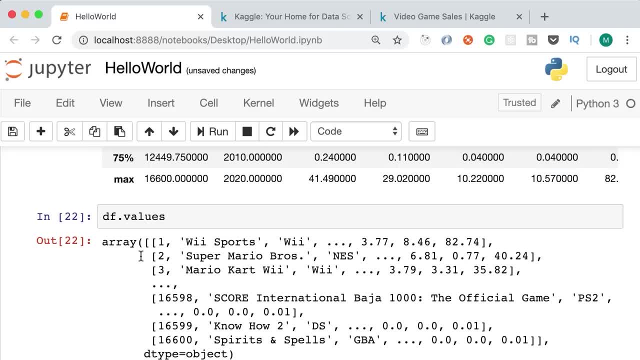 let's run this. as you can see, this returns a two dimensional array. this square bracket indicates the outer array, and the second one represents the inner array. So the first element in our outer array is an array itself. these are the values in this array, which 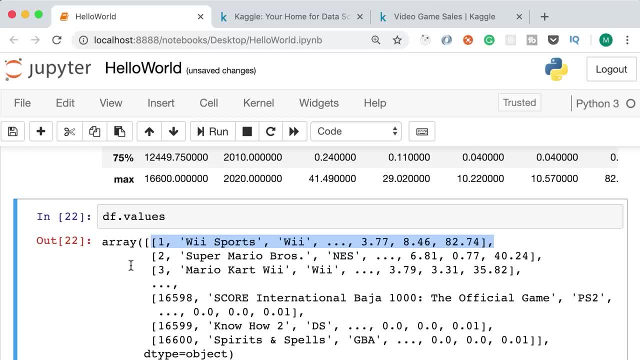 basically represent the first row in our data set. So the video game we're ranking, one which is called Wii Sports. So this was a basic overview of Pandas data frames. In the next section I'm going to show you some of the useful shortcuts of Jupiter. 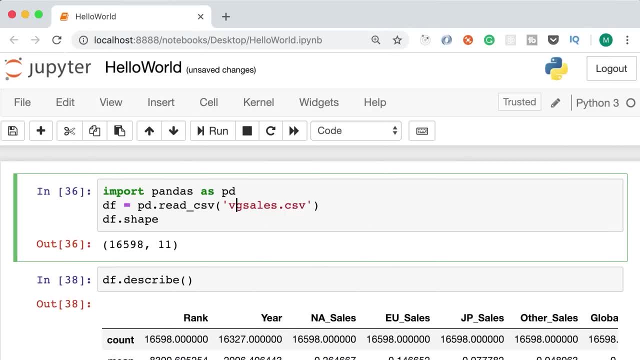 In this lecture, I'm going to show you some of the most useful shortcuts in Jupiter. Now, the first thing I want you to pay attention to is this green bar on the left. This indicates that this cell is currently in the edit mode, So we can write code here Now, if we. 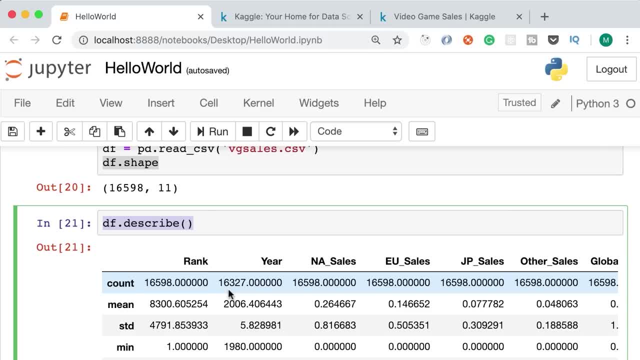 clean up our data set. One option is to remove the records that don't have a value for the year column, or we can assign them a default value. That really depends on the project. Now, another attribute for each column is mean, so this is the average of all the values. Now, in the case, 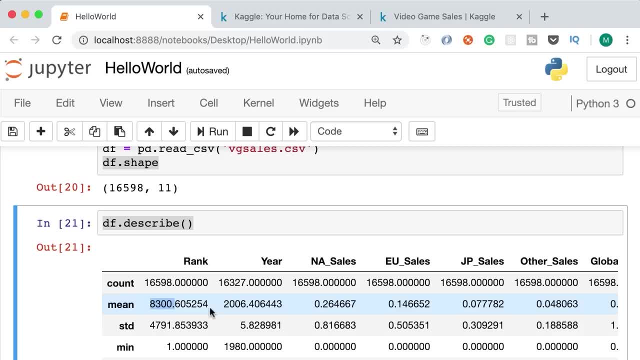 of the rank column. this value doesn't really matter, but look at the year. So the average year for all these video games in our data set is 2006,, and this might be important in the problem we're trying to solve. We also have standard deviation, which is a measure to quantify. 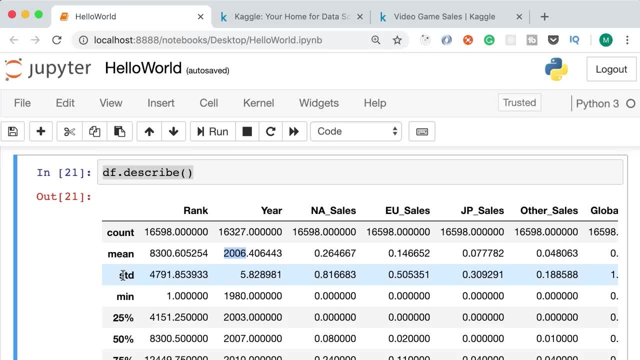 the amount of variation in our set of values Below that we have min. as an example, the minimum value for the year column is 1980. So quite often when we work with a new data set we call the describe method to get some basic statistics about. 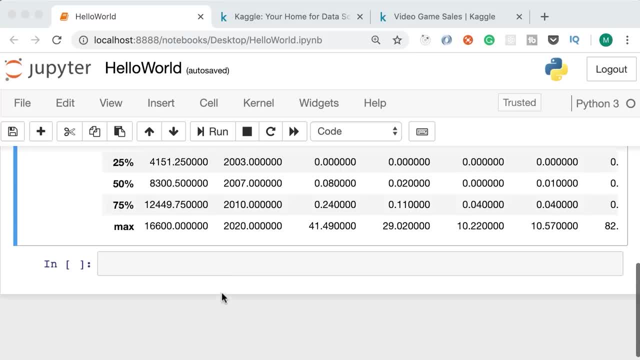 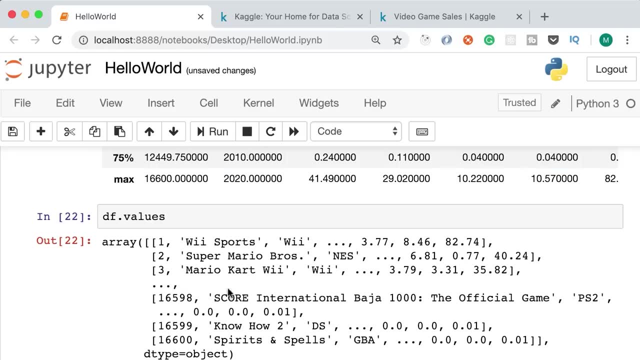 our data. Let me show you another useful attribute. So in the next segment, let's type dfvalues. let's run this. as you can see, this returns a two dimensional array. this square bracket indicates the outer array and the second one represents the inner array. 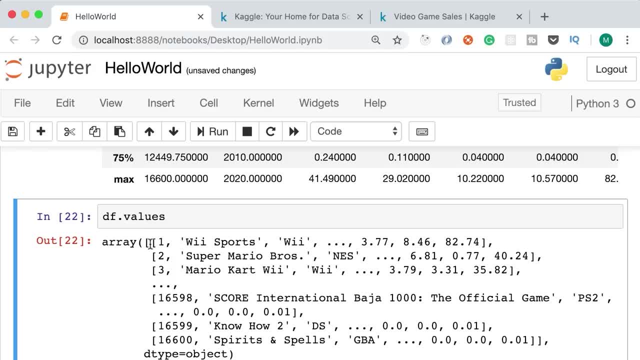 So the first element in our outer array is an array itself. these are the values in this array which basically represent the first row in our data set. So the video game we're ranking, one which is called Wii Sports. So this was a basic overview. 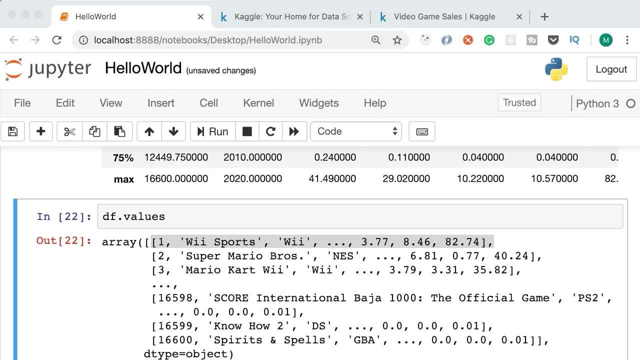 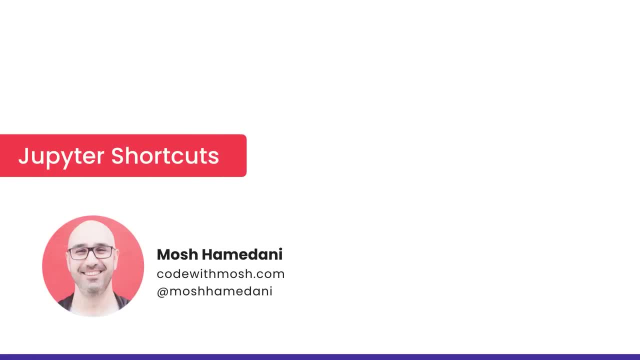 of pandas data frames. In the next lecture, I'm going to show you some of the useful shortcuts of Jupiter. In this lecture, I'm going to show you some of the most useful shortcuts of Jupiter. In this lecture, I'm going to show you some of the most useful shortcuts of Jupiter. 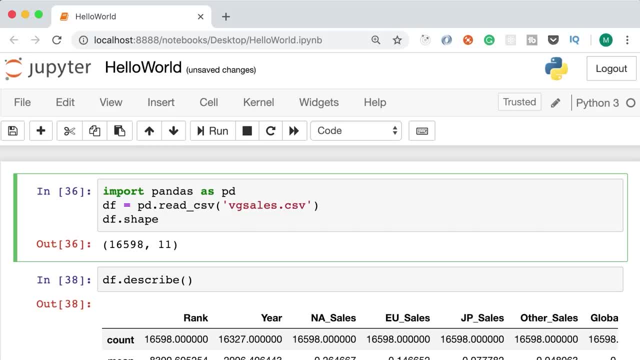 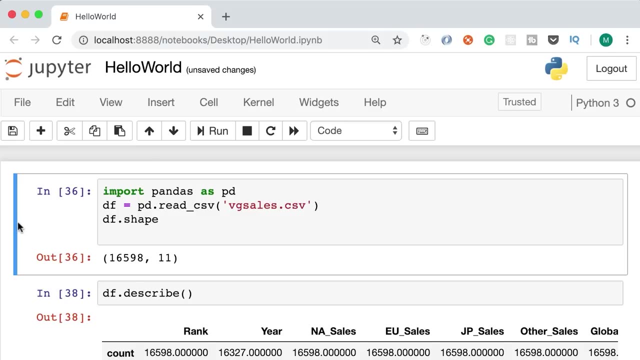 Now, the first thing I want you to pay attention to is this green bar on the left. This indicates that this cell is currently in the edit mode, so we can write code here. Now, if we press the escape key, green turns to blue, and that means this cell is currently in the command mode. 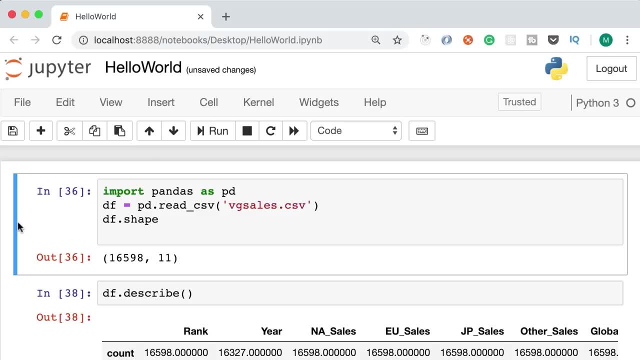 press the escape key, green turns to blue and that means this cell is currently in the command mode. So basically, the activated cell can be either in the edit mode or the command mode. Depending on the mode, we have different shortcuts. So here we're. 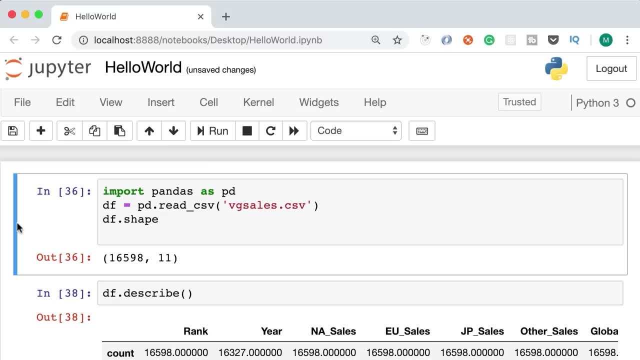 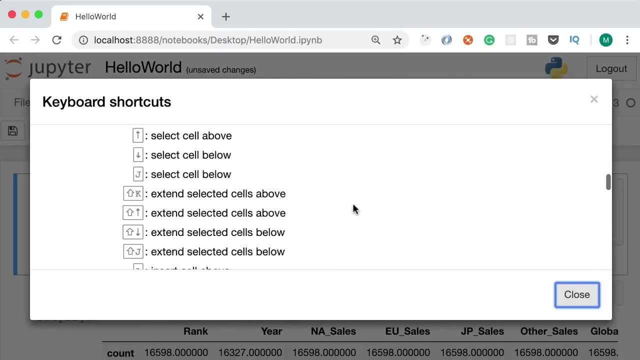 So basically, the activated cell can be either in the edit mode or the command mode. Depending on the mode, we have different shortcuts. So here we're currently in the command mode. If we press H, we can see the list of all the keyboard shortcuts Right above. 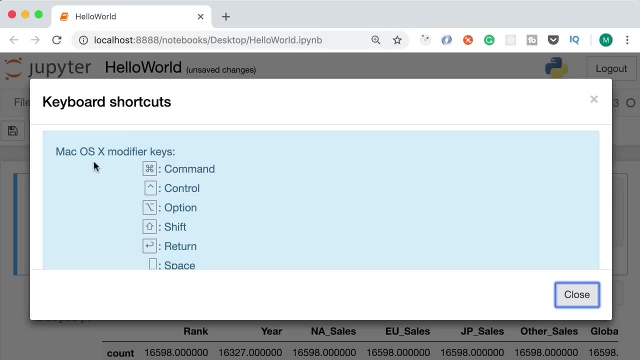 this list we can see macOS modifier keys. these are the extra keys that we have on a Mac keyboard. If you're a Windows user, you're not going to see this. So, as an example, here is the shape of the command key. this is control. this is option. 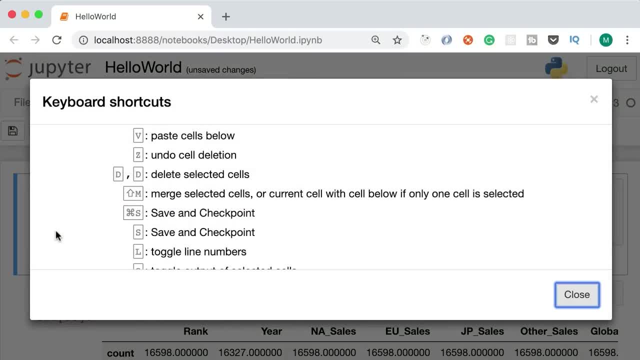 currently in the command mode. If we press h, we can see the list of all the keyboard shortcuts. Right above this list we can see macOS modifier keys. these are the extra keys that we have on a Mac keyboard. If you're a Windows user, you're not going to see this. So as an example here, 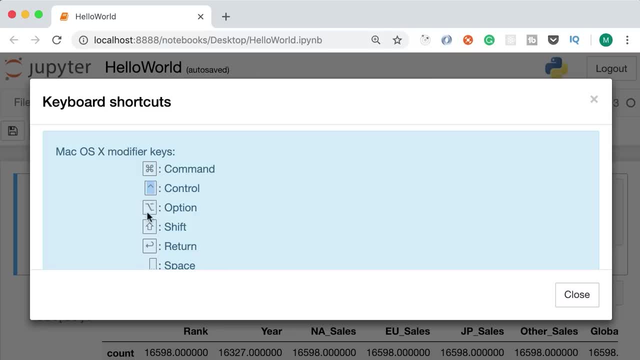 is the shape of the command key, this is control, this is option, and so on. With this guideline, you can easily understand the shortcut associated with each command. Let me show you. So here we have all the commands when a cell is in the command mode. 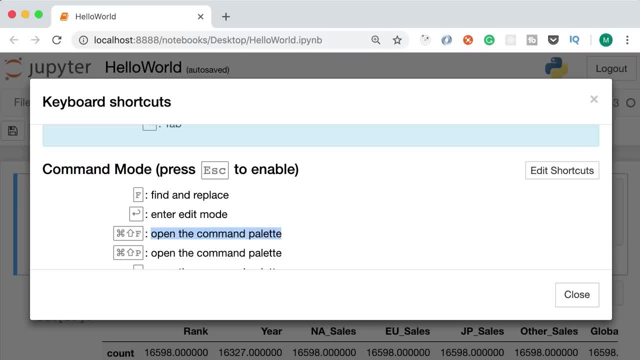 For example, we have this command: open the command palette. This is exactly like the command palette that we have in VS code. Here's a shortcut to execute this command, That is, command shift and f. Okay, So here we have lots of shortcuts. of course you're not. 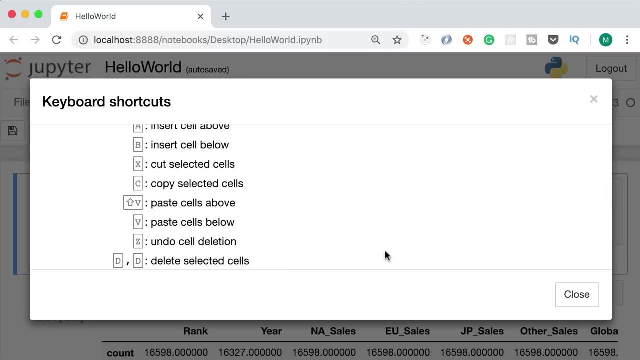 going to use all of them all the time, but it's good to have a quick look here to see what is available for you. With these shortcuts, you can write code much faster, So let me show you some of the most useful ones. I'm going to close this. 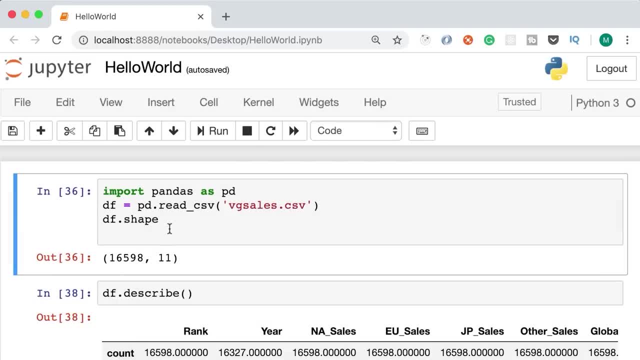 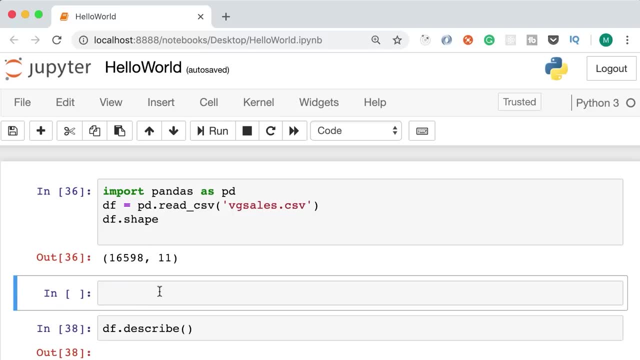 Now, with our first cell in the command mode, I'm going to press b and this inserts a new cell below this cell. We can also go back to our first cell. press escape. now the cell is in the command mode. we can insert an empty cell above this cell by pressing a. 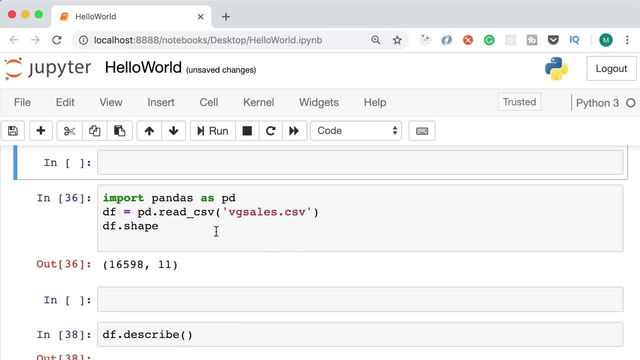 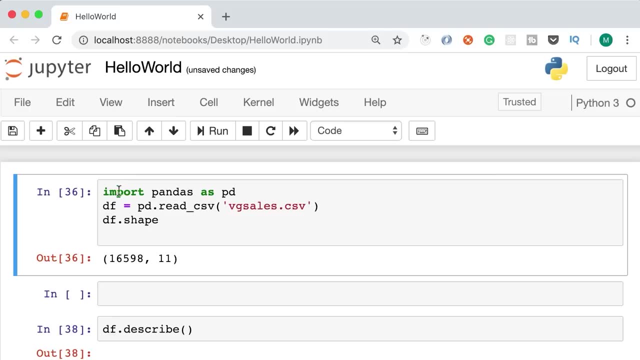 So either a or b, a for above and b for below. Okay, Now, if you don't want this cell, you can press d twice to delete it. Like this: Now, in this cell I'm going to print a hello world message, So print. 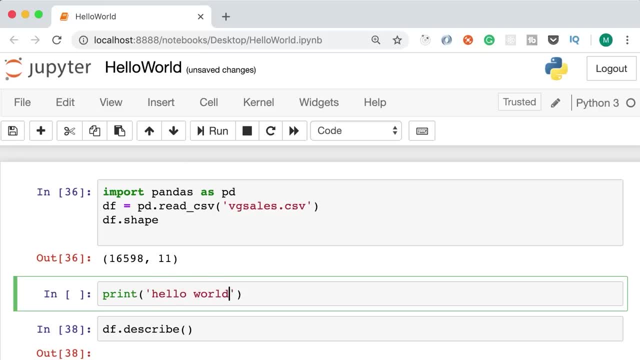 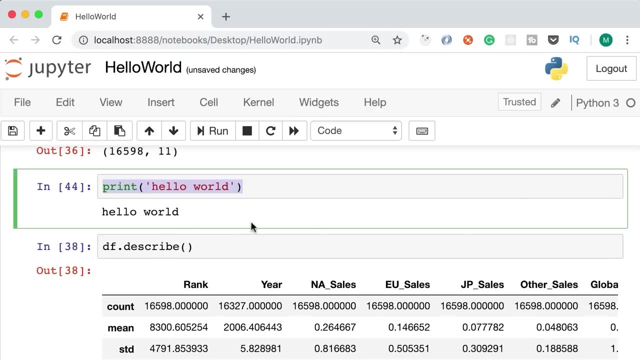 hello world. Now to run the code in this cell, we can click on the run button here. so here's our print function, and right below that you can see the output of this function. But note that when you run a cell, 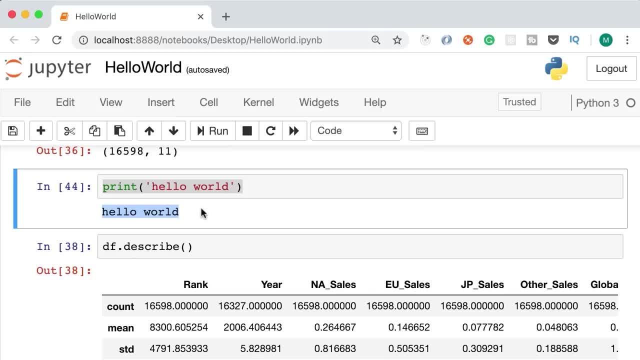 this will only execute the code in that cell. In other words, the code in other cells will not be executed. Let me show you what I mean. So in the cell below this cell, I'm going to delete the call to the describe method. Instead, I'm going to print: 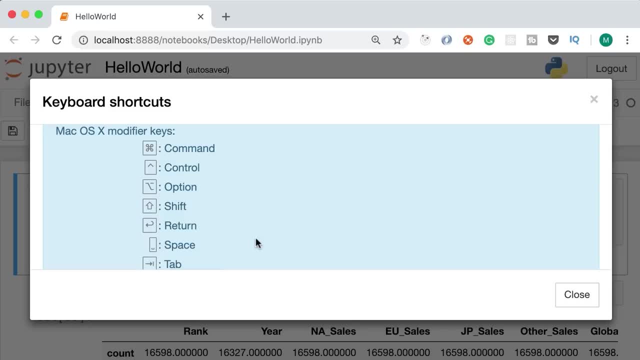 and so on. With this guideline, you can easily understand the shortcut associated with each command. Let me show you So. here we have all the commands. when a cell is in the command mode, For example, we have this command: open the command palette. 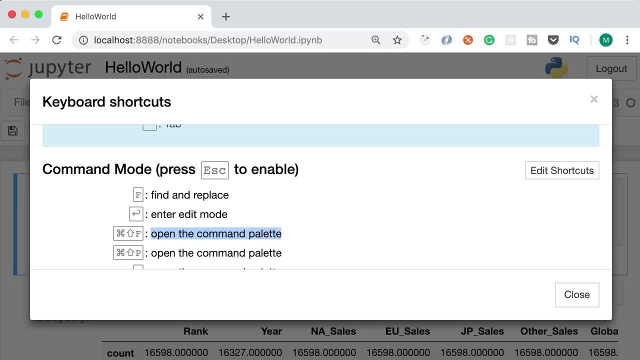 This is exactly like the command palette that we have in VS code. Here's a shortcut to execute this command, That is, command shift and F. Okay, So here we have lots of shortcuts. of course, you're not going to use all of them all the time, but it's good to have a quick look. 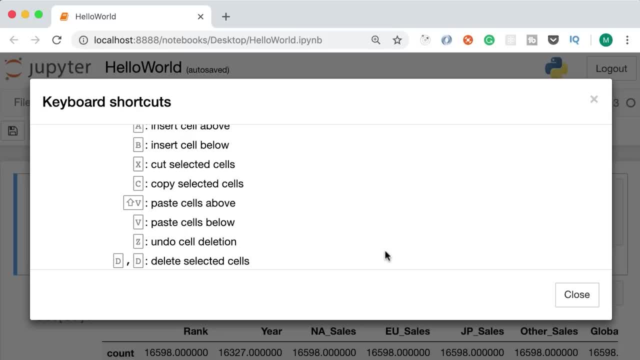 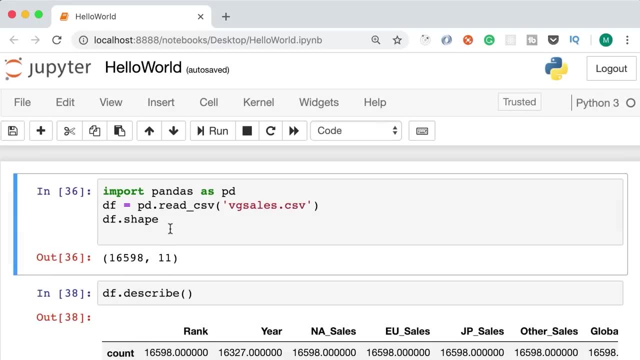 here to see what is available for you. With this shortcut you can write code much faster. So let me show you some of the most useful ones. I'm going to close this Now with our first cell in the command mode. I'm going to press. 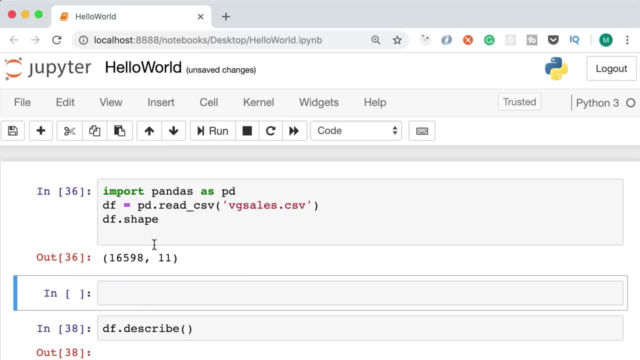 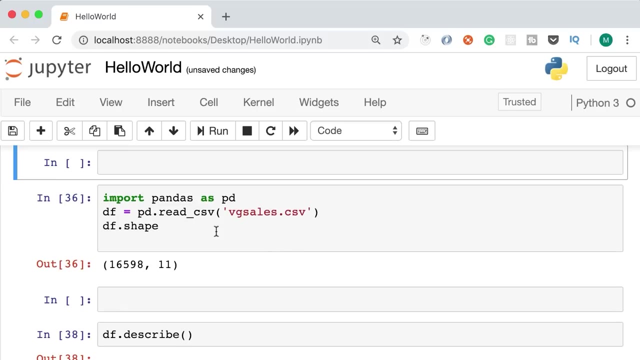 B and this inserts a new cell below this cell. We can also go back to our first cell press escape. now the cell is in the command mode. we can insert an empty cell above this cell by pressing A. So either A or B, A for above and B for below. okay, 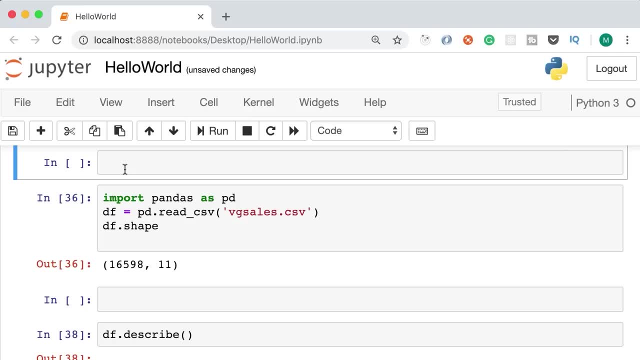 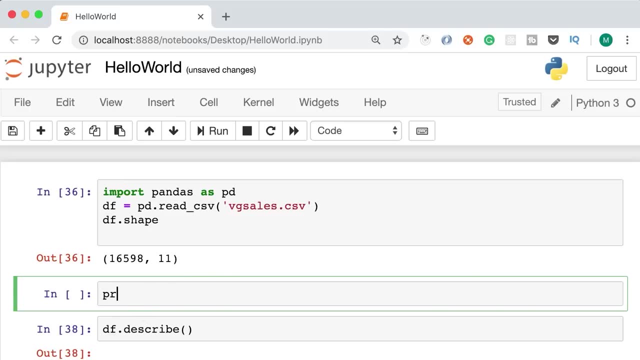 Now, if you don't want this cell, you can press D twice to delete it. Like this: Now in this cell I'm going to print a hello world message, so print hello world Now to run the code in this cell. we can. 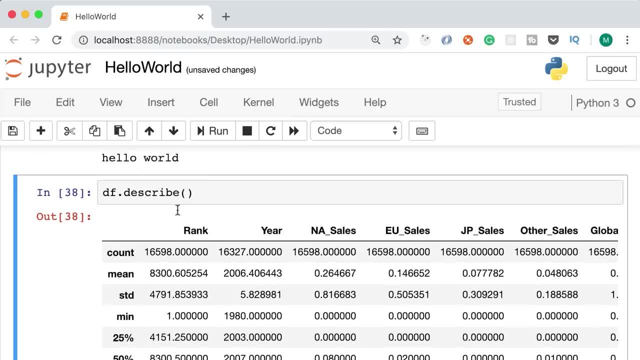 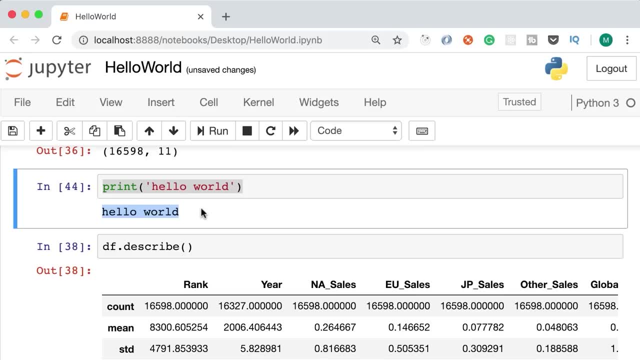 click on the run button here. so here's our print function, and right below that you can see the output of this function. But note that when you run a cell, this will only execute the code in that cell. In other words, the code in other cells will not be executed. Let me show you what I mean. 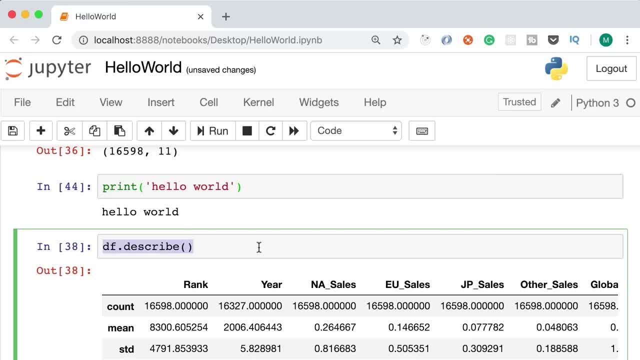 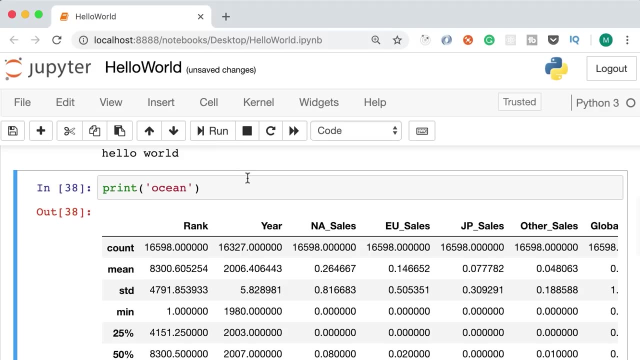 So in the cell below this cell I'm going to delete the call to the describe method. Instead I'm going to print ocean. Now I'm going to put the cursor back in this cell where we print the hello world message and run this cell So we can see hello world is displayed here. 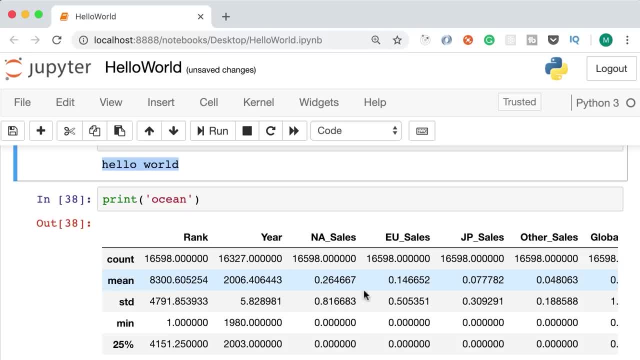 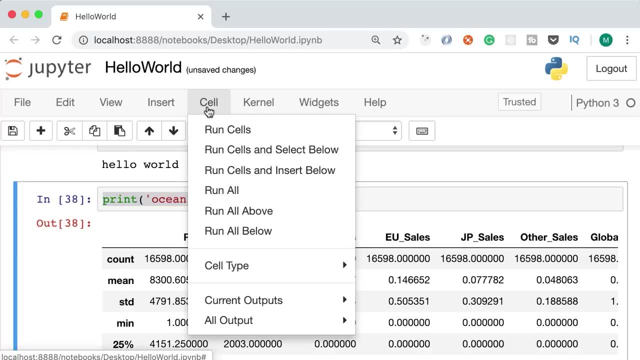 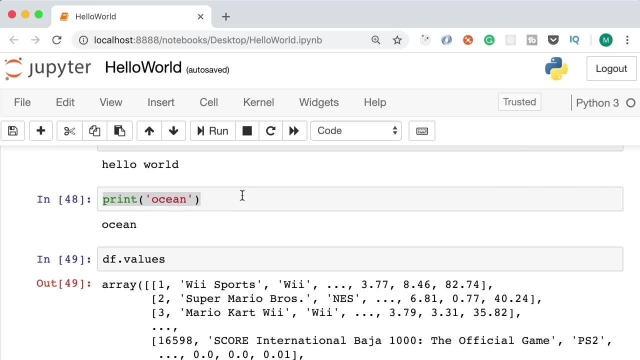 but the cell below is still displaying the describe table, so we don't see the changes here. Now, to solve this problem, we can go to the cell menu on the top and run all cells together. This can work for small projects, but sometimes you're working with a large data set, so if you want to run all these cells, 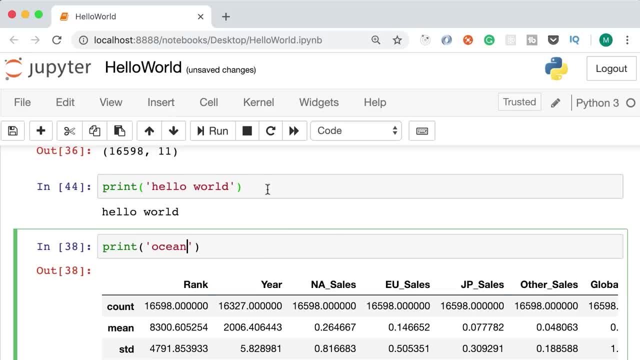 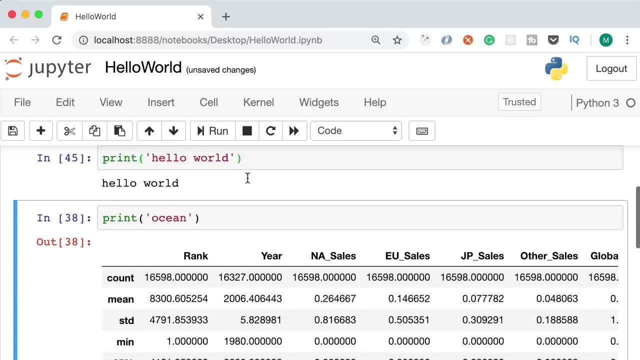 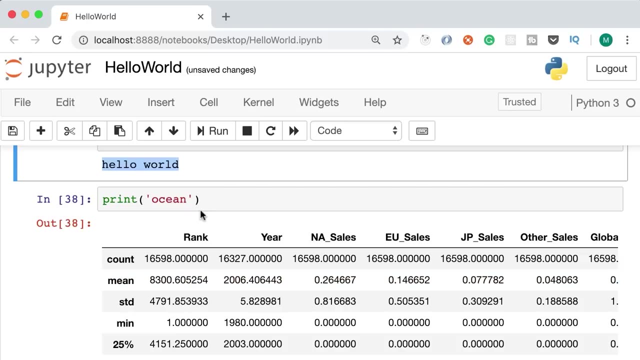 ocean. Now I'm going to put the cursor back in this cell where we print the hello world message and run this cell So we can see hello world is displayed here, but the cell below is still displaying the describe table, so we don't see the changes here. Now to solve. 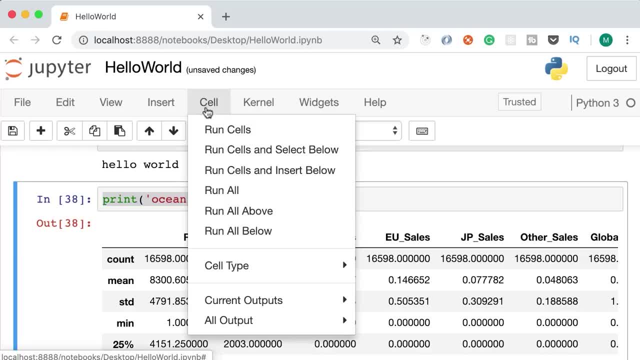 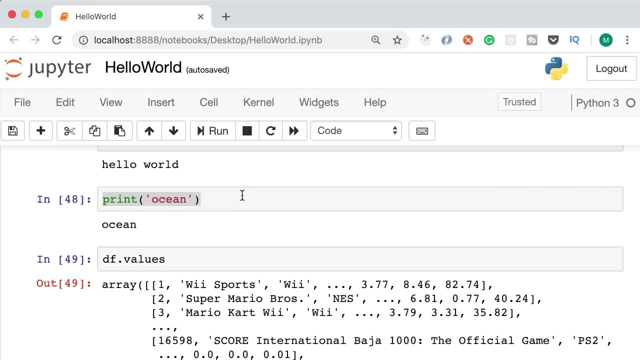 this problem. we can go to the cell menu on the top and run all cells together. This can work for small projects, but sometimes you're working with a large data set, so if you want to run all these cells together, it's going to take a lot of time. That is the reason. 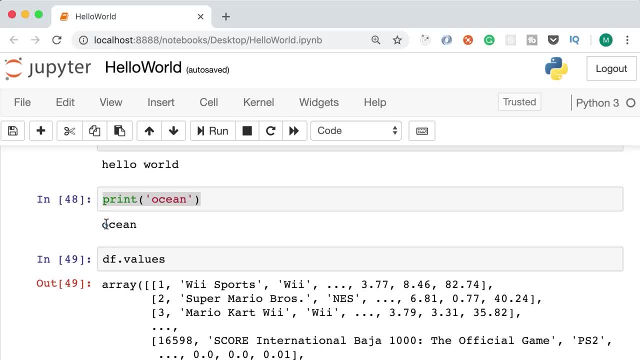 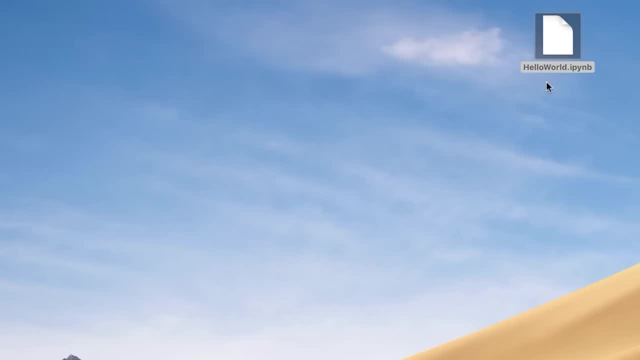 Jupiter saves the output of each cell, so we don't have to rerun that code if it hasn't changed. So this notebook file that we have here includes our source code organized in cells, as well as the output for each cell. That is why it's different from a regular 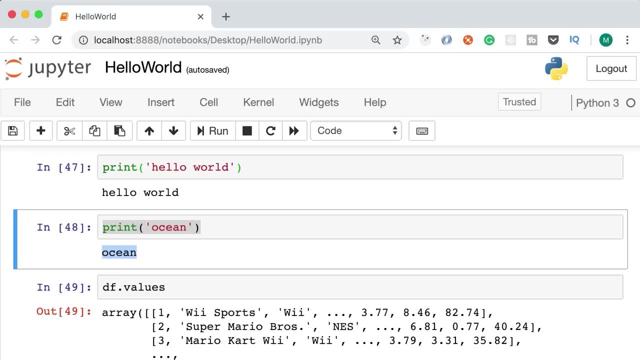 pie file where we only have the source code. Here we also have auto completion and intellisense. So in the cell let's call DF data frame dot. now if you press tab you can see all of the attributes and methods in this object. So let's call. 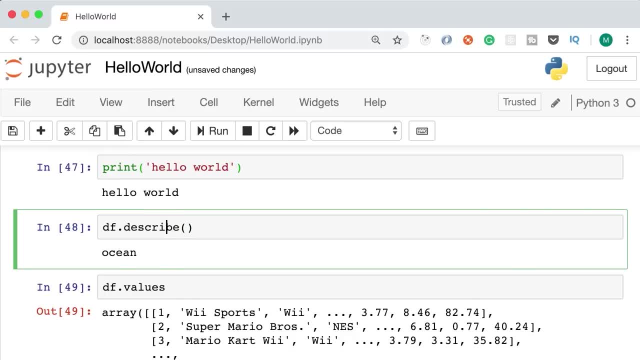 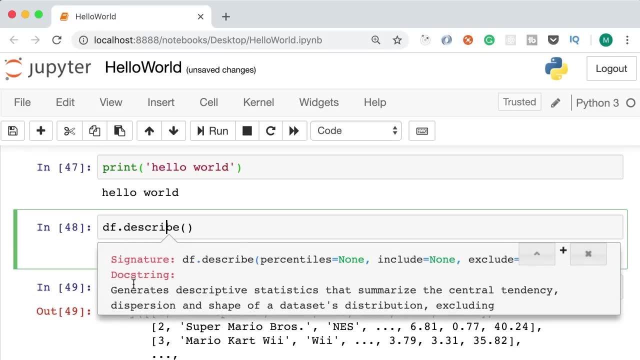 describe. now with the cursor on the name of the method we can press shift and tab to see this tool tip that describes what this method does and what parameter it takes. So here in front of signature you can see the describe method. these are the parameters. 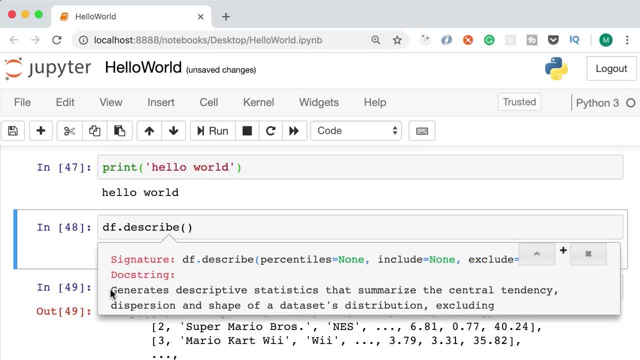 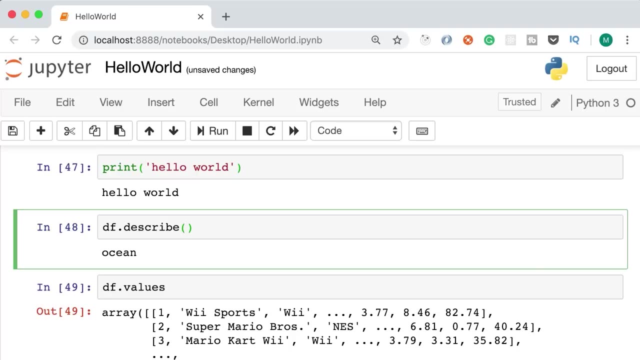 and their default value, and right below that you can see the description of what this method does. In this case, it generates descriptive statistics that summarize the central tendency, and so on. Similar to VS code, we can also convert a line to comment by pressing command and slash on Mac, or control slash. 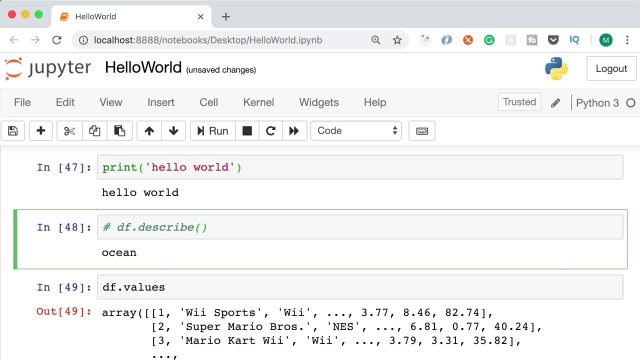 on Windows like this. Now this line is a comment. we can press the same shortcut one more time to remove the comment. So these were some of the most useful shortcuts in Jupyter. Now, over the next few lectures, we're going to work on a real machine learning project. but before we get, 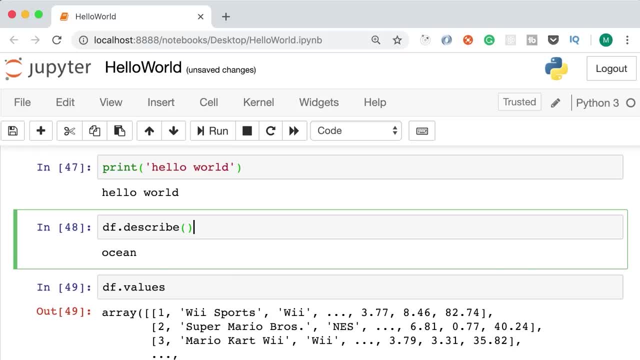 there, let's delete all the cells here, so we start with only a single empty cell. So here in this cell, first I'm going to press the escape button. now the cell is blue, so we're in the command mode and we can delete the cell by pressing. 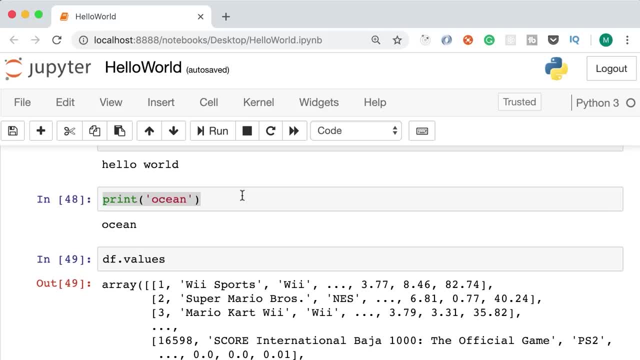 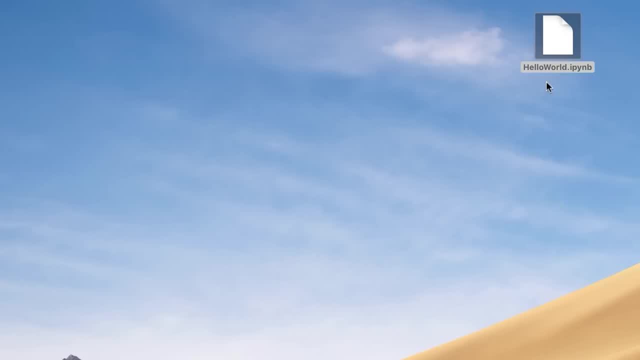 together. it's going to take a lot of time. That is the reason. Jupiter saves the output of each cell, so we don't have to rerun that code if it hasn't changed. So this notebook file that we have here includes our source code organized in cells, as well as the output. 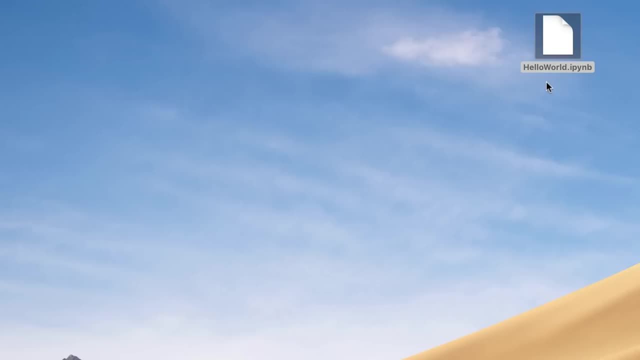 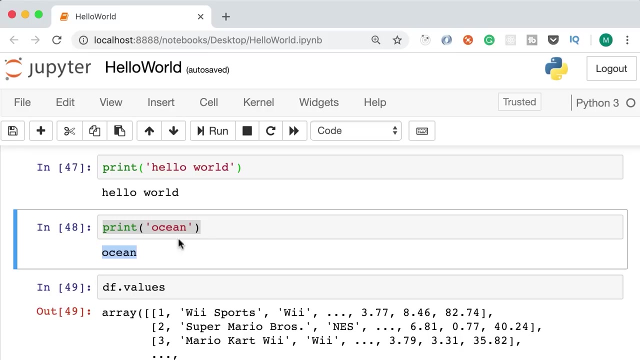 for each cell. That is why it's different from a regular pi file where we only have the source code. Here we also have auto completion and intellisense. so in the cell let's call df, data frame dot. now if you press tab you can see that it will. 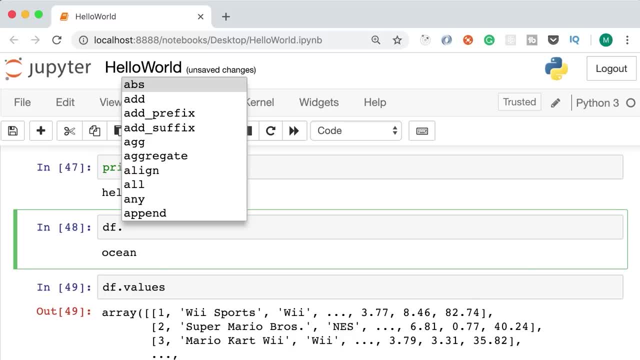 see all the attributes and methods in this object. So let's call describe. now with the cursor on the name of the method, we can press shift and tab to see this tooltip that describes what this method does and what parameter it takes. 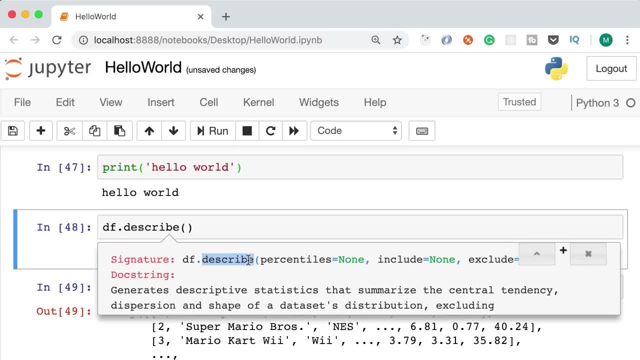 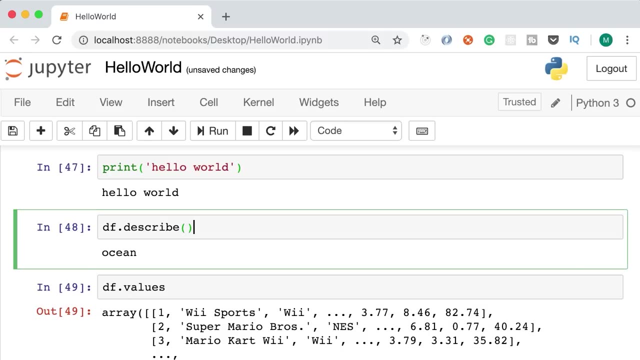 So here in front of signature you can see the describe method. these are the parameters and their default value, and right below that you can see the description of what this method does. In this case it generates descriptive statistics that summarizes the central tendency and so on. Similar to VS code, we can also convert a line. 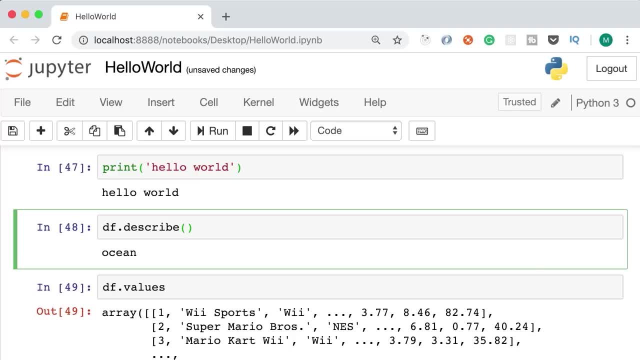 to comment by pressing command and slash on mac or control slash on windows, like this: Now this line is a comment, we can press the same shortcut one more time to remove the comment. So these were some of the most useful shortcuts in Jupyter. 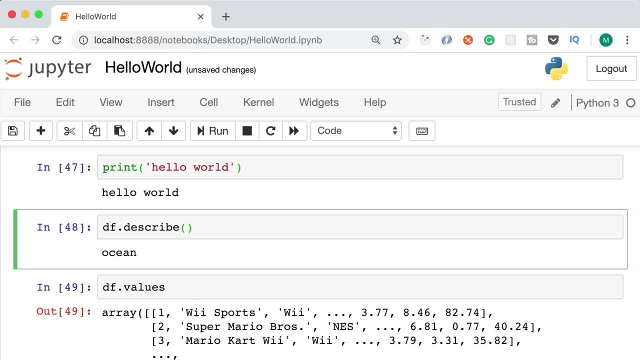 Now, over the next few lectures, we're going to work on a real machine learning project. But before we get there, let's delete all the cells here, so we start with only a single empty cell. So here in this cell first, I'm going to press the escape button. now the cell is blue, so we're 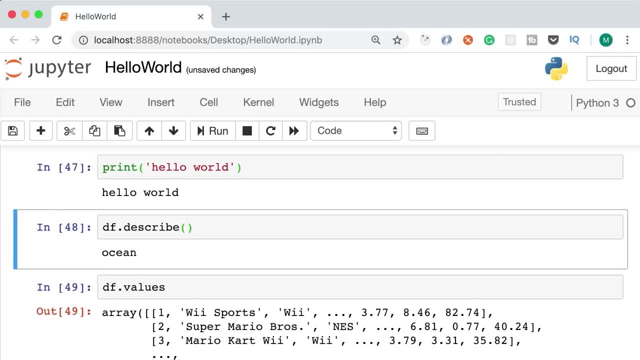 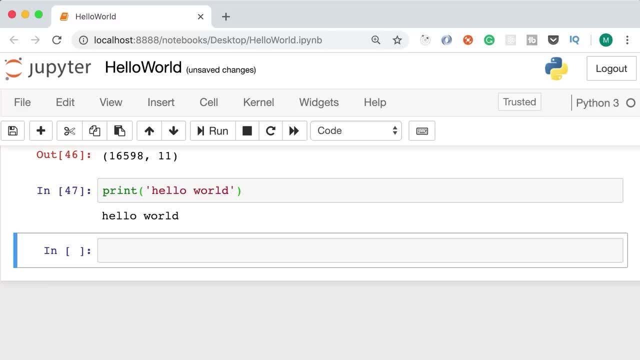 in the command mode, and we can delete the cell by pressing d twice. There you go. now the next cell is activated and it's in the command mode, so let's delete this as well. We have two more cells to delete. there you go, and the last one like this: 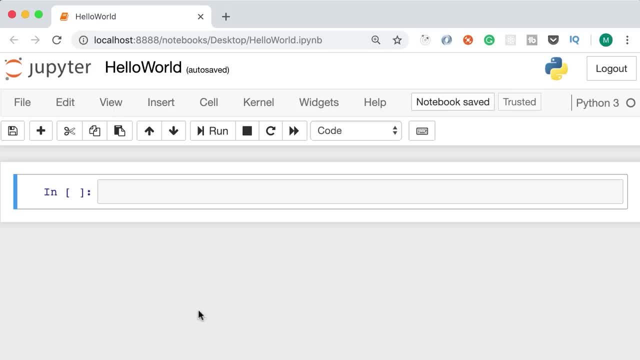 So now we have the project and we can delete the next one and the last one. like this, We have an empty notebook with a single cell. Hey guys, I just wanted to let you know that I have an online coding school at codewithmoshcom. 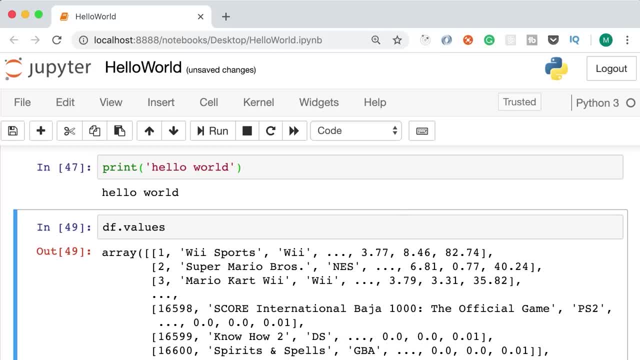 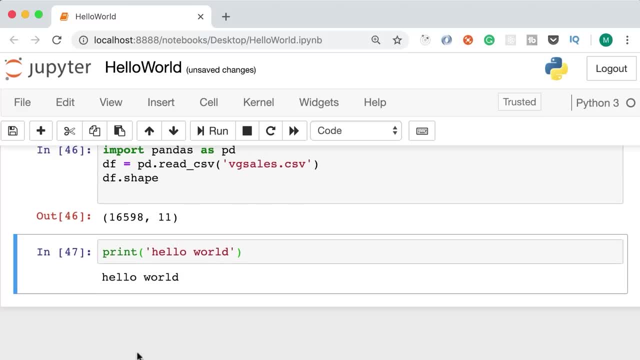 D twice. There you go. now the next cell is activated and it's in the command mode, so let's delete this as well. We have two more cells to delete. there you go, and the last one like this: So now we have an empty notebook. 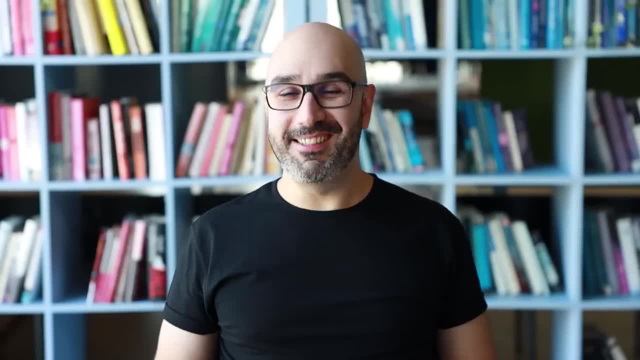 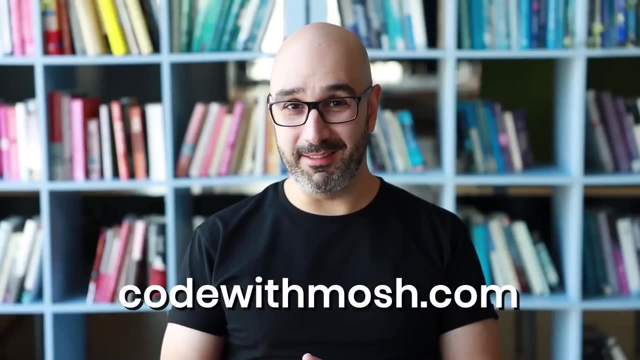 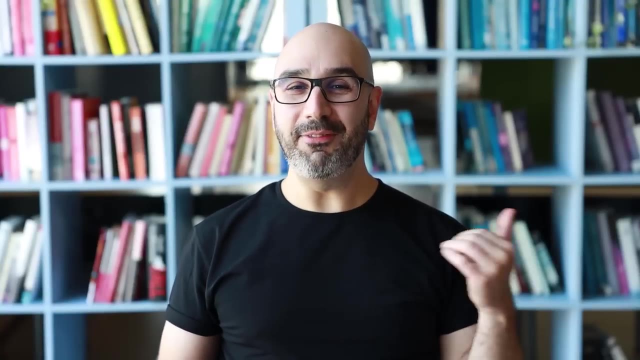 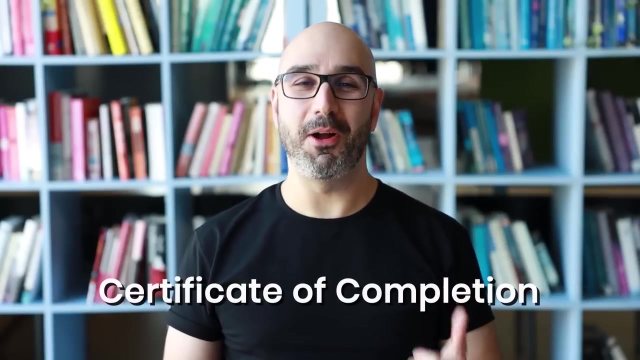 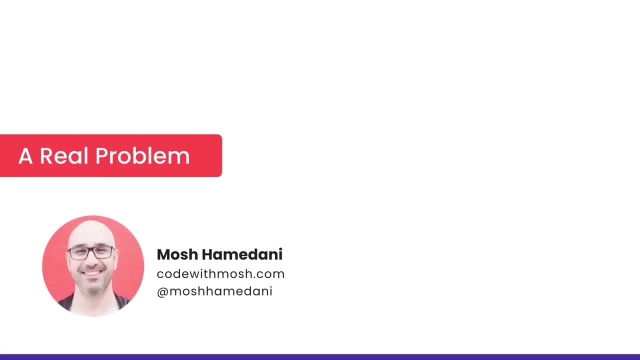 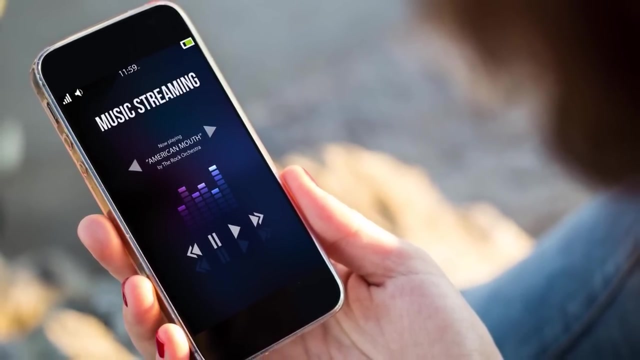 with a single cell. So that's it for this video. I hope you enjoyed it and I'll see you in the next one. Bye machine learning project. Imagine we have an online music store. When our users sign up, we ask their age and gender and, based on their 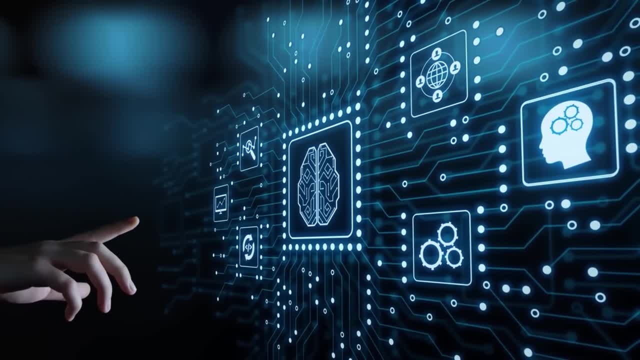 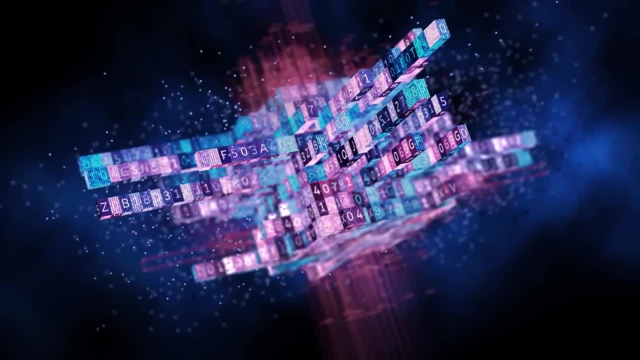 profile, we recommend various music albums they're likely to buy. So in this project we want to use machine learning to increase sales. So we want to build a model. we feed this model with some sample data based on the existing users. Our model will learn. 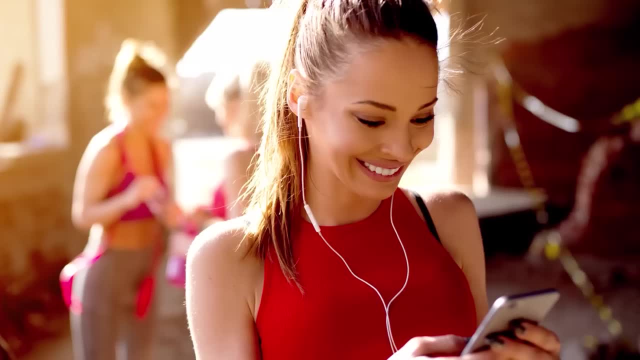 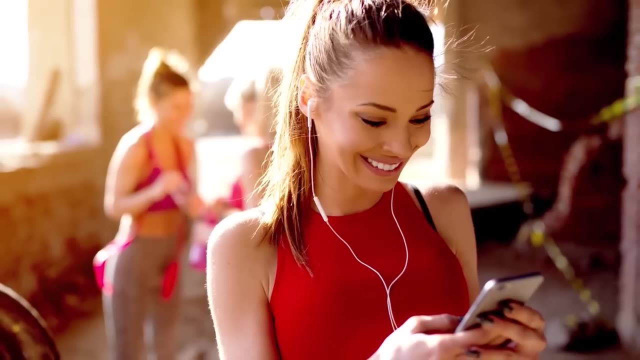 the patterns in our data so we can ask it to make predictions. When a new user signs up, we tell our model: hey, we have a new user with this profile. what is the kind of music that this user is interested in? Our model will say jazz or hip hop or whatever. 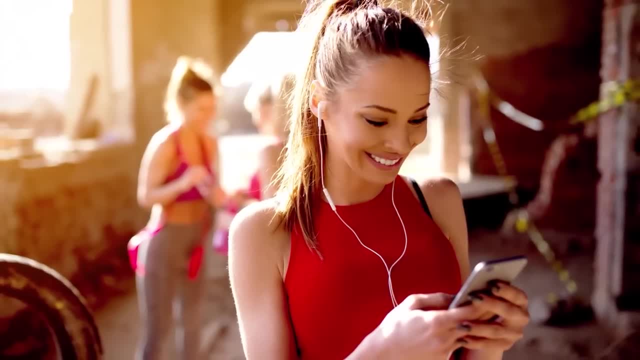 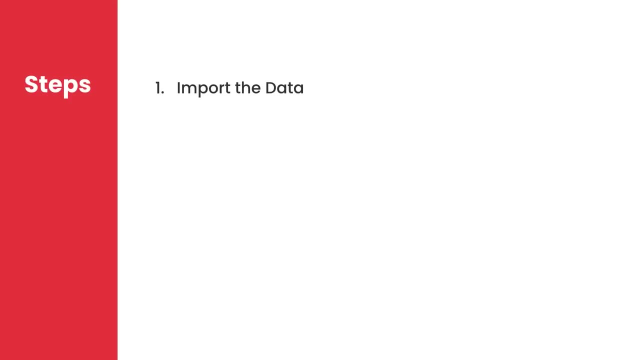 And based on that we can make suggestions to the user. So this is the problem we're going to solve. Now back to the list of steps in a machine learning project. First we need to import our data. then we should prepare or clean it. next we select a machine learning algorithm to build a model. 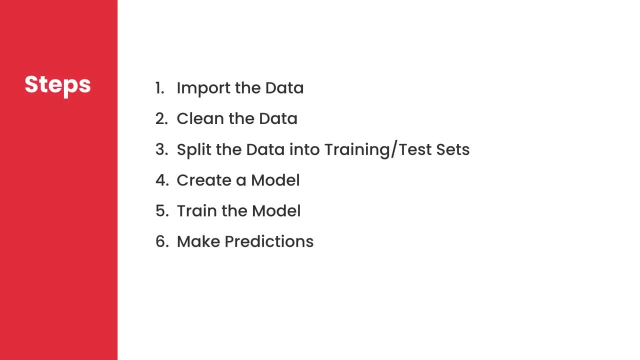 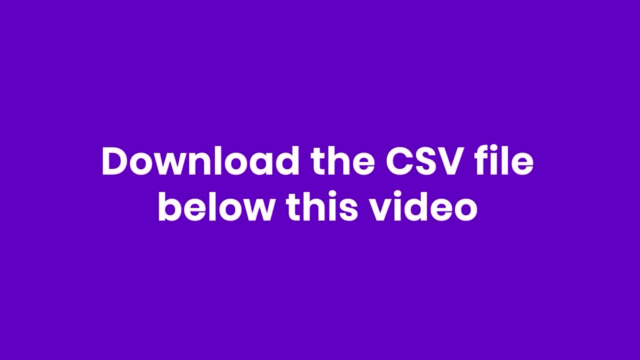 we train our model and ask it to make predictions, and finally, we evaluate our algorithm to see its accuracy. If it's not accurate, we either fine tune our model or select a different algorithm. So let's focus on the first step. Download the CSV file below this video. This is a very basic 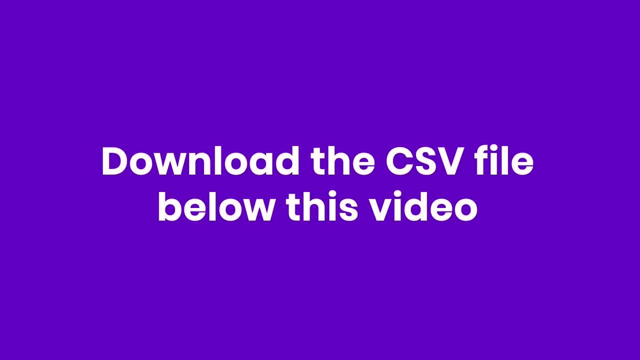 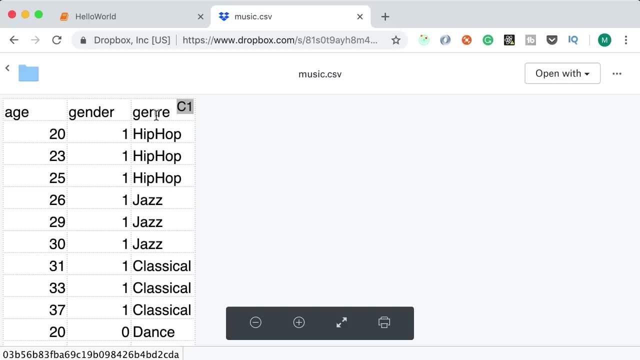 CSV that I've created for this project. It's just some random made up data. it's not real. So we have a table with three columns: age, gender and genre. Gender can either be one which represents a male, or zero, which represents a female. 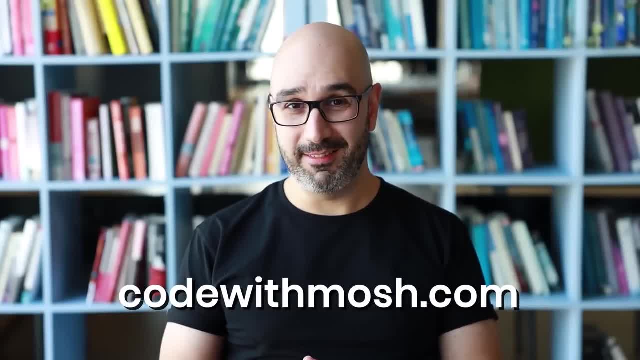 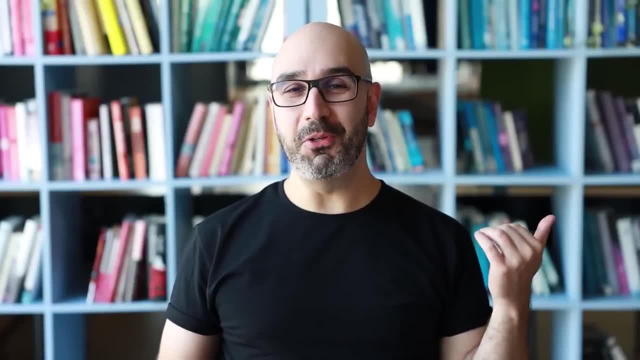 where you can find plenty of courses on web and mobile development. In fact, I have a comprehensive Python course that teaches you everything about Python, from the basics to more advanced concepts. So after you watch this tutorial, if you want to learn more, you may want to look at my Python course. it comes with a 30 day money back guarantee. 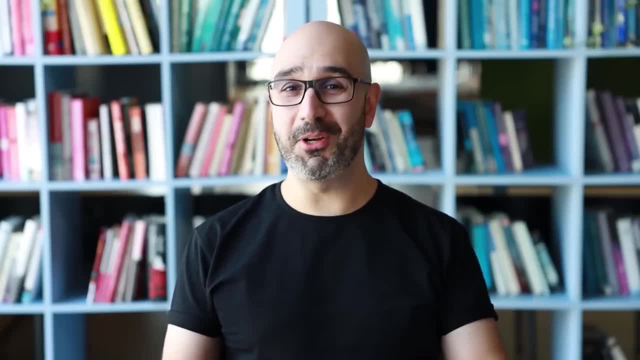 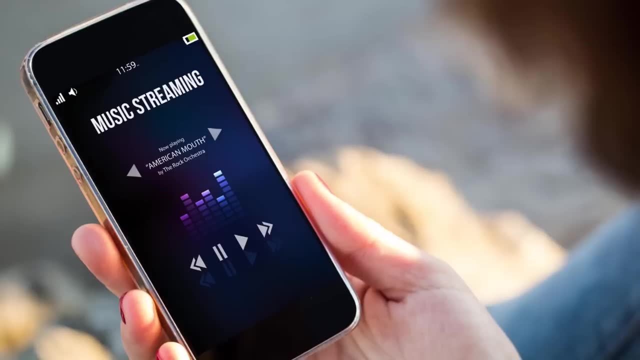 and a certificate of completion you can add to your resume. In case you're interested, the link is below this video. Over the next few lectures we're going to work on a real machine learning project. Imagine we have an online music store. 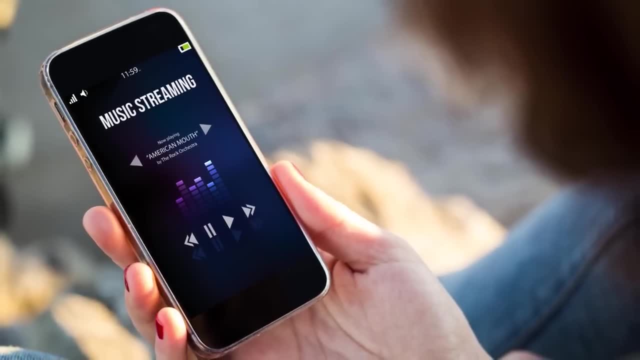 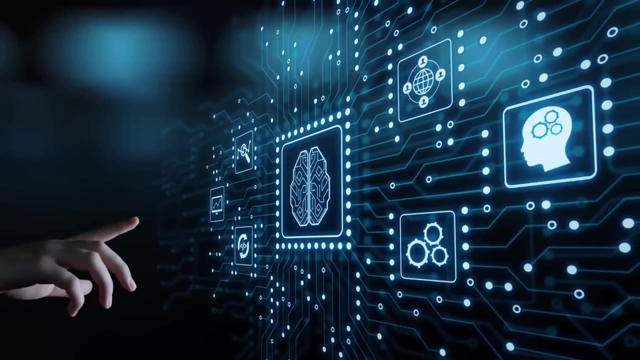 When our users sign up, we ask their age and gender and, based on their profile, we recommend various music albums they're likely to buy. So in this project we want to use machine learning to increase sales. So we want to build a model. we feed this model with some 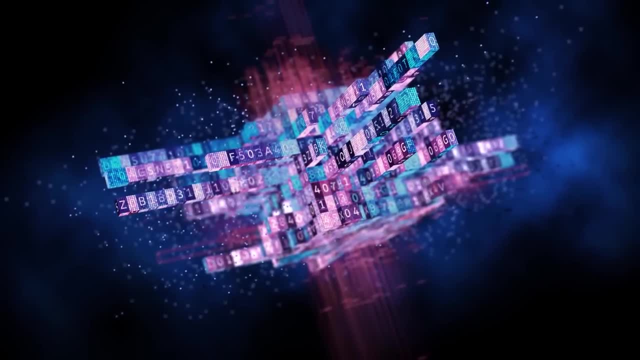 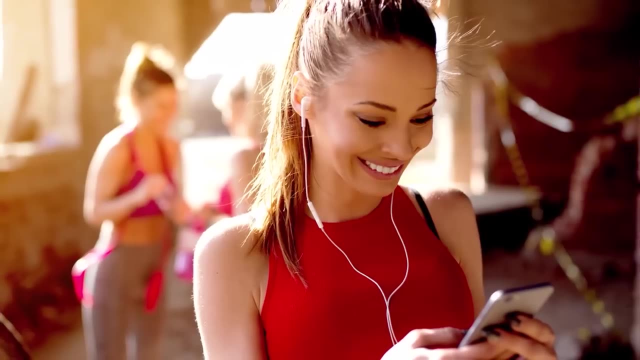 sample data based on the existing users. Our model will learn the patterns in our data so we can ask it to make predictions. When a new user signs up, we tell our model: hey, we have a new user with this profile. what is the kind of music that this user is interested in? 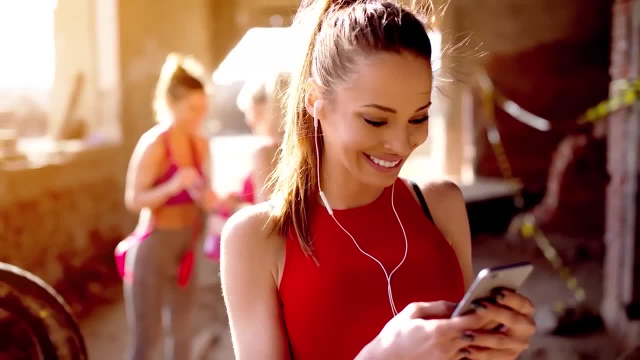 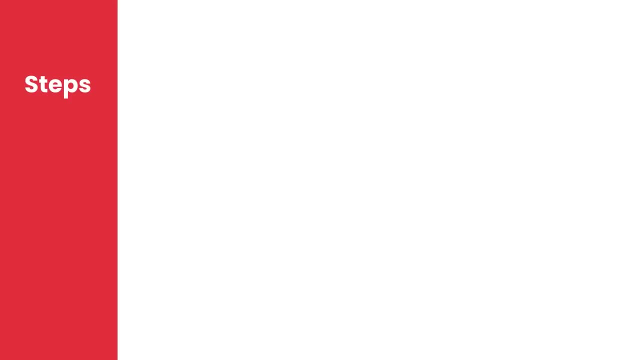 Our model will say jazz or hip hop or whatever, And based on that we can make suggestions to the user. So this is the problem we're going to solve. Now back to the list of steps in a machine learning project. First we need to. 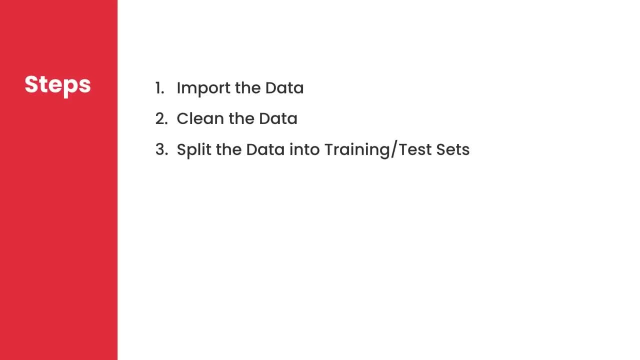 import our data, then we should prepare or clean it. next, we select a machine learning algorithm to build a model. we train our model and ask it to make predictions And finally, we evaluate our algorithm to see its accuracy. If it's not accurate, we either fine tune our model. 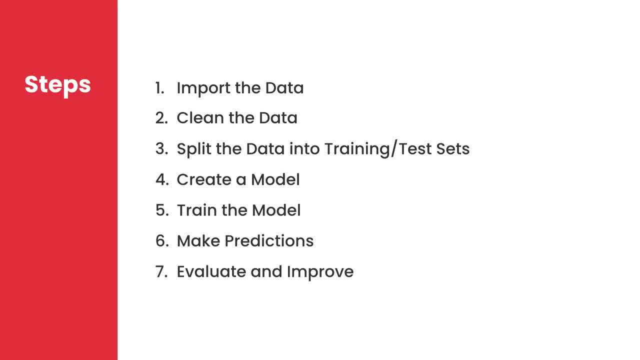 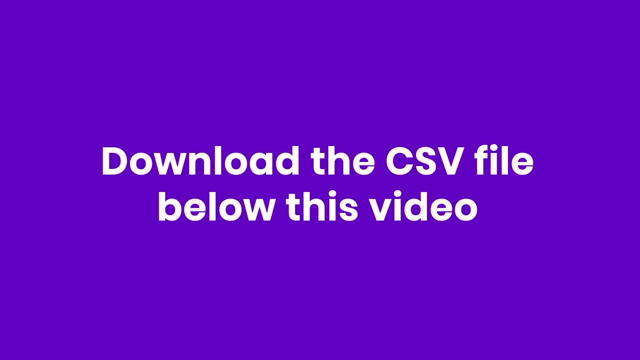 or select a different algorithm. So let's focus on the first step: Download the CSV file below this video. This is a very basic CSV that I've created for this project. It's just some random made up data. it's not real. 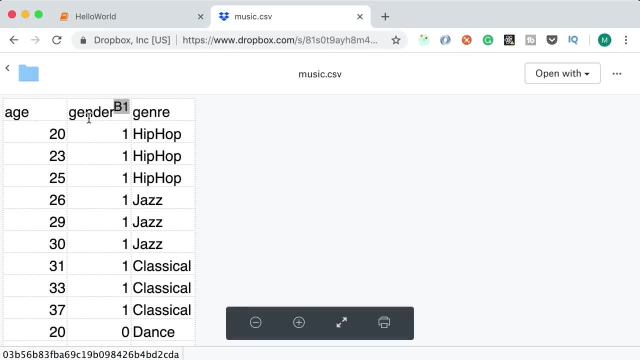 So we have a table with three columns: age, gender and genre. Gender can either be 1,, which represents a male, or 0,, which represents a female. Here I'm making a few assumptions. I'm assuming that men between 20 and 25 like hip hop. men between 26 and 30 like jazz, and after the age of 30, they like classical music. For women, I'm assuming that if they're between 20 and 25, they like dance music. if they're between 26 and 30, they like 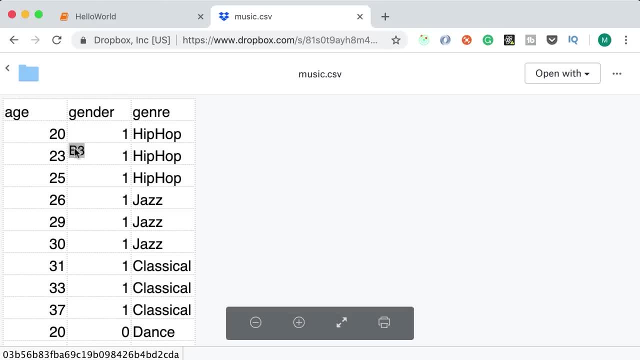 Here I'm making a few assumptions. I'm assuming that men between 20 and 25 like hip hop, men between 26 and 30 like jazz, and after the age of 30, they like classical music. For women, I'm assuming that if they're between 20 and 25, they like 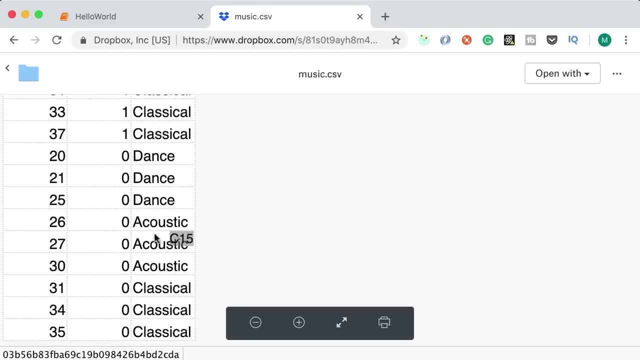 dance music. if they're between 26 and 30, they like acoustic music and, just like men, after the age of 30, they like classical music. Once again, this is a made up pattern. it's not the representation of the reality. 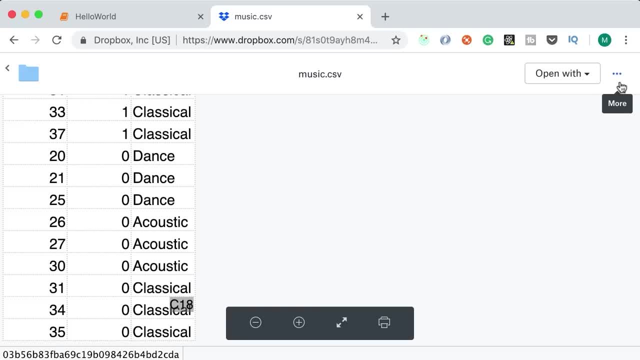 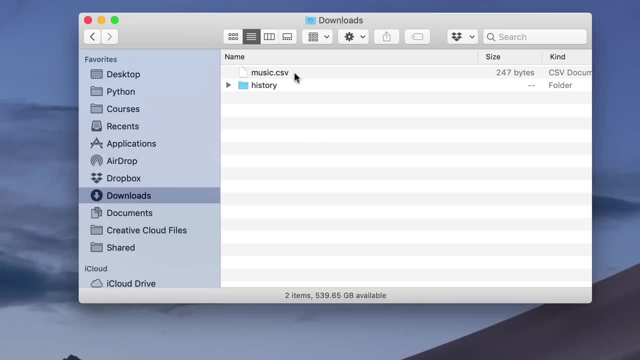 So let's go ahead and build our model And download the CSV. Click on this dot dot dot icon here and download this file. In my downloads folder here we have this musiccsv. I'm going to drag and drop this onto desktop because that's where I've stored. 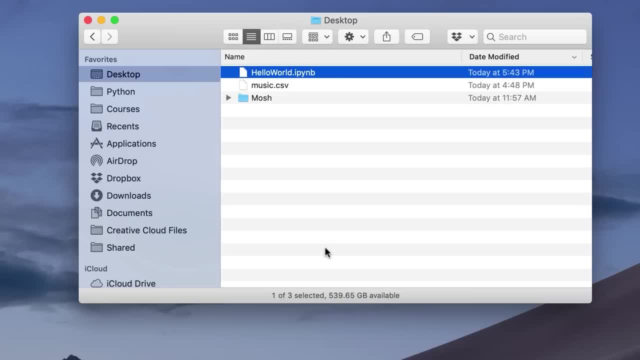 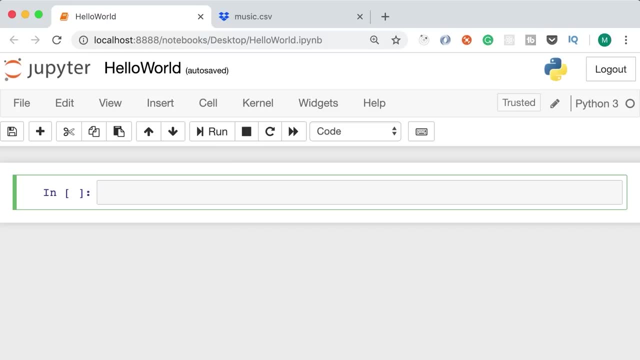 this hello world notebook. So I want you to put the CSV file right next to your Jupyter notebook. Now back to our notebook. you need to read the CSV file. So just like before, first we need to import the pandas module. so import pandas as. 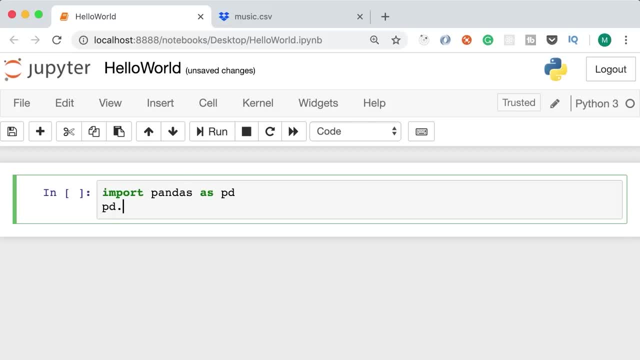 pd And then we'll call pd. that read underline csv, and the name of our file is music dot csv. As you saw earlier, this returns a data frame which is a two dimensional array similar to an Excel spreadsheet, So let's call that music underline data. 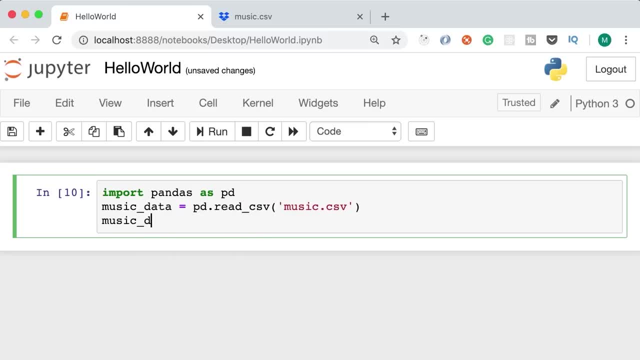 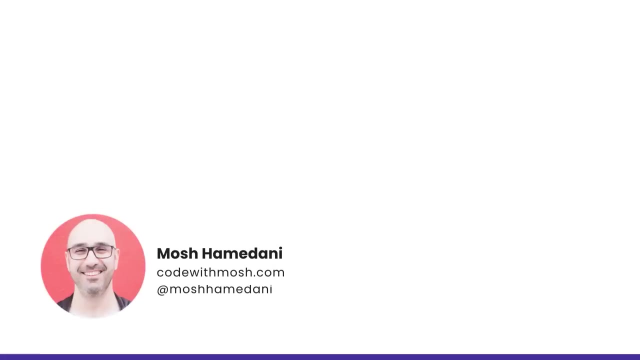 Now let's inspect this music underline data to make sure we loaded everything properly, So run. So here's our data frame, beautiful. Next we need to prepare or clean the data, And that's the topic for the next lecture. The second step in a machine learning project is cleaning or preparing. 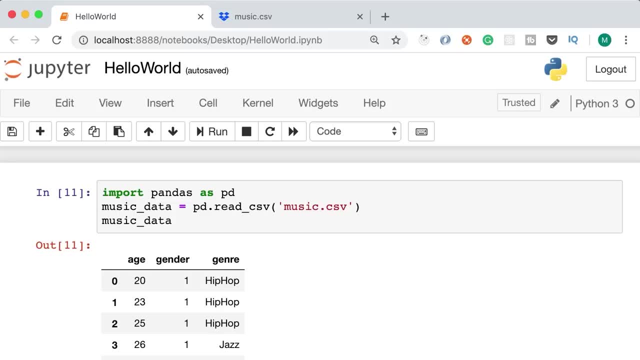 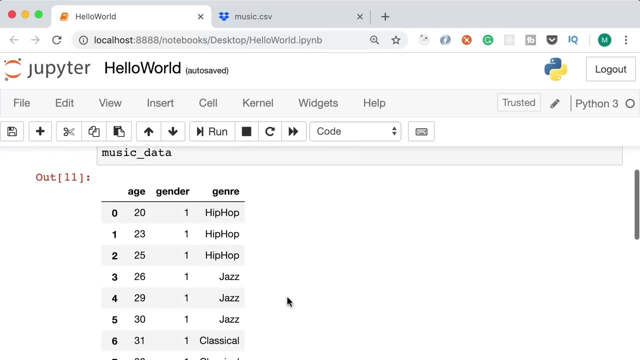 the data, And that involves tasks such as removing duplicates, null values and so on. Now, in this particular data set, we don't have to do any kind of cleaning because we don't have any duplicates And, as you can see, all rows have values for all columns. 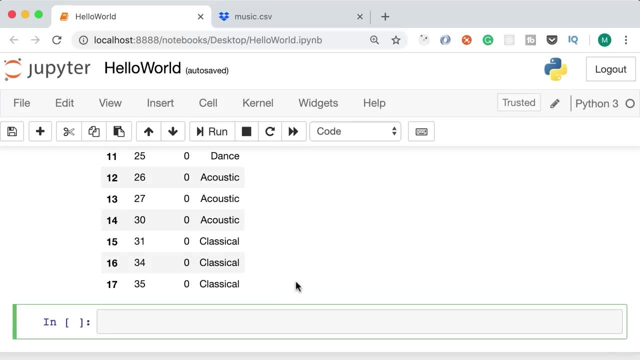 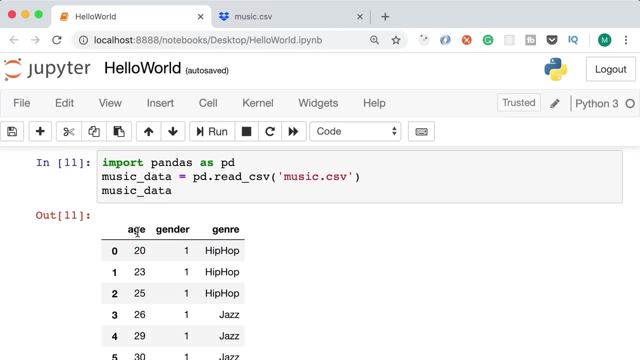 So we don't have null values. But there is one thing we need to do: We should split this data set into two separate data sets: One with the first two columns, which we refer to as the input set, and the other with the last column, which we refer to as the output set. 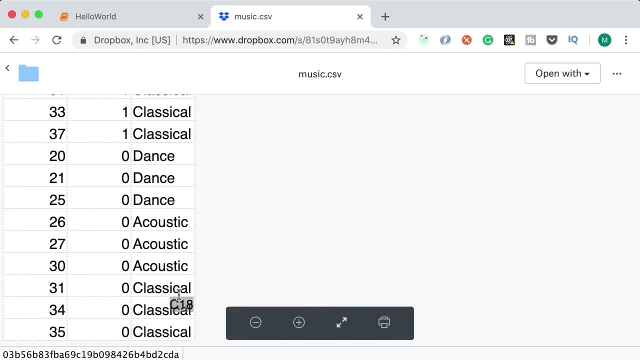 acoustic music and, just like men after the age of 30, they like classical music. Once again, this is a made up pattern. it's not the representation of the reality. So let's go ahead and download this CSV. Click on this dot dot dot icon here and download. 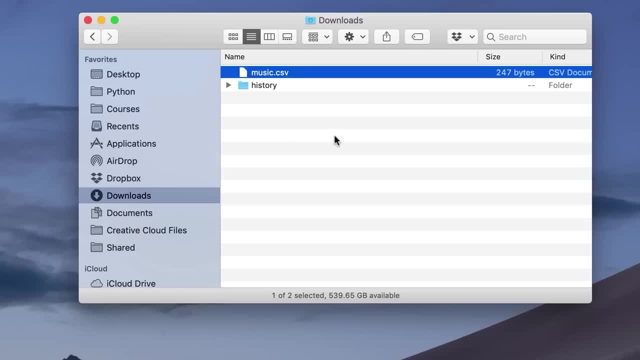 this file In my downloads folder. here we have this musiccsv. I'm going to drag and drop this onto the desktop because that's where I've stored this hello world notebook. So I want you to put the CSV file right next to your Jupyter notebook. 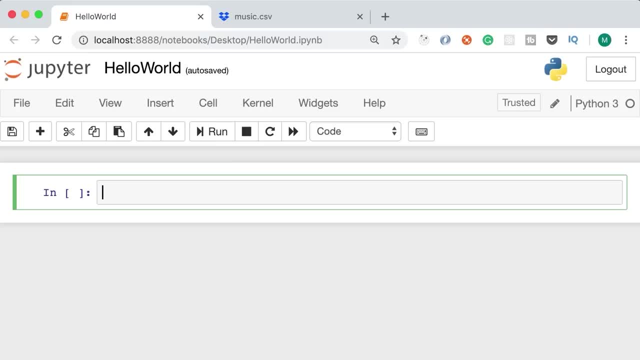 Now back to our notebook. we need to read the CSV file. So, just like before, first we need to import the pandas module. so import pandas as pd, And then we'll call pdread, analyze csv, and the name of our file is musiccsv. 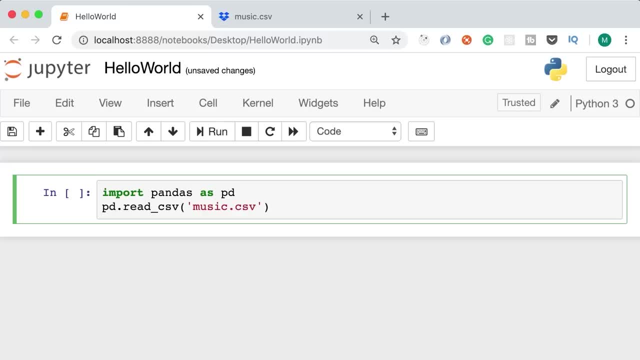 As you saw earlier, this returns the CSV file, A data frame which is a two dimensional array similar to an excel spreadsheet. So let's call that music underline data. Now let's inspect this music underline data to make sure we loaded everything properly. So 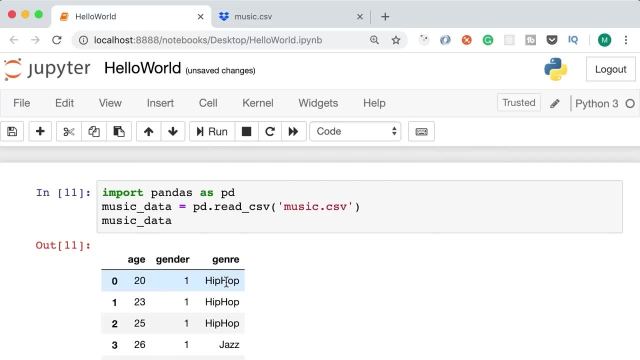 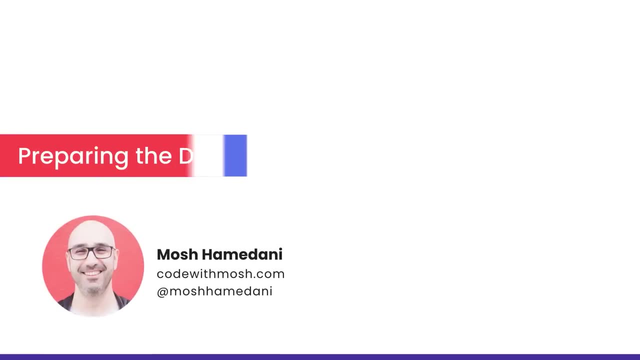 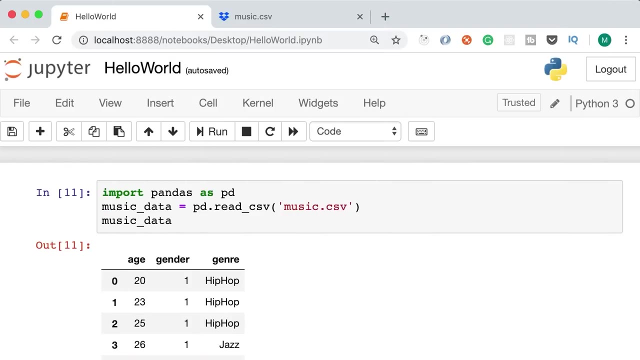 run. so here's our data frame, beautiful. next we need to prepare or clean the data, and that's the topic for the next lecture. The second step in a machine learning project is cleaning or preparing the data, And that involves tasks such as removing, 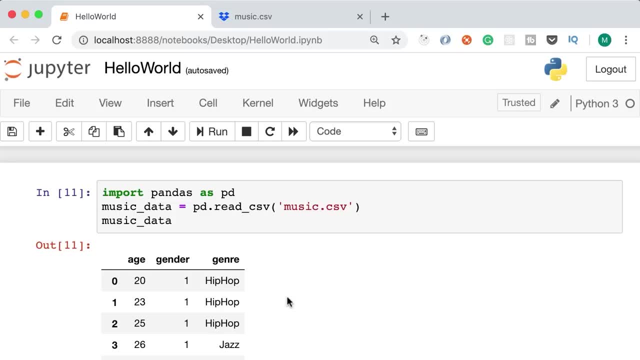 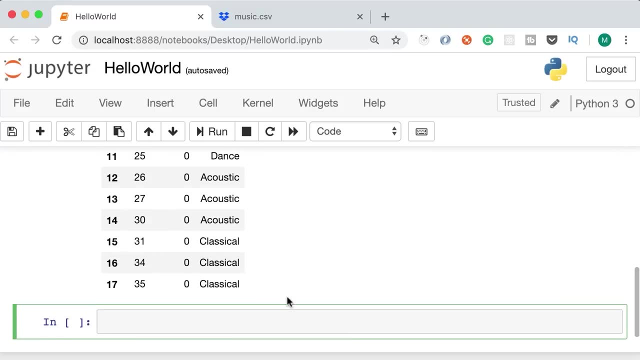 duplicates, null values and so on. Now, in this particular data set, we don't have to do any kind of cleaning because we don't have any duplicates and, as you can see, all rows have values for all columns, So we don't have null values. 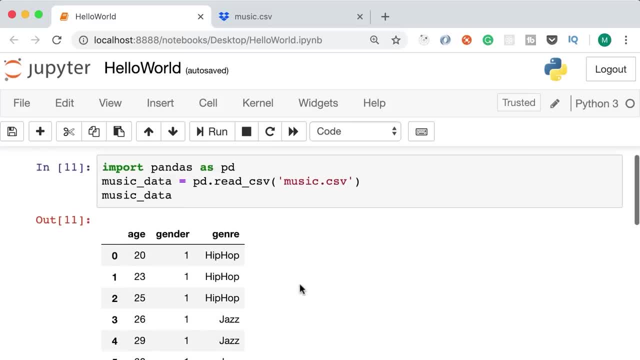 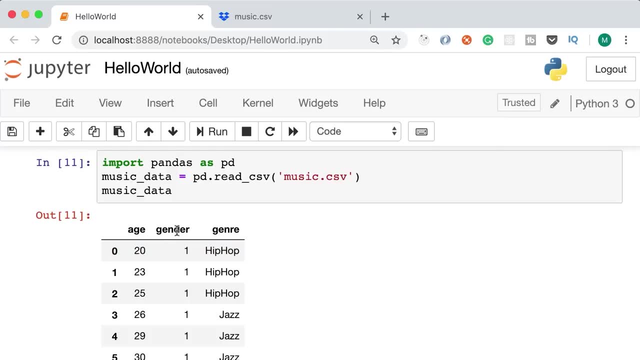 But there is one thing we need to do: We should split this data set into two separate data sets, One with the first two columns, which we refer to as the input set, and the other with the last column, which we refer to as the output set. So when we train, 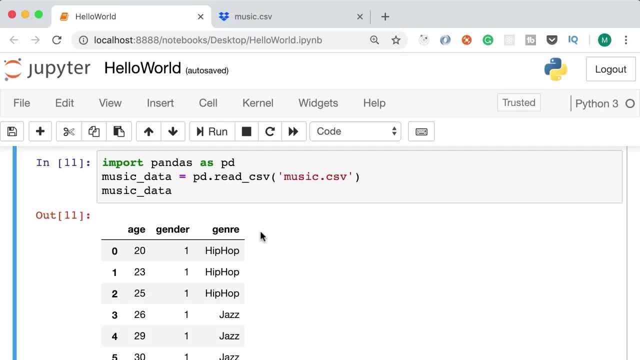 a model. we give it two separate data sets: the input set and the output set. The output set, which is, in this case, the genre column, contains the predictions. So we're telling our model that if we have a user who is 20 years old and is a male, 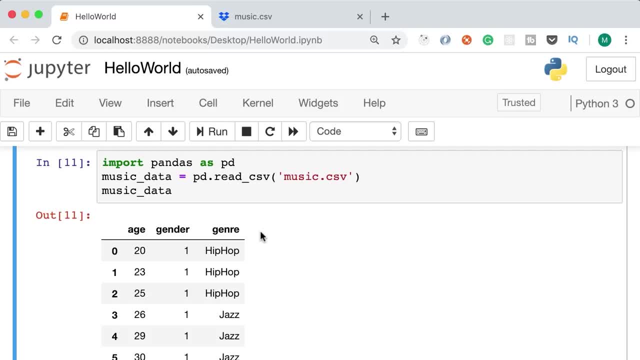 So when we train a model, we give it two separate data sets: The input set and the output set. The output set, which is in this case the genre column, contains the predictions. So we're telling our model that if we have a user who is 20 years old, 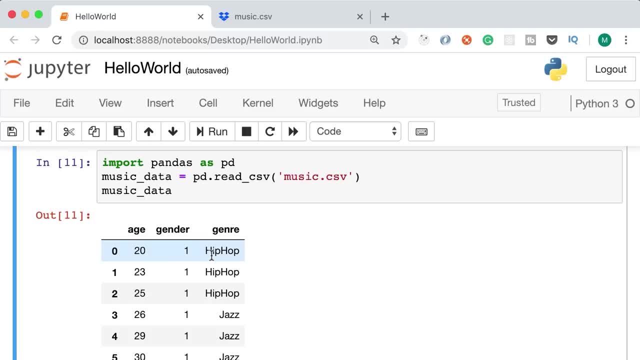 and is a male. they like hip hop. Once we train our model, then we give it a new input set. For example, we say: hey, we have a new user who is 21 years old and is a male. What is the genre of the music that this user probably likes? As you can see, 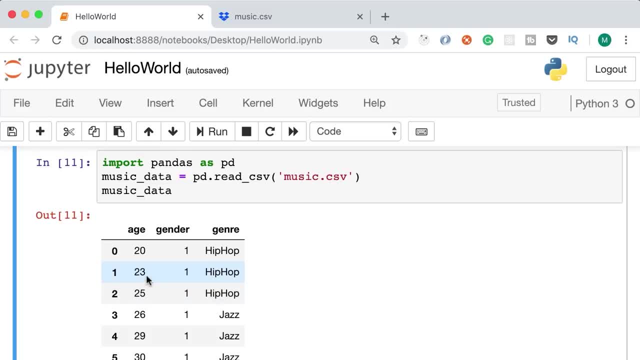 in our input set, we don't have a sample for a 21 year old male, So we're going to ask our model to predict that. That is the reason we need to split this data set into two separate sets: Input and output. So back to our code. 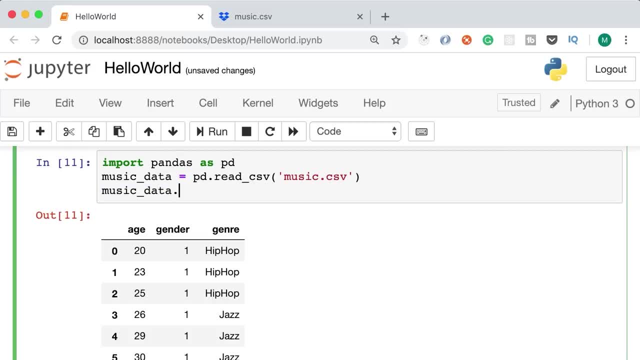 this data frame object has a method called drop. Now, if you put the cursor on the method name and press shift and tab, you can see this tool tip. so this is the signature of this drop method. these are the parameters that we can pass here. The parameter we're going to use in this lecture is columns. 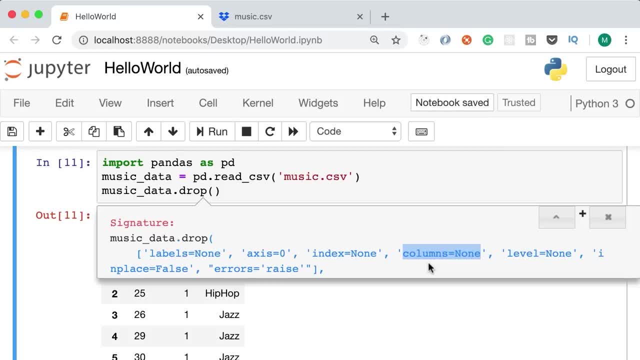 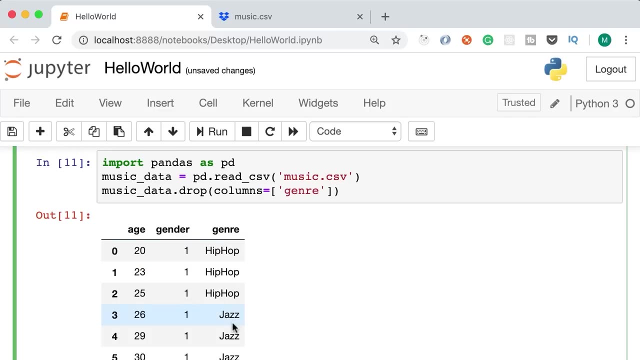 which is set to none by default. With this parameter, we can specify the columns we want to drop. So in this case we set columns to an array with one string genre. Now, this method doesn't actually modify the original data set. in fact, it will create a new data set. 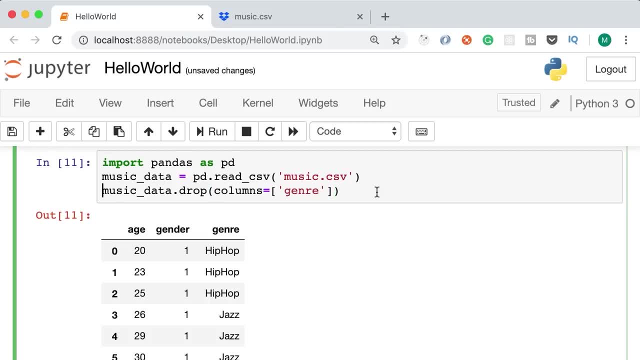 but without this column. So by convention we use a capital X to represent that data set. So capital X equals this expression. Now let's inspect x. so, as you can see, our input set, or x, includes these two columns: age and gender. 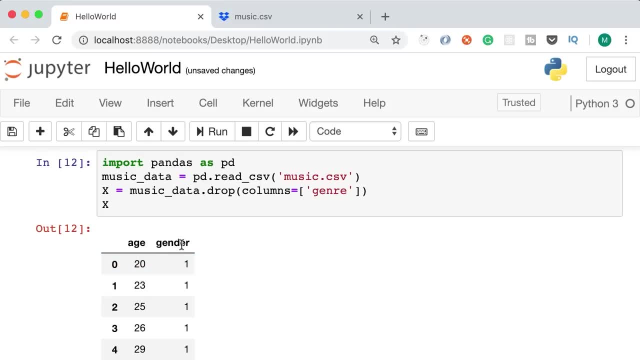 It doesn't have the output or predictions. Next, we need to create our output set. So once again, we start with our data frame: music data. using square brackets, we can get all the values in a given column In this case. 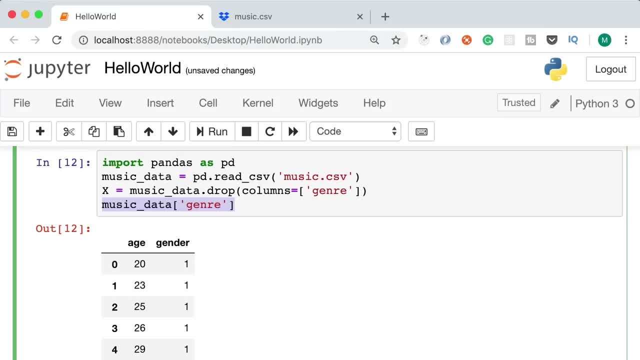 genre. Once again, this returns a new data set. by convention we use a lower case y to represent that. So that is our output data set. Let's inspect that as well. so in this data set we only have the predictions or the answers. So we have prepared our data. 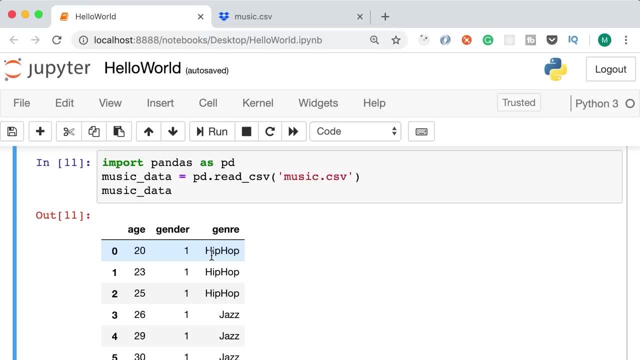 they like hip hop. Once we train our model, then we give it a new input set. For example, we say: hey, we have a new user who is 21 years old and is a male. What is the genre of the music that this user probably likes? 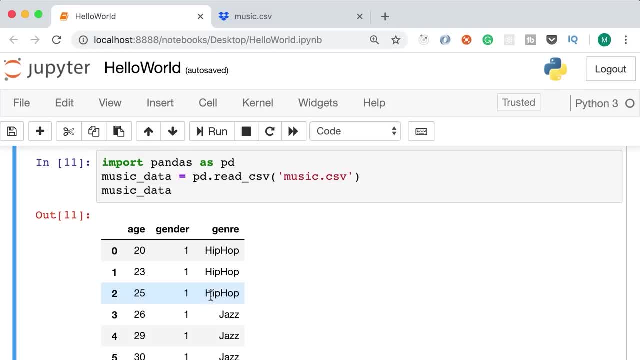 As you can see in our input set, we don't have a sample for a 21 year old male, So we're going to ask our model to predict that. That is the reason we need to split this data set into two separate sets. 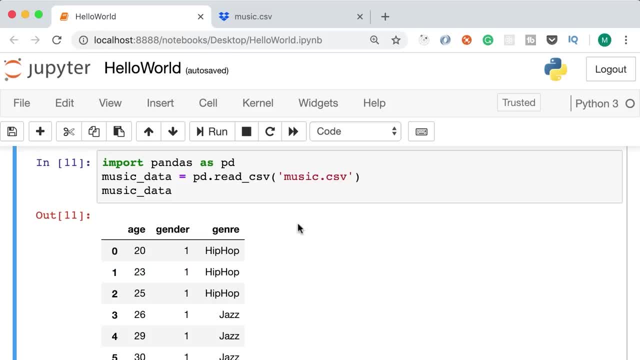 Input and output. So back to our code. this data frame object has a method called drop. Now if you put the cursor on the method name and press shift and tab, you can see this tooltip. so this is the signature of this drop method. 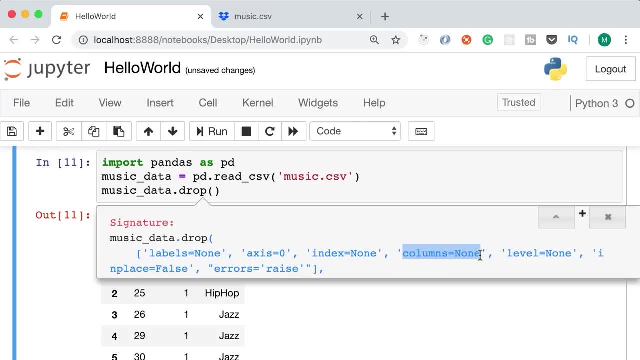 These are the parameters that we can pass here. The parameter we're going to use in this lecture is columns, which is set to none by default. With this parameter, we can specify the columns we want to drop. So in this case, we set columns to an array. 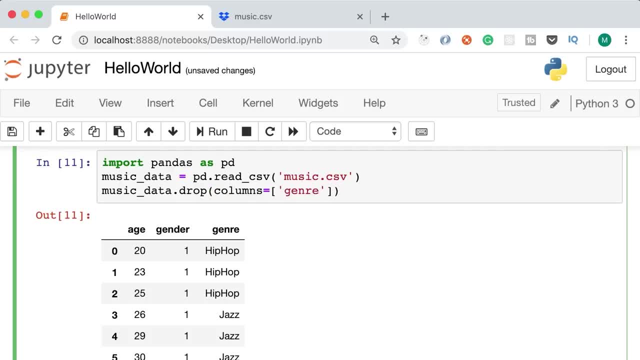 with one string genre. Now this method doesn't actually modify the original data set. in fact it will create a new data set, but without this column. So by convention we use a capital X to represent that data set. So capital X equals this expression. 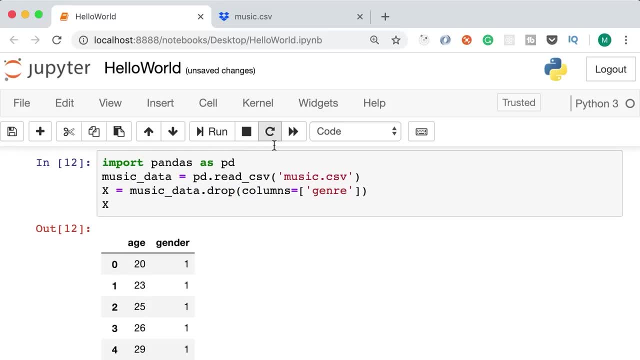 Now let's inspect x so, as you can see, our input set, or, x, includes these two columns: age and gender. It doesn't have the output or predictions. Next, we need to create our output set. So, once again, we start with our data frame. music data using square brackets. 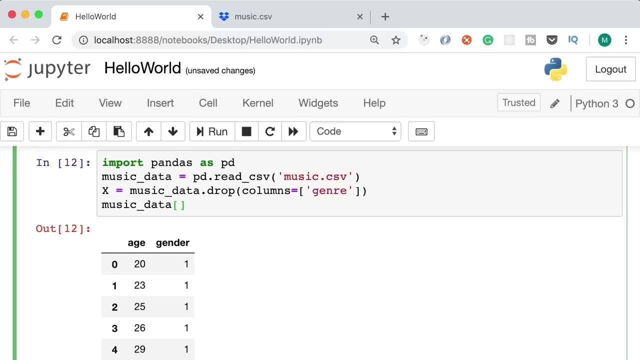 we can get all the values in a given column in this case genre. Once again, this returns a new data set. by convention, we use a lower case y to represent that. So that is our output data set. Let's inspect that as well. 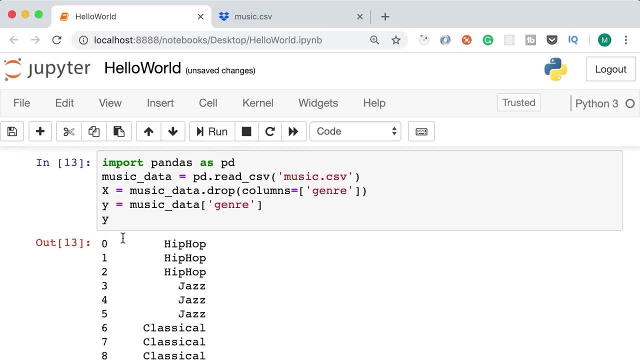 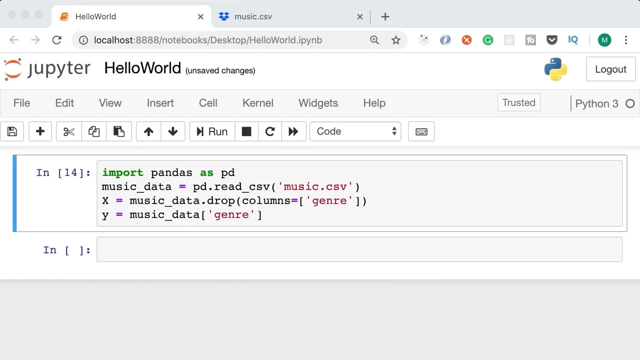 So in this data set we only have the predictions or the answers. So we have prepared our data. next we need to create a model using an algorithm. The next step is to build a model using a machine learning algorithm. There's so many algorithms out there and each algorithm has its pros. 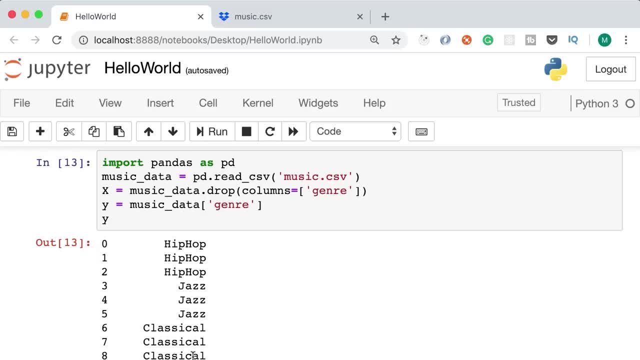 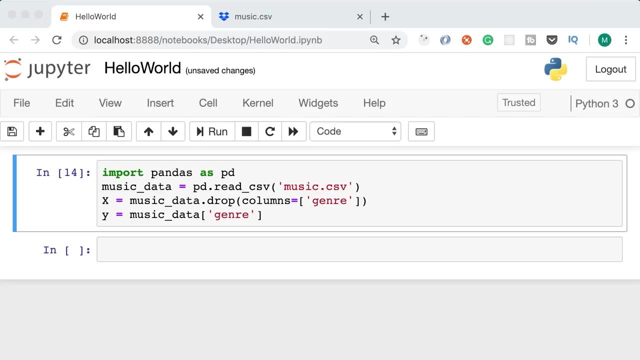 next, we need to create a model using an algorithm. The next step is to build a model using a machine learning algorithm. There's so many algorithms out there and each algorithm has its pros and cons in terms of the performance and accuracy. In this lecture, we're going to use a very simple algorithm called 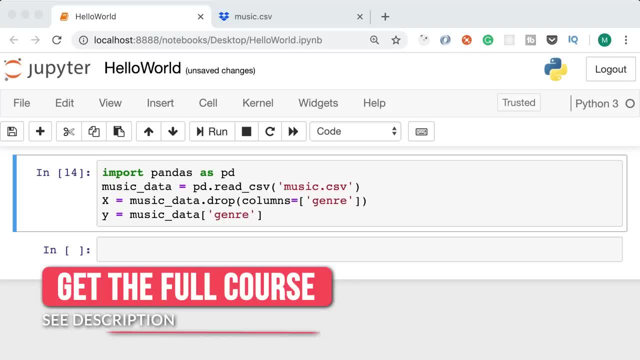 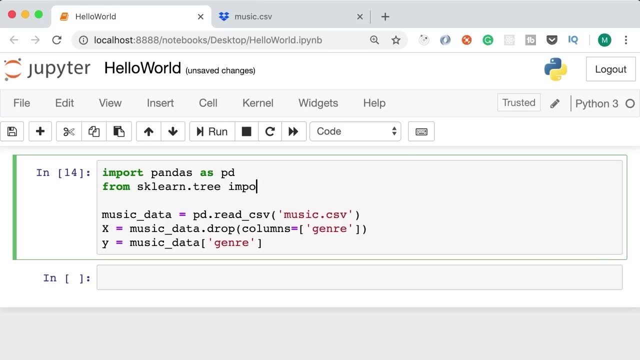 decision tree. Now, the good news is that we don't have to explicitly program these algorithms. they're already implemented for us in a library called scikit. learn So here, on the top from sklearntree. let's import the decision tree. 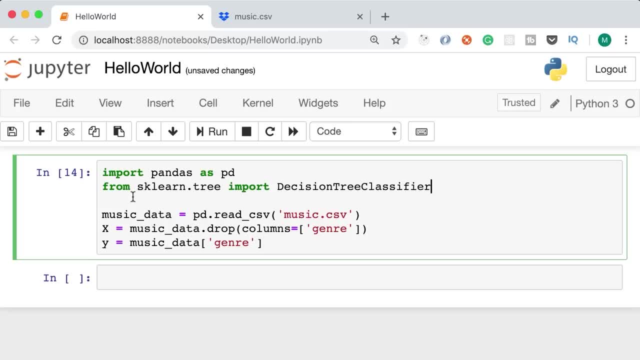 classifier. So sklearn is the package that comes with scikit learn library. this is the most popular machine learning library in python. In this package we have a module called tree and in this module we have a class called decision tree classifier. This class implements the decision tree algorithm. 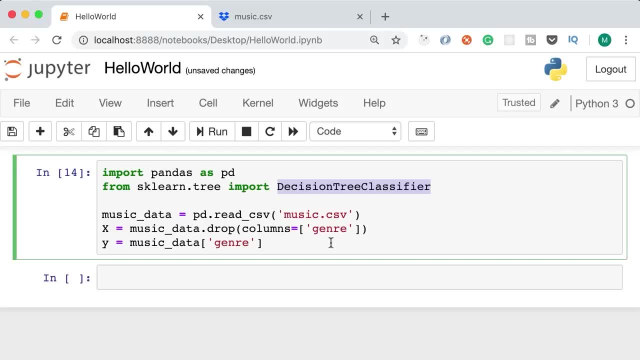 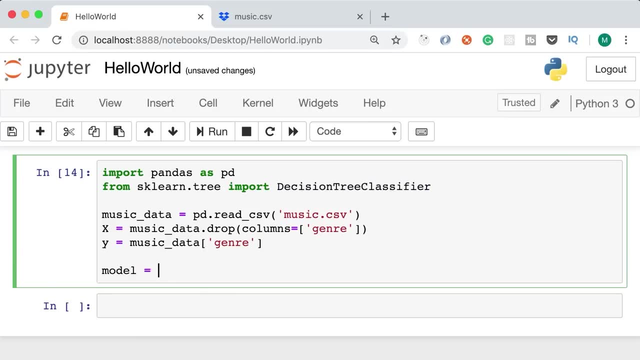 Okay, So now we need to create a new instance of this class. So at the end, let's create an object called model and set it to a new instance of decision tree classifier Like this: So now we have a model. next we need to train it so it learns patterns in the data. 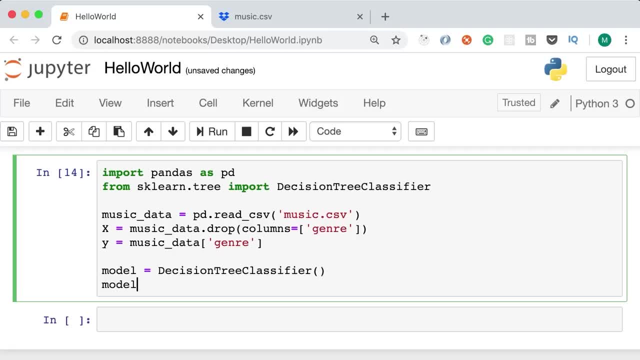 And that is pretty easy. We call modelfit. this method takes two data sets, the input set and the output set. So they are capital: x and y. Now, finally, we need to ask our model to make a prediction. So we can ask it: what is the kind of music? 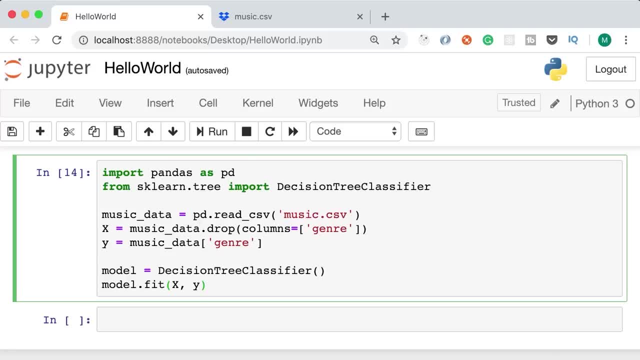 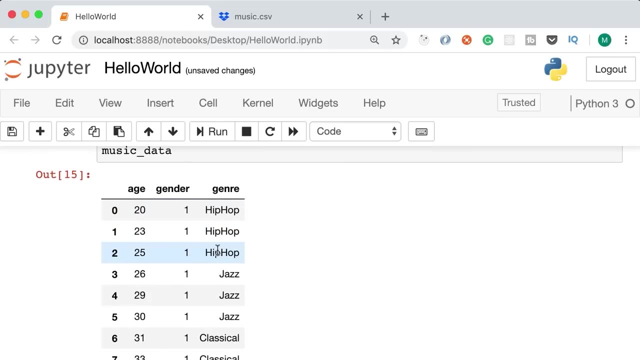 that a 21 year old male likes. Now, before we do that, let's temporarily inspect our initial data set, that is, music data. So look what we got here. As I told you earlier, I've assumed that men between 20 and 25 like hip hop music, But here we only have 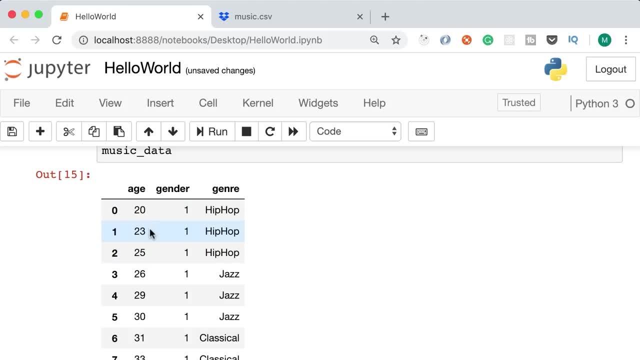 three samples for men aged 20,, 23, and 25.. We don't have a sample for a 21 year old male, So if you ask our model to predict the kind of music that a 21 year old male likes, we expect. 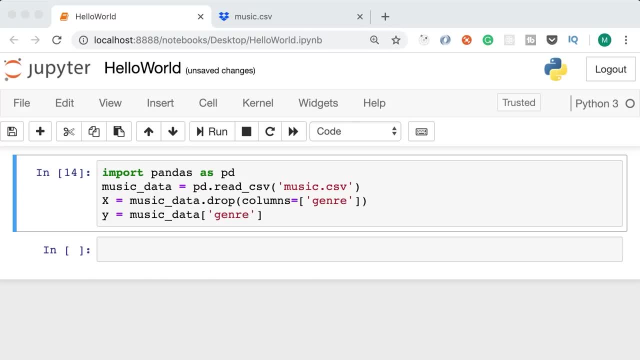 and cons in terms of the performance and accuracy. In this lecture, we're going to use a very simple algorithm called decision tree. Now, the good news is that we don't have to explicitly program these algorithms. They're already implemented for us in a library called scikit learn. 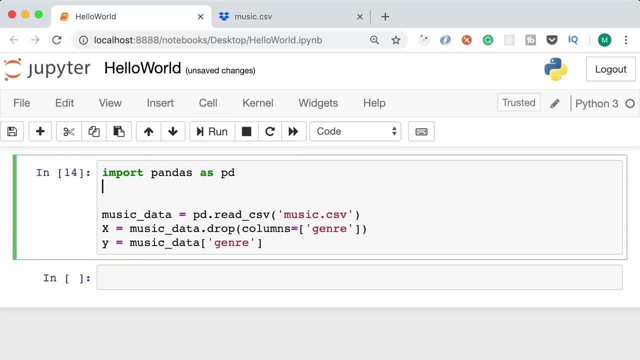 So here on the top from sklearntree, let's import the decision tree classifier. So sklearn is the package that comes with scikit learn library. this is the most popular machine learning library in python. In this package we have a module called tree and in this module 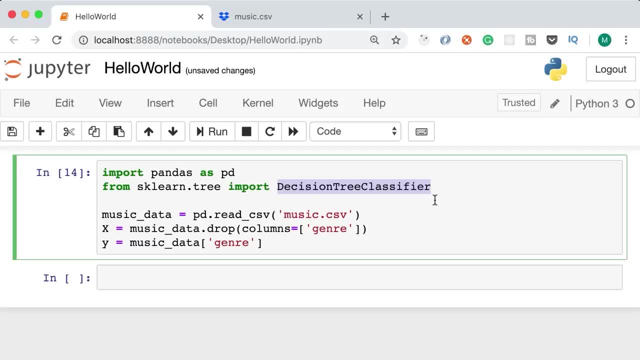 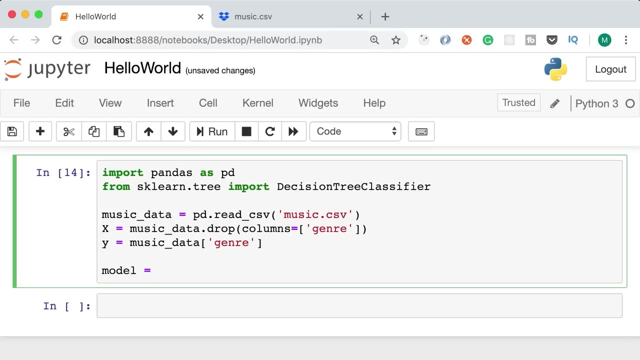 we have a class called decision tree classifier. This class implements the decision tree algorithm. Okay, So now we need to create a new instance of this class. So at the end, let's create an object called model and set it to a new instance of decision tree. 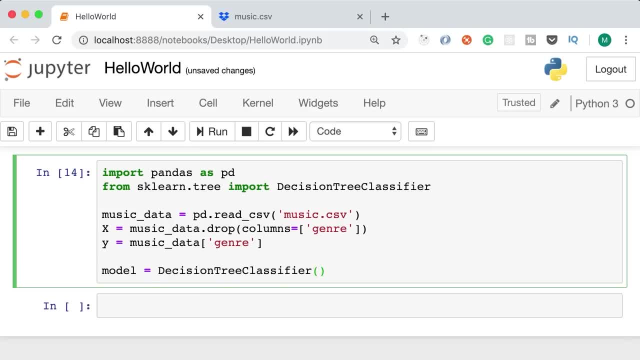 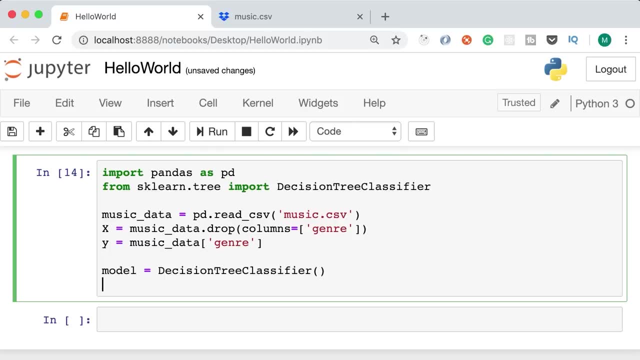 classifier Like this. So now we have a model. next we need to train it so it learns patterns in the data, And that is pretty easy. We call model that fit. this method takes two data sets: the input set and the output set. So they are. 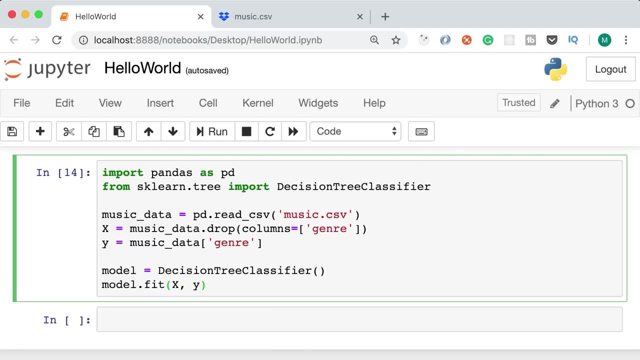 capital X and Y. Now, finally, we need to ask our model to make a prediction, So we can ask it: what is the kind of music that a 21 year old male likes? Now, before we do that, let's temporarily inspect our initial data set, that is, music data. 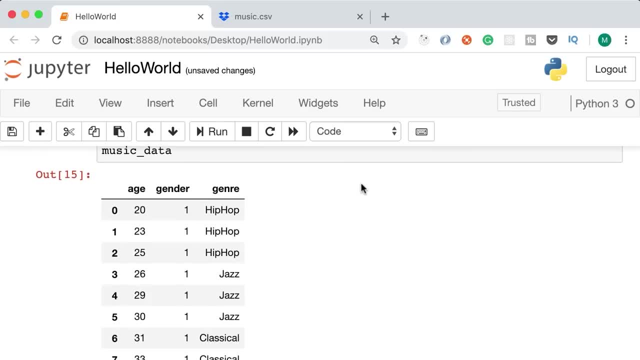 So look what we got here. As I told you earlier, I've assumed that men between 20 and 25 like hip hop music, but here we only have three samples for men aged 20,, 23, and 25.. We don't have a sample. 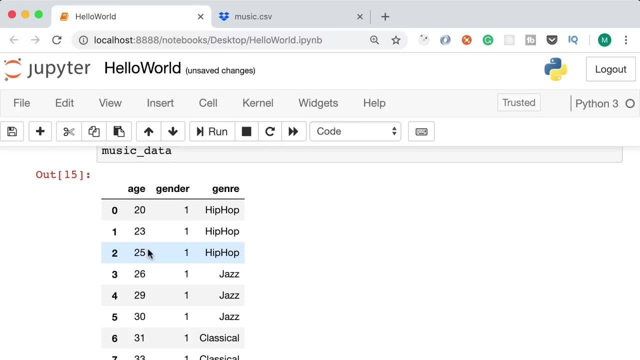 for a 21 year old male. So if you ask our model to predict the kind of music that a 21 year old male likes, we expect it to say hip hop. Similarly, I've assumed that women between 20 and 25 like dance music, but we don't have a sample for a 22 year old female. 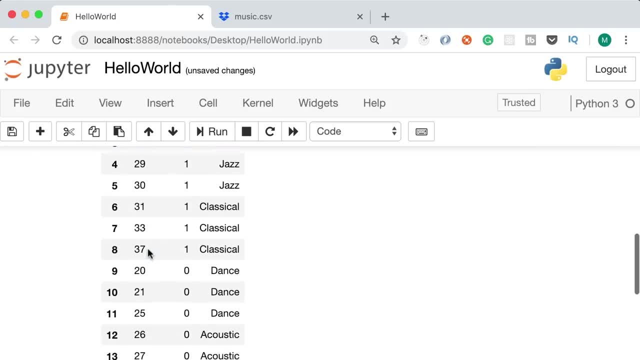 it to say hip hop. Similarly, I've assumed that women between 20 and 25 like dance music, but we don't have a sample for a 22 year old female. So, once again, if you ask our model to predict the kind of music that a 22 year old woman likes, we expect. 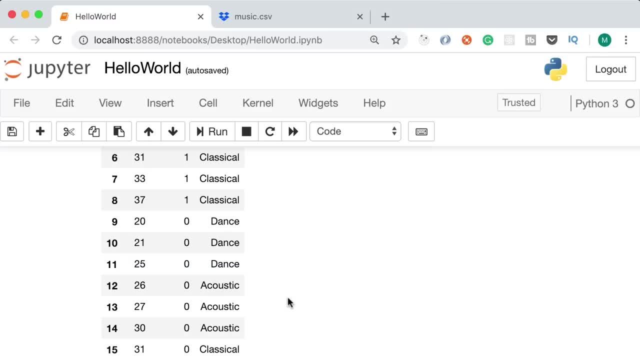 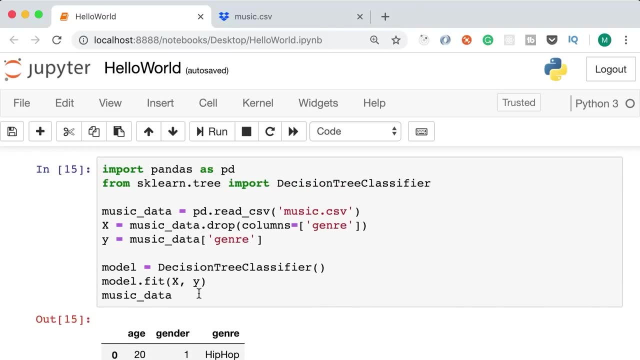 it to say dance. So with these assumptions, let's go ahead and ask our model to make predictions. So let's remove the last line and instead we're going to call modelpredict. This method takes a two dimensional array, So 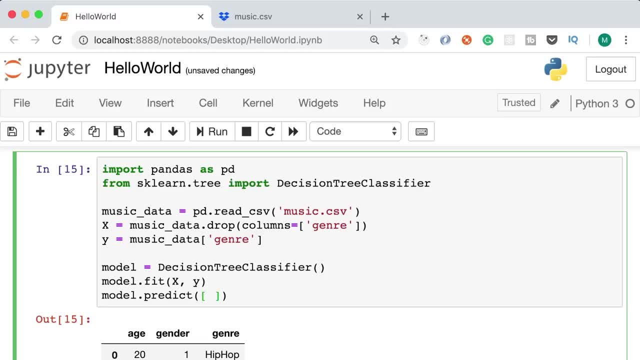 here's the outer array. in this array each element is an array, So I'm going to pass another array here and in this array I'm going to pass a new input set: A 21 year old male, So 21,. 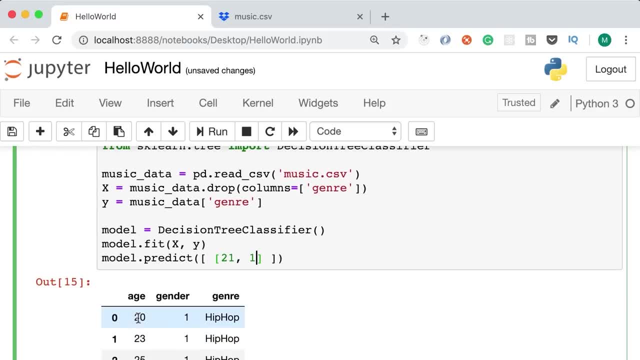 1.. That is like a new record in this table. Okay, So this is one input set. let's pass another input set for a 22 year old female. So here's another array. here we add 22,, 0.. So we're asking our model. 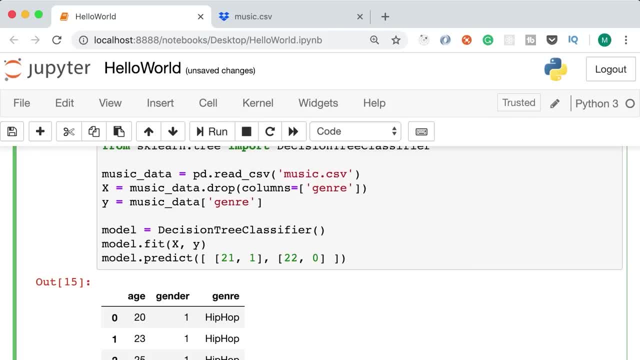 to make two predictions at the same time. We get the result and store it in a variable called predictions. and finally let's inspect that in our notebook Run. look what we got. Our model is saying that a 21 year old male likes hip hop. 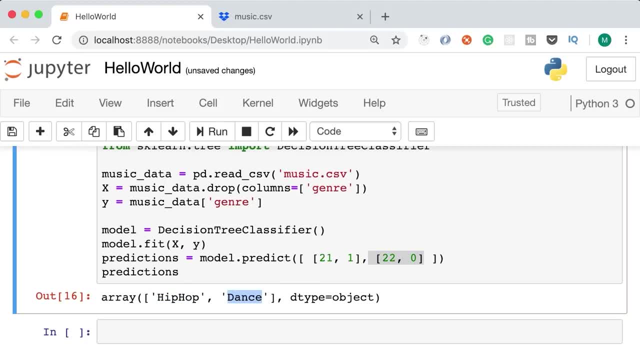 and a 22 year old female likes dance music. So our model could successfully make predictions here. beautiful, But wait a second. building a model that makes predictions accurately is not always that easy. As I told you earlier, after we build a model, we need to measure its accuracy. 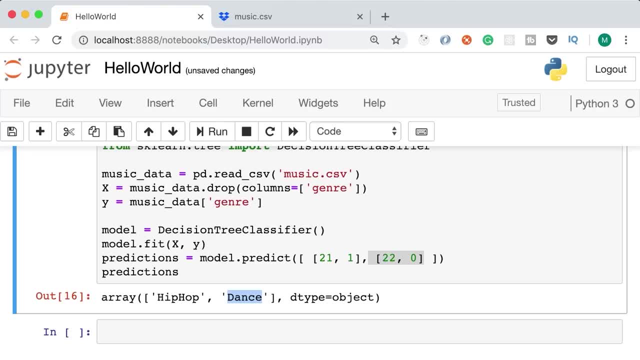 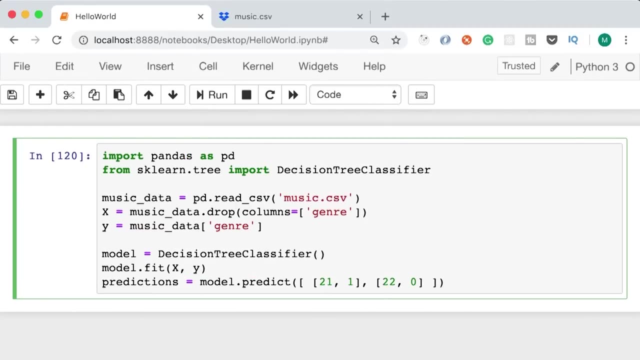 And if it's not accurate enough, we should either fine tune it or build a model using a different algorithm. So in the next lecture, I'm going to show you how to measure the accuracy of a model. In this lecture, I'm going to show you how to measure the accuracy of your models. 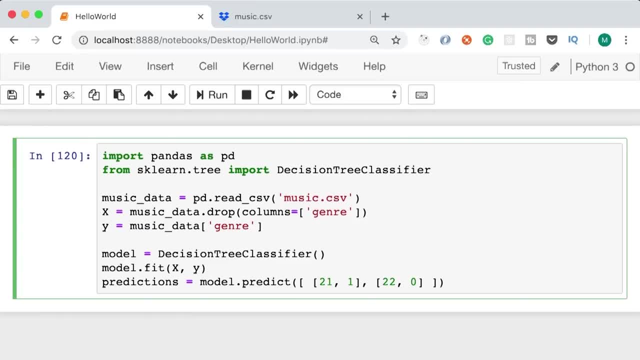 Now, in order to do so, first we need to split our data set into two sets, One for training and the other for training, Because right now we're passing the entire data set for training the model, and we're using two samples for making predictions. 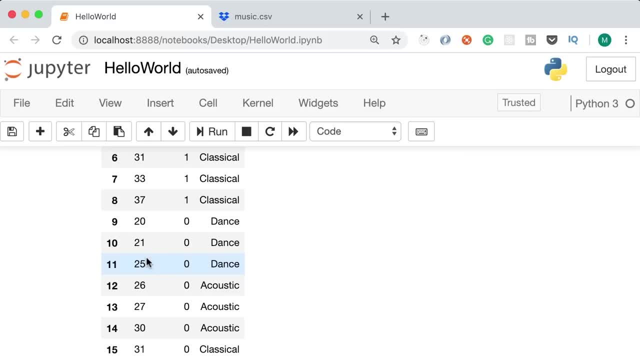 So, once again, if you ask our model to predict the kind of music that a 22 year old woman likes, we expect it to say dance. So, with these assumptions, let's go ahead and ask our model to make predictions. So, 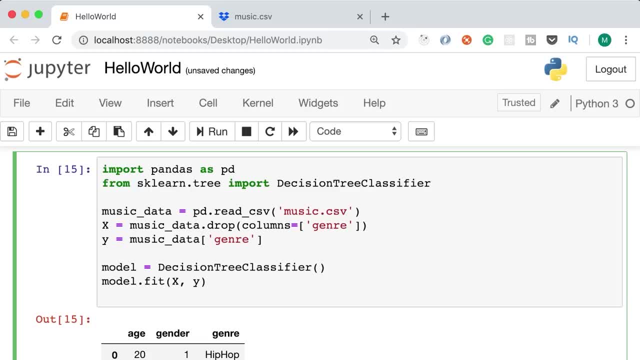 let's remove the last line and instead we're going to call modelpredict. This method takes a two dimensional array, So here's the outer array. in this array, each element is an array, So I'm going to pass another array here, and in this array I'm going to pass a new input set. 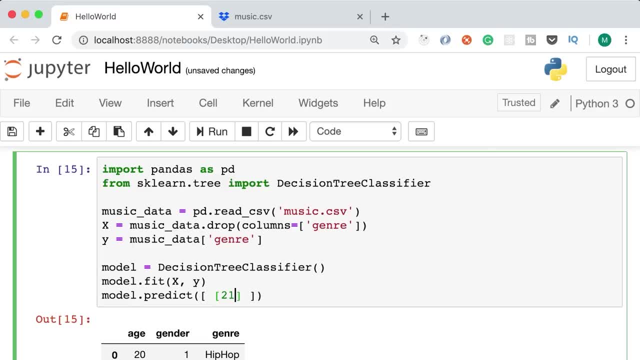 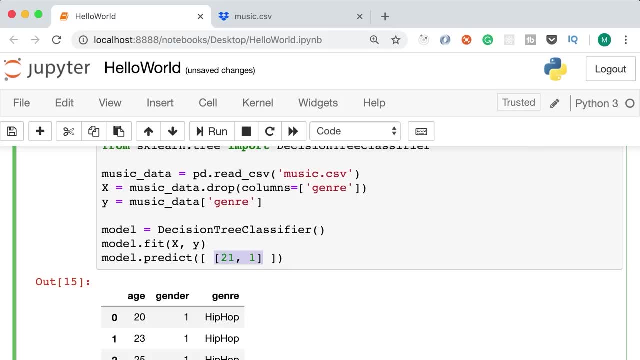 A 21 year old male, so 21, 1.. That is like a new record in this table. Okay, So this is one input set. let's pass another input set for a 22 year old female. So here's another array. 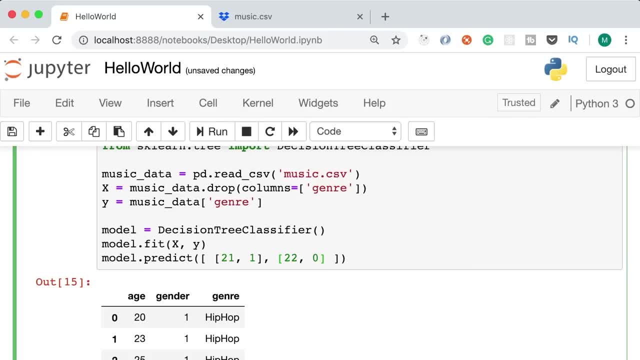 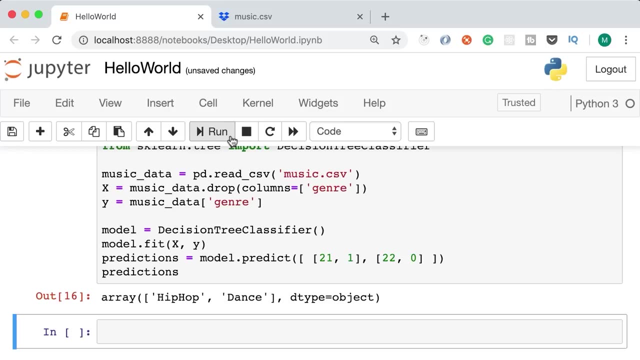 here we add 22,- 0.. So we're asking our model to make two predictions at the same time. We get the result and store it in a variable called predictions. and finally let's inspect that in our notebook Run. look what we got. 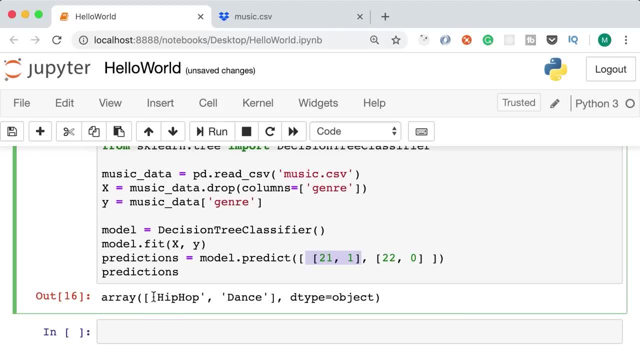 Our model is saying that a 21 year old male likes hip hop and a 22 year old female likes dance music. So our model could successfully make predictions here. beautiful, But wait a second. building a model that makes predictions accurately is not always that easy. 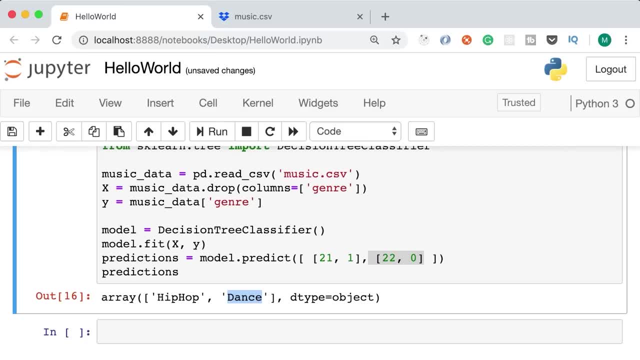 As I told you earlier, after we build a model, we need to measure its accuracy, And if it's not accurate enough, we should either fine tune it or build a model using a different algorithm. So in the next lecture, I'm going to show you how to measure the accuracy of a model. 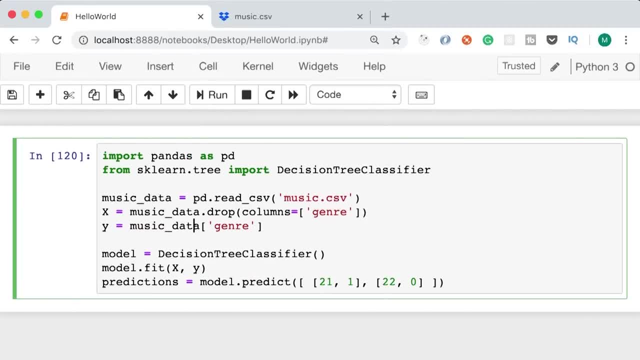 In this lecture, I'm going to show you how to measure the accuracy of your models. Now, in order to do so, first we need to split our data set into two sets: one for training and the other for testing. Because right now, 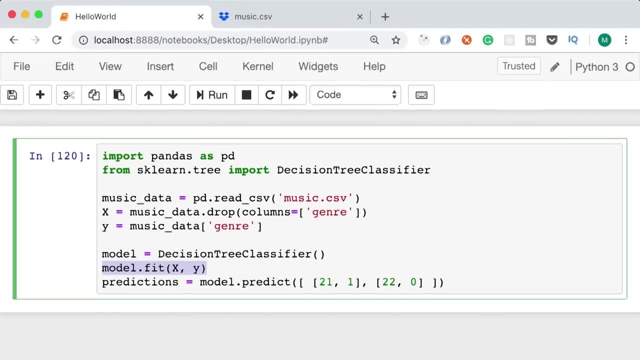 we're passing the entire data set for training the model and we're using two samples for making predictions. That is the only way to calculate the accuracy of a model. A general rule of thumb is to allocate 70-80% of our data for training. 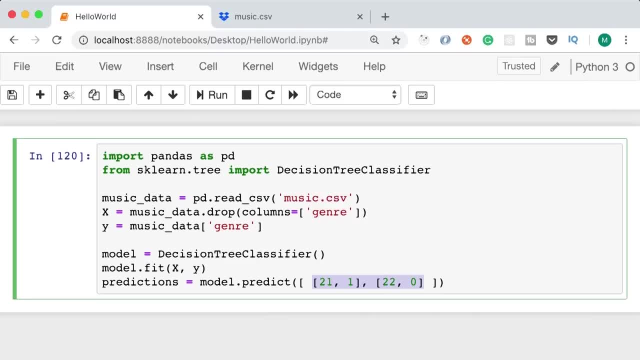 That is not enough to calculate the accuracy of a model. A general rule of thumb is to allocate 70-80% of our data for training and the other 20-30% for testing. Then, instead of passing only two samples for making predictions, 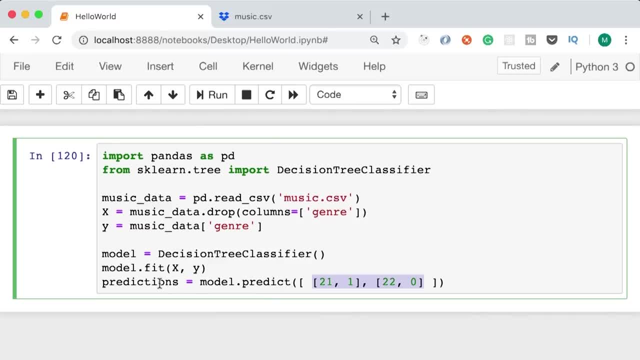 we can pass the data set we have for testing. we'll get the predictions and then we can compare these predictions with the actual values in the test set. Based on that, we can calculate the accuracy. That's really easy. all we have to do is to import a couple of functions and call them in this: 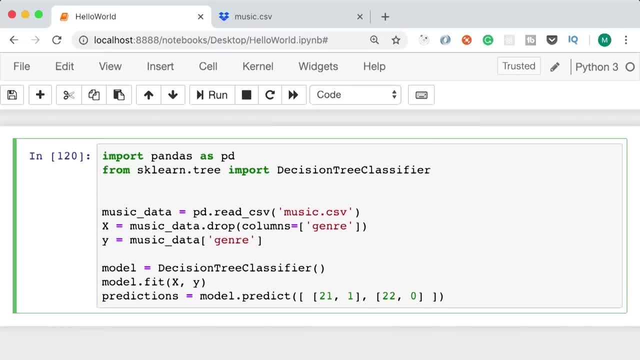 code. Let me show you So. first, on the top, from sklearnmodel, underline selection module, we import a function called train test split. With this function we can easily split our data set into two sets for training and testing. Now, right here, after we define x and y, 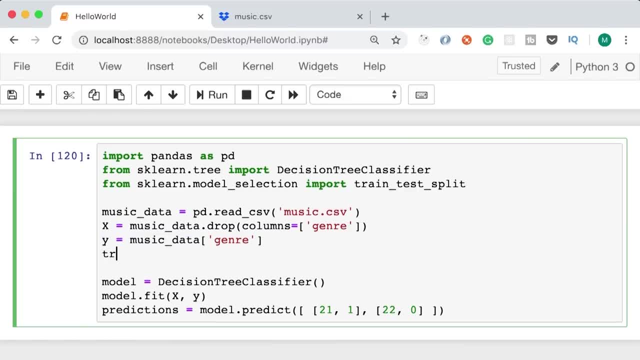 sets. we call this function So train test split. we give it three arguments: x, y and a keyword argument that specifies the size of our test data set. So test underline size. we set it to 0.2.. So we are allocating 20%. 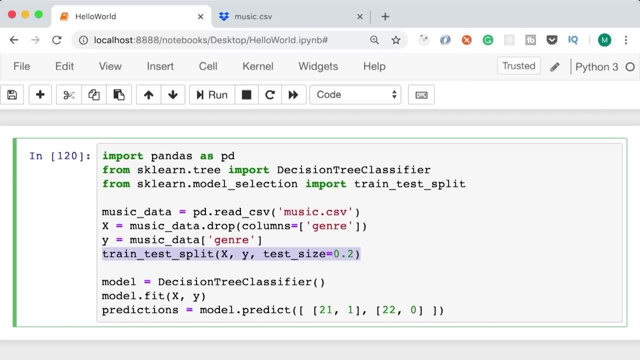 of our data for testing. Now this function returns a tuple, so we can unpack it into four variables right here: x underline train, x underline test, y underline train and y underline test. So the first two variables are the input sets for training. 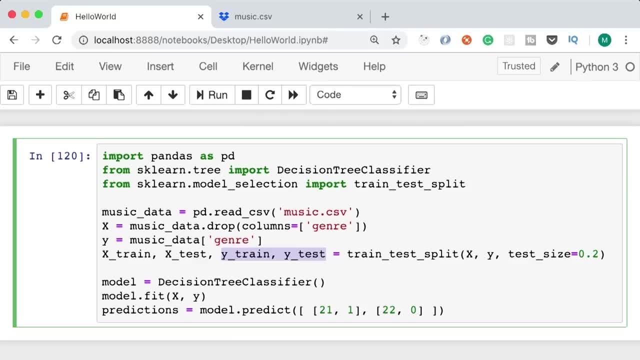 and testing and the other are the output sets for training and testing. Now, when training our model, instead of passing the data set, we want to pass only the training data set. So x underline train and y underline train. Also, when making predictions: 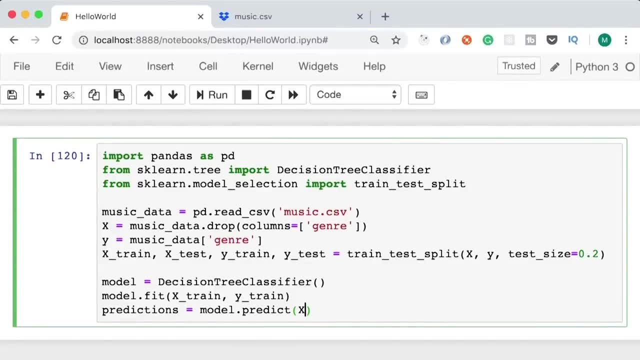 instead of passing these two samples, we pass x underline test. So that is the data set that contains input values for testing. Now we get the predictions. To calculate the accuracy, we simply have to compare these predictions with the actual values we have in our output set for. 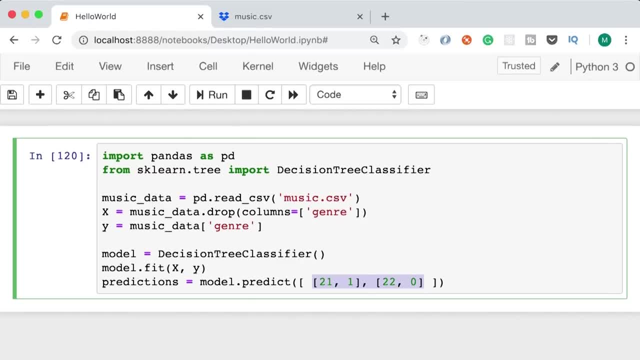 and the other 20-30% for testing. Then, instead of passing only two samples for making predictions, we can pass the data set we have for testing. we'll get the predictions and then we can compare these predictions with the actual values in the test set. Based on that, 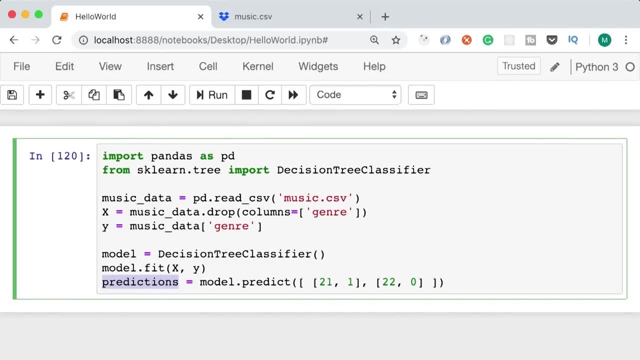 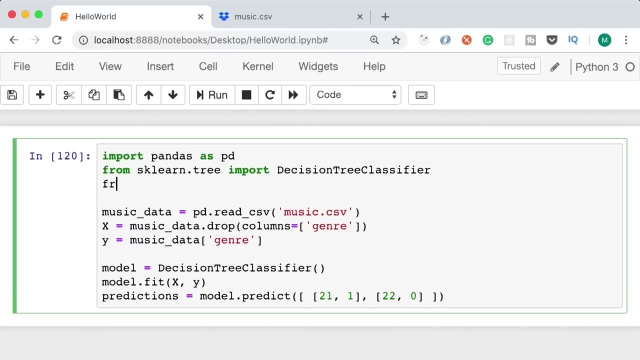 we can calculate the accuracy. That's really easy. all we have to do is to import a couple of functions and call them in this code. Let me show you So. first, on the top from sklearn, that model underline selection module, we import a function called train test split. 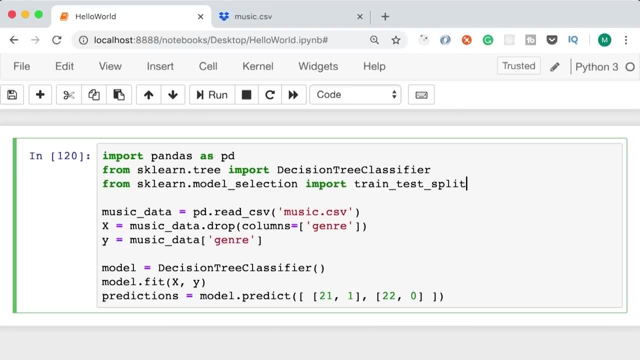 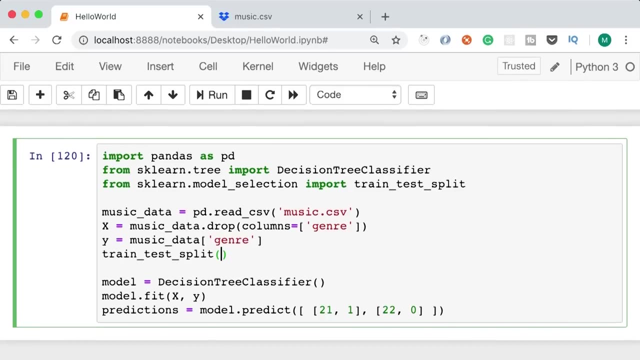 With this function we can easily split our data set into two sets for training and testing. Now, right here, after we define x and y sets, we call this function So train test split. we give it three arguments: x, y, 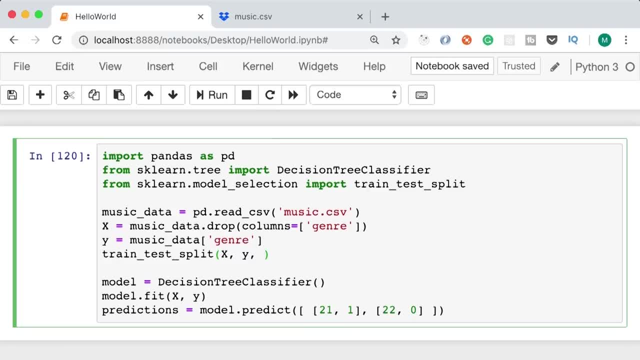 and a keyword argument that specifies the size of our test data set. So, test underline size, we set it to 0.2. So we are allocating 20% of our data for testing. Now this function returns a tuple, so we can. 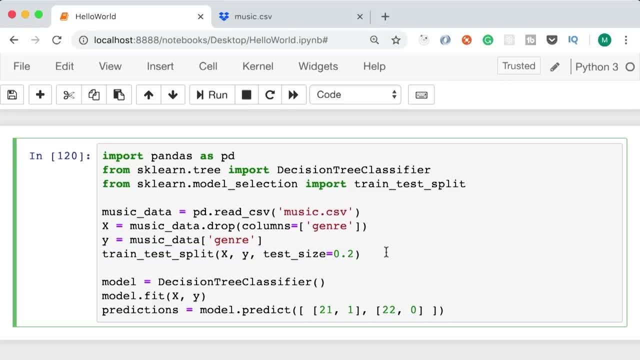 unpack it into four variables right here: Underline train, x underline test, y underline train and y underline test. So the first two variables are the input sets for training and testing and the other are the output sets for training and testing. Now, when training. 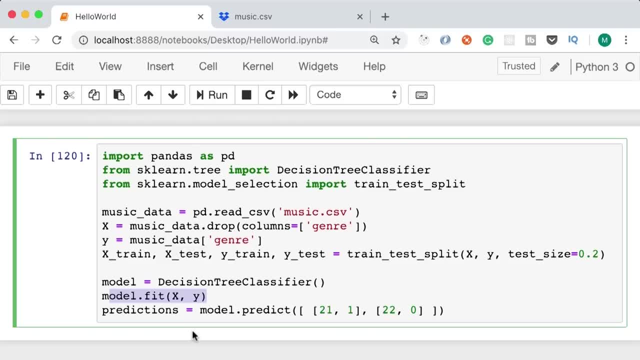 our model. instead of passing the entire data set, we want to pass only the training data set. So x underline train and y underline train. Also, when making predictions, instead of passing these two samples, we pass x underline test. 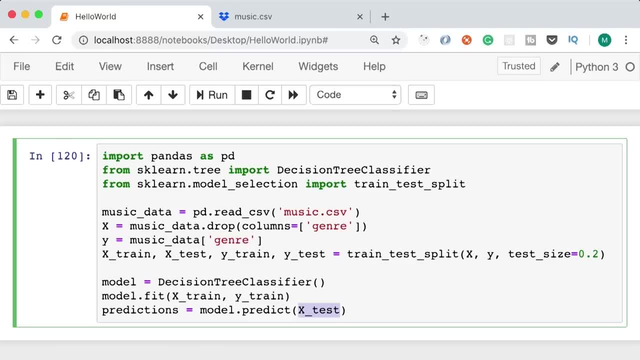 So that is the data set that contains input values for testing. Now we get the predictions. To calculate the accuracy, we simply have to compare these predictions with the actual values we have in our output set for testing. That is very easy. First, on the top, we need to import a function. so 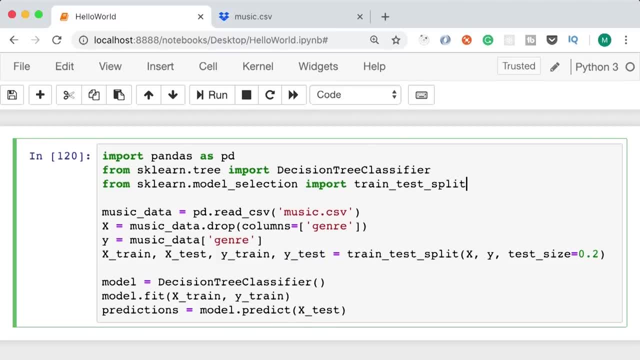 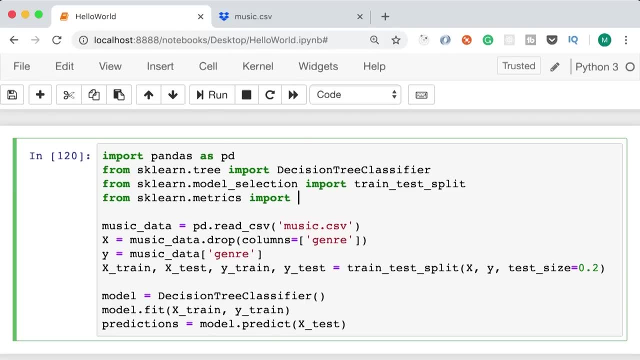 testing. That is very easy. First, on the top, we need to import a function, so from sklearnmetrics, import accuracy underline score. Now, at the very end, we call this function so accuracy score and give it two arguments: y, underline test. 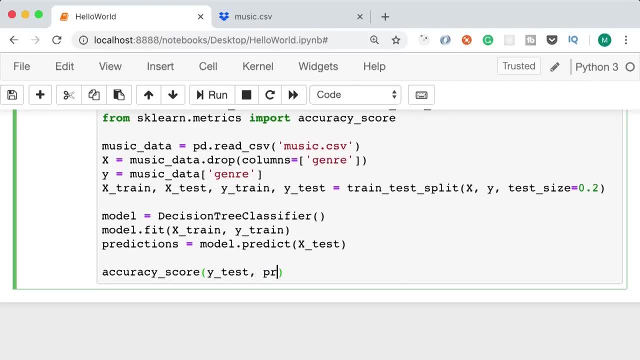 which contains the expected values, and predictions, which contains the actual values. Now this function returns an accuracy score between 0 to 1. So we can store it here and simply display it on the console. So let's go ahead and run this program. so the accuracy score is. 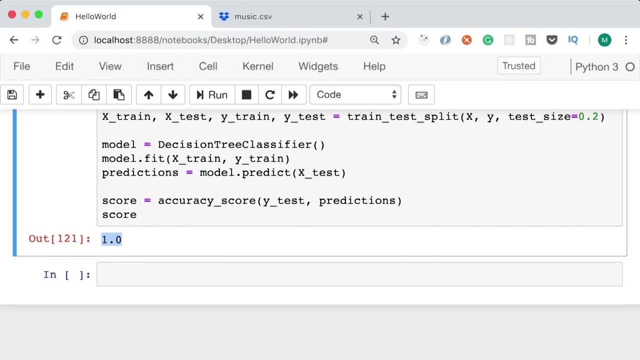 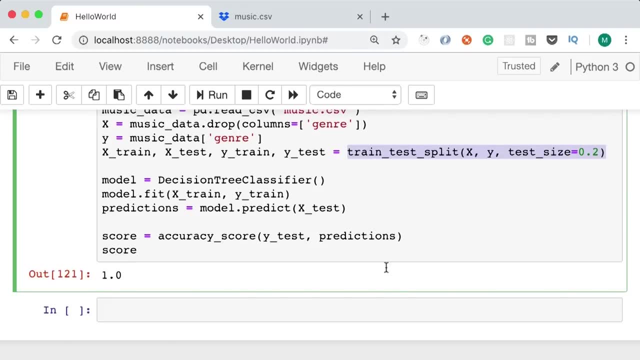 1 or 100%. but if we run this one more time, we're going to see a different result, because every time we split our data set into training and test sets, we'll have different data sets, because this function randomly picks data for training and testing. Let me show you, So put the cursor. 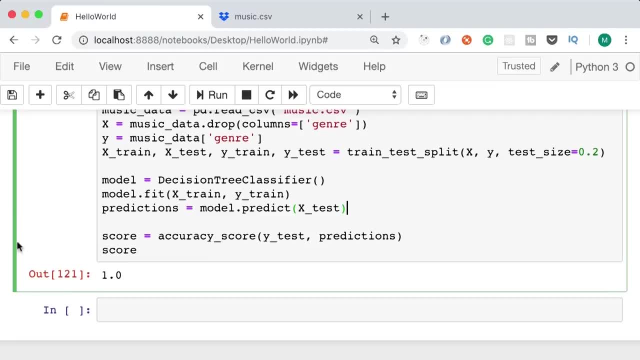 in the cell. now you can see this cell is activated. Note that if you click this button here, it will run this cell and also insert a new cell below this cell. Let me show you So if I go to the second cell. 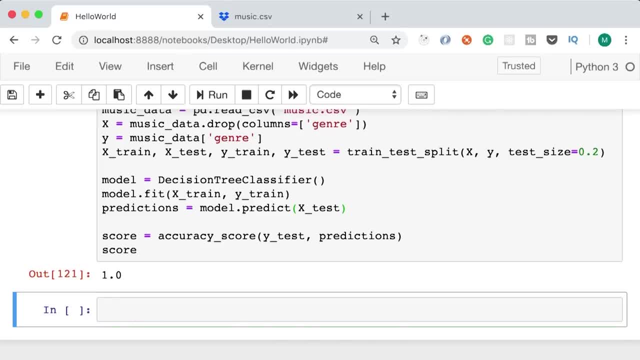 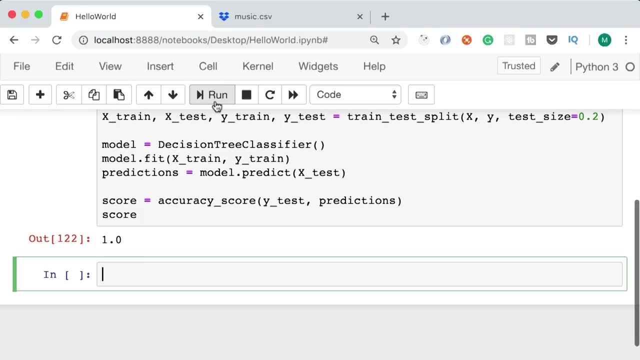 press the escape button. now we are in the command mode. press d twice. okay, now it's deleted. if we click the run button, you can see this code was executed and now we have a new cell. So if you want to run our first cell, 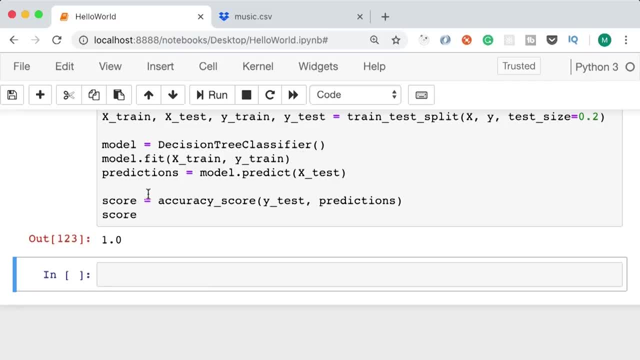 multiple times. every time we have to click this and then run it, and then click again and run it. it's a little bit tedious, So I'll show you a short cut. Activate the first cell and press control and enter. 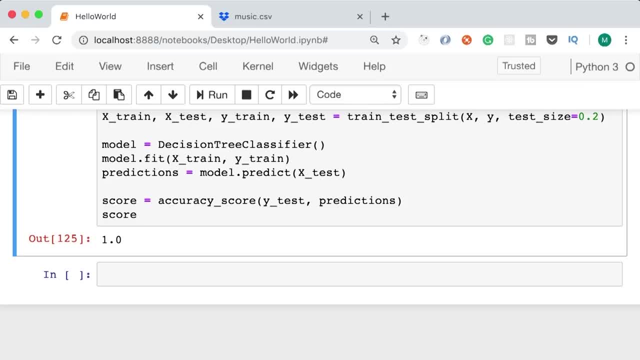 This runs the current cell without adding a new cell below it. So back here let's try it multiple times. okay, now look, the accuracy dropped to 0.75.. It's still good. so the accuracy score here is somewhere between: 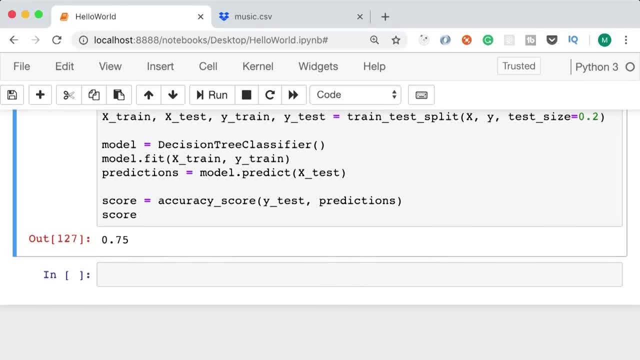 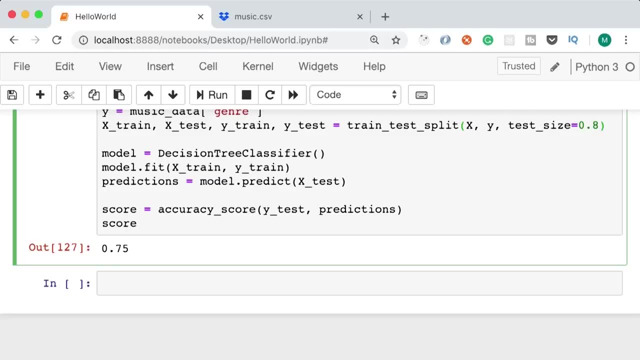 75% to 100%. But let me show you something If I change the test size from 0.2 to 0.8, so essentially we're using only 20% of our data for training this model and we're using the other 80% for testing. 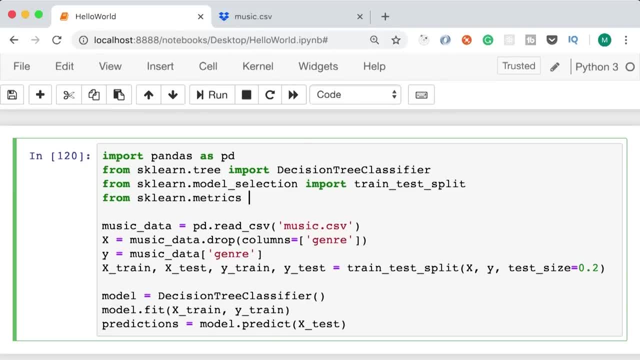 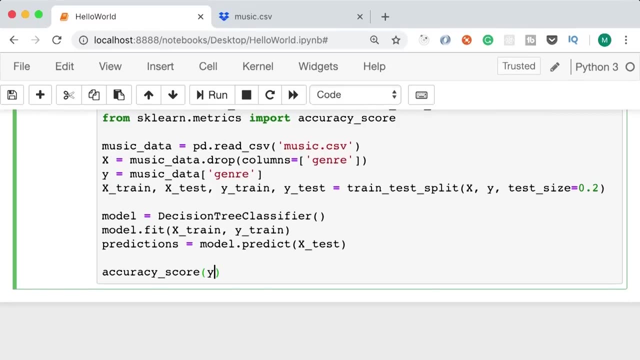 from sklearnmetrics. import: accuracy underline score. Now, at the very end, we call this function so accuracy score and give it two arguments: y underline test, which contains the expected values, and predictions, which contains the actual values. Now this function returns. 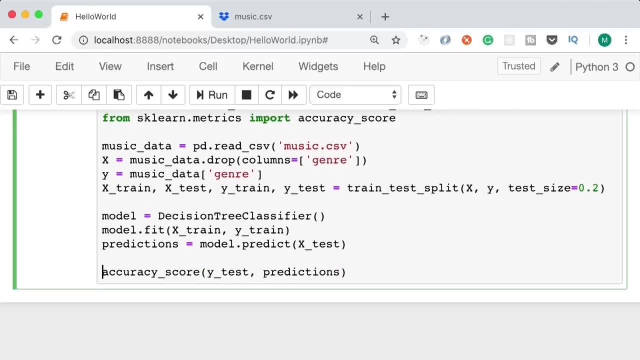 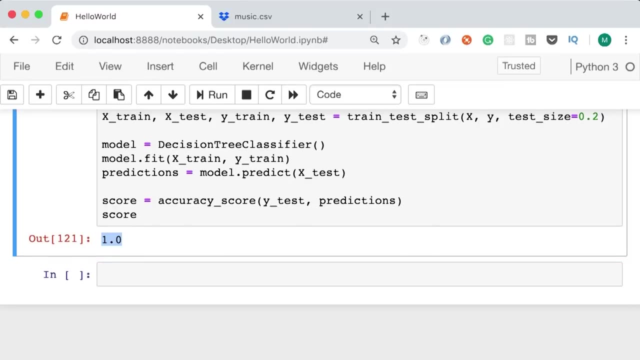 an accuracy score between 0 to 1.. So we can store it here and simply display it on the console. So let's go ahead and run this program. so the accuracy score is 1 or 100%. but if you run this one more time you're going to see a different result, because every time 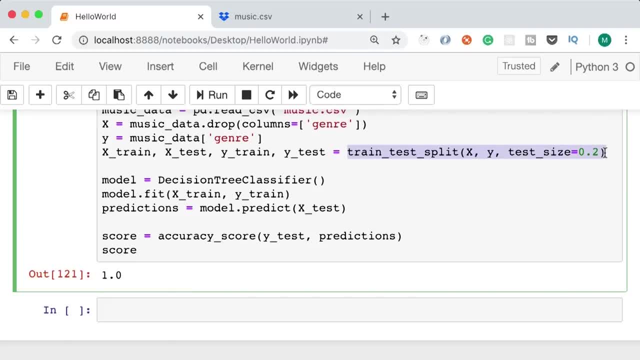 we split our data set into training and test sets, we'll have different data sets because this function randomly picks data for training and testing. Let me show you. So put the cursor in the cell. now you can see this cell is activated. Note that if you click this button here, it will. 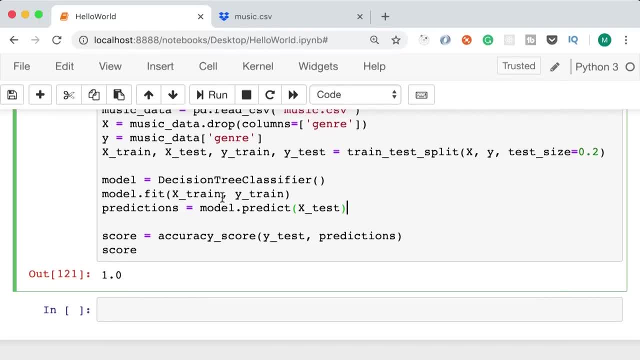 run this cell and also insert a new cell below this cell. Let me show you So. if I go to the second cell, press the escape button. now we are in the command mode. press d twice. okay, now it's deleted if we click the run button. 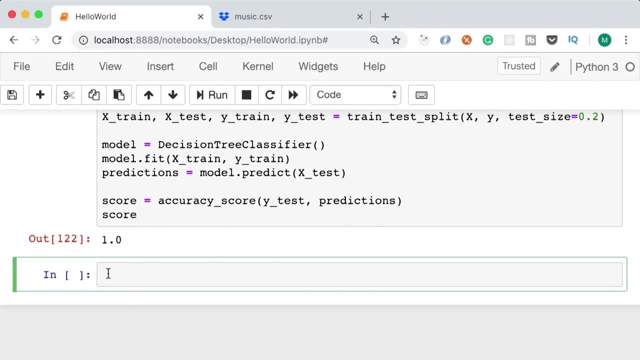 you can see, this code was executed and now we have a new cell. So if you want to run our first cell multiple times, every time we have to click this and then run it, and then click again and run it. it's a little bit. 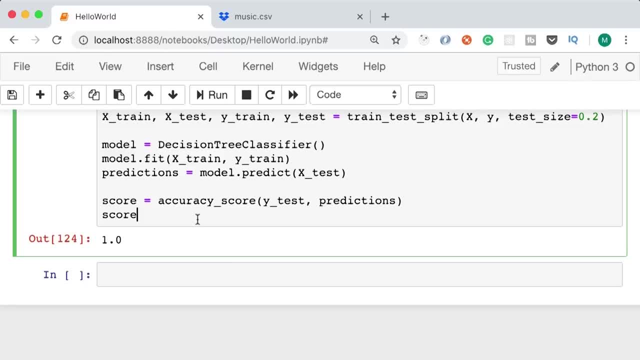 tedious, So I'll show you a shortcut: Activate the first cell and press control and enter. This runs the current cell without adding a new cell below it. So back here, let's run it multiple times. okay, now look the accuracy. 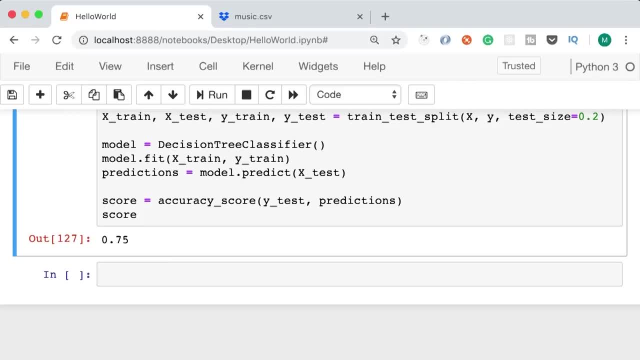 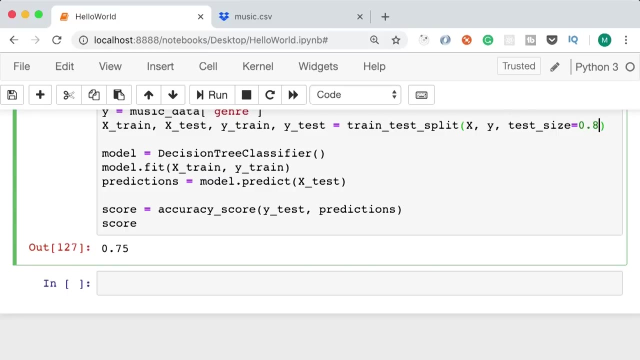 dropped to 0.7.. It's still good. so the accuracy score here is somewhere between 75% to 100%. But let me show you something. If I change the test size from 0.2 to 0.8, so essentially we're using only 20% of our 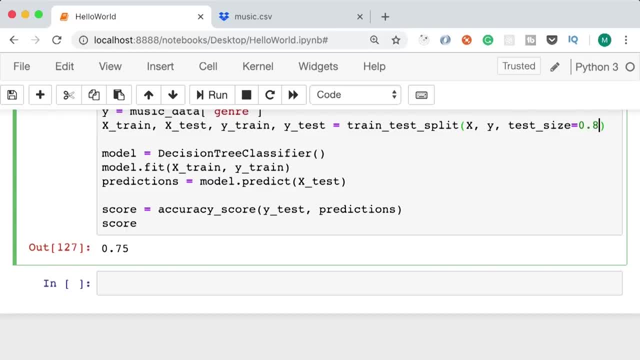 data for training this model and we're using the other 80% for testing. Now let's see what happens when we run this cell multiple times. So control and enter. look, the accuracy immediately dropped to 0.4.. One more time now: 46%. 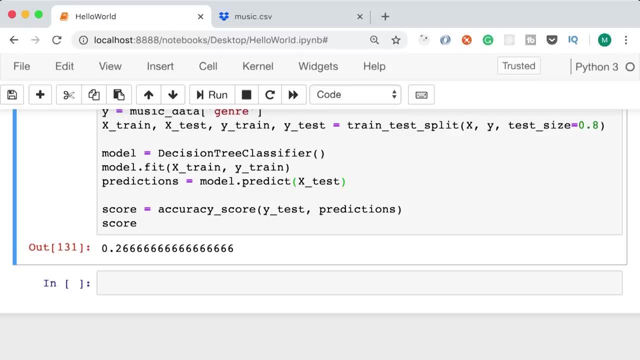 40%, 26%. it's really really bad. The reason this is happening is because we are using very little data for training this model. This is one of the key concepts in machine learning: The more data we give to our model and the cleaner 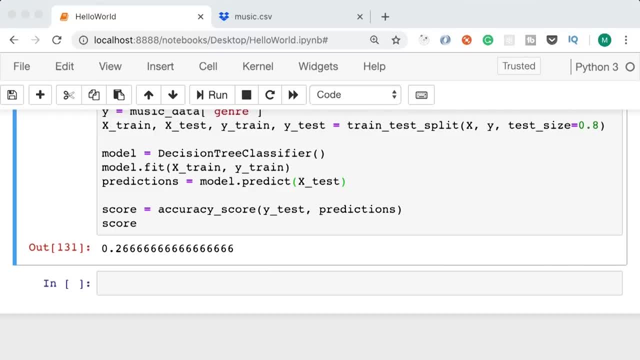 the data is, we get the better result. So if you have duplicates, irrelevant data or incomplete values, our model will learn bad patterns in our data. That is why it's really important to clean our data before training our model. Now let's change this back to 0.2,. 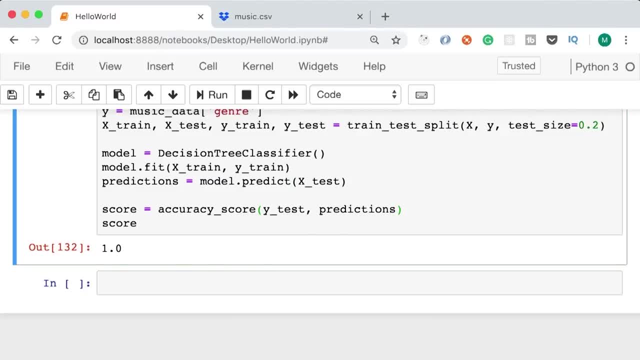 run this one more time. okay, now the accuracy is 1, 75%. now it dropped to 50% again. the reason this is happening is because we don't have enough data. Some machine learning problems require thousands or even millions of samples. 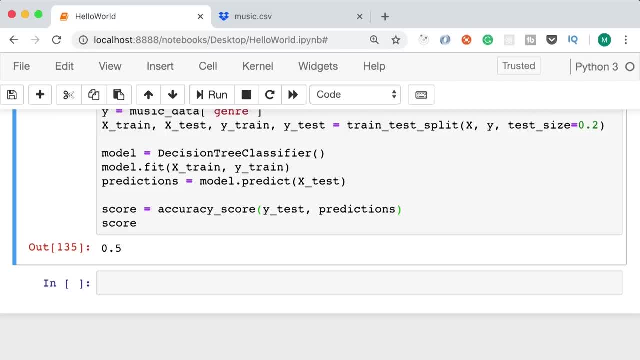 to train a model. The more complex the problem is, the more data we need. For example, here we're only dealing with a table of 3 columns, but if you want to build a model to tell if a picture is a cat or a dog or a horse or a lion, we'll need millions. 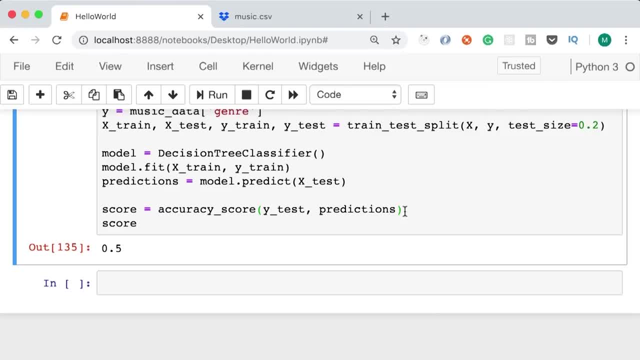 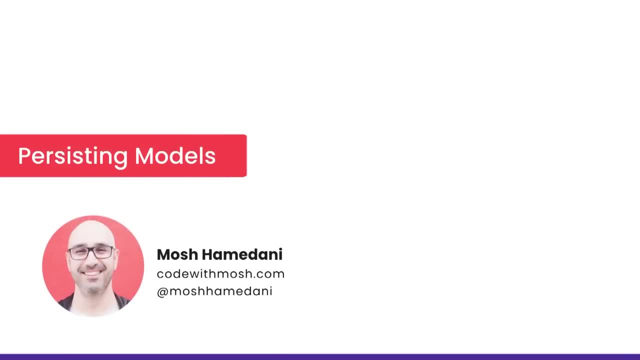 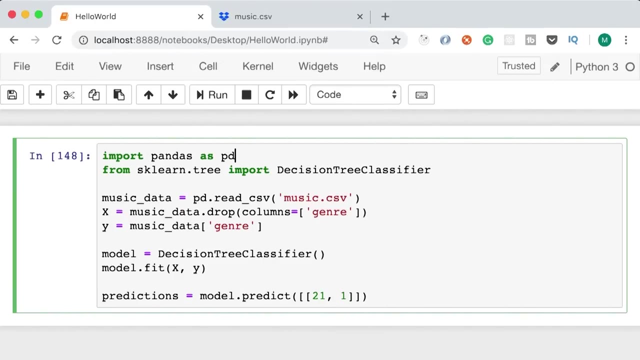 of pictures. The more animals we want to support, the more pictures we need. In the next lecture we're going to talk about model persistence. So this is a very basic implementation of building and training a model to make predictions. Now to simplify: 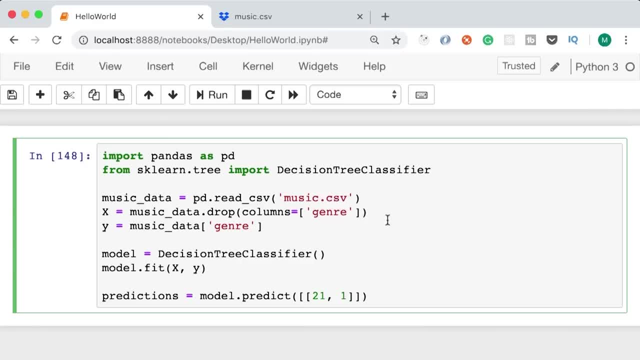 things. I have removed all the code that I've used in this video, The code that we wrote in the last lecture for calculating the accuracy, because in this lecture we're going to focus on a different topic. So basically, we import our data set, create a model, train it and then 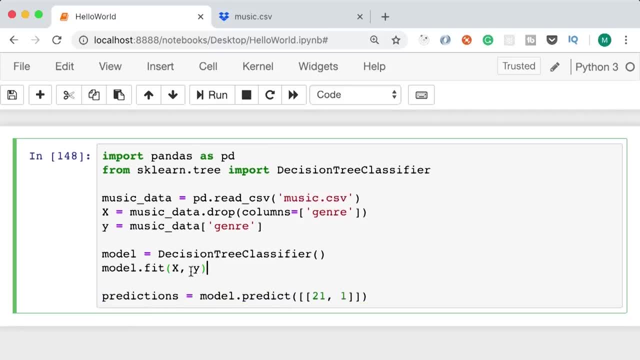 ask it to make predictions. Now, this piece of code that you see here is not what we want to run every time we have a new user or every time we want to make recommendations to an existing user, Because training a model can sometimes be really time consuming. In this example, we're dealing 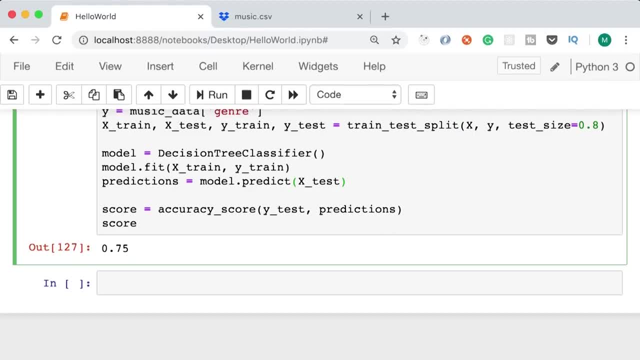 Now let's see what happens when we run this cell multiple times. So control and enter. look the accuracy immediately dropped to 0.4,. one more time now: 46%, 40%, 26%. it's really, really bad. The reason this is happening is because we are using very 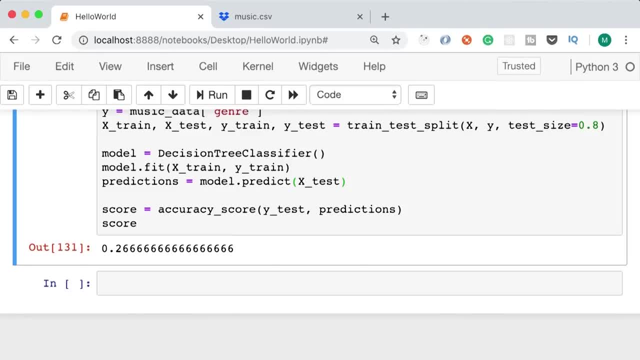 little data for training this model. This is one of the key concepts in machine learning. The more data we give to our model and the cleaner the data is, we get the better result. So if you have duplicates, irrelevant data or incomplete values, our model will learn bad patterns in our data. 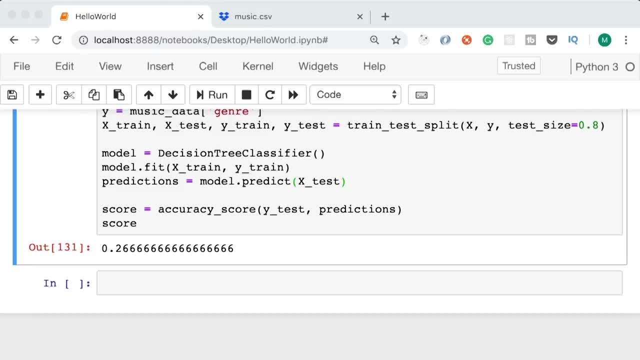 That is why it's really important to clean our data before training our model. Now let's change this back to 0.2, run this one more time. okay, now the accuracy is 1, 75%. now it dropped to 50% again. 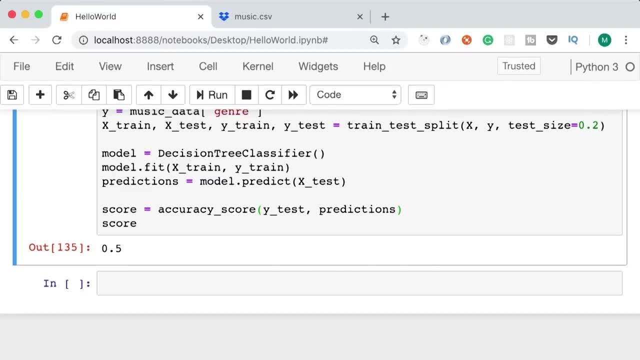 the reason this is happening is because we don't have enough data. Some machine learning problems require thousands of data, thousands of data, thousands of data Or even millions of samples to train a model. The more complex the problem is, the more data we need, For example. here we are only dealing with. 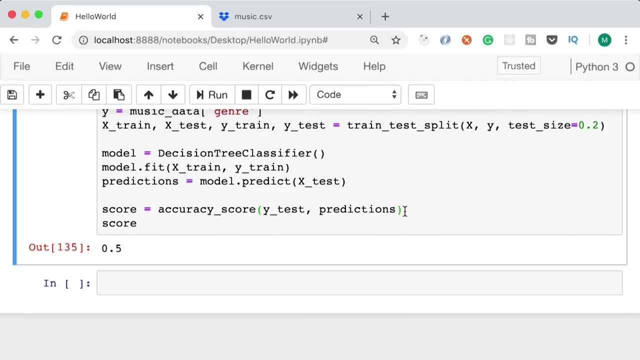 a table of three columns, but if you want to build a model to tell if a picture is a cat or a dog or a horse or a lion, we'll need millions of pictures. The more animals we want to support, the more pictures we need. 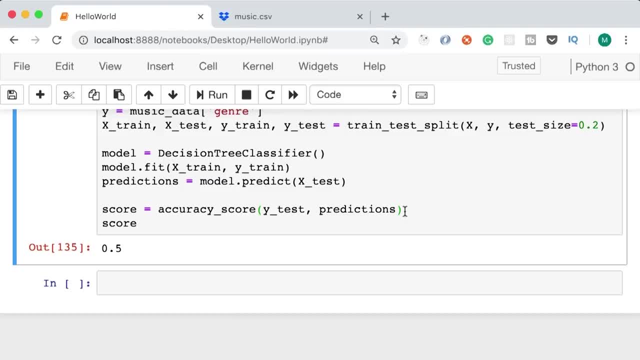 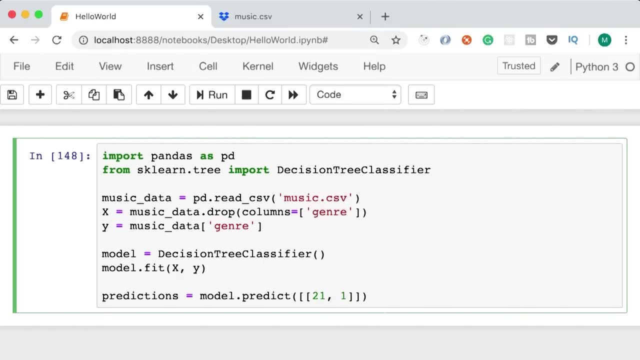 In the next lecture we're going to talk about model persistence. So this is a very important implementation of building and training a model to make predictions. Now, to simplify things, I have removed all the code that we wrote in the last lecture for calculating the accuracy, because in this lecture we're going to focus. 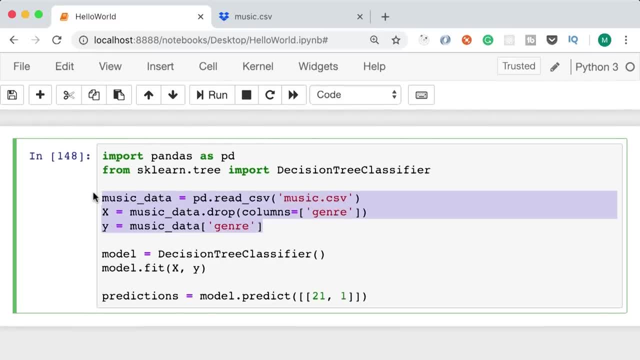 on a different topic. So, basically, we import our data set, create a model, train it and then ask it to make predictions. Now, this piece of code that you see here is not what we want to run every time we have a new user, or every time 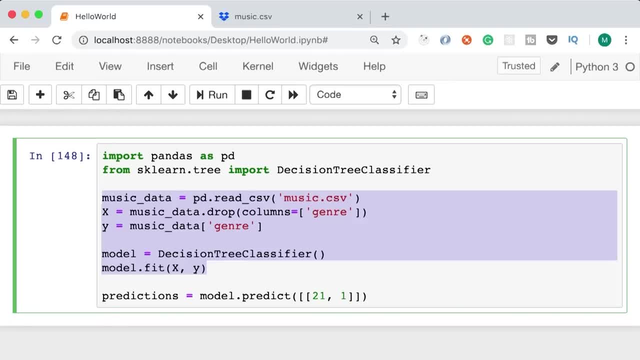 we want to make recommendations to an existing user, Because training a model can sometimes be really time consuming. In this example, we're dealing with a very small data set that has only 20 records, But in real applications we might have a data set with thousands or millions of samples. 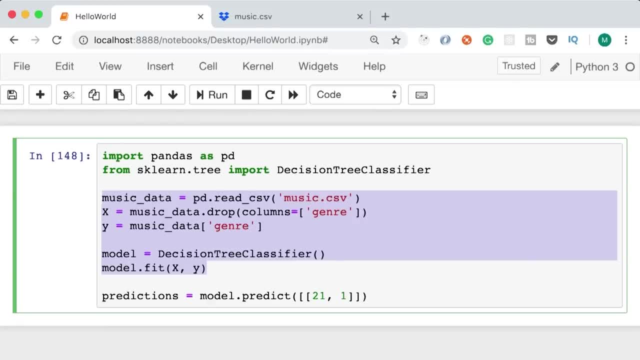 with a very small data set that has only 20 records. But in real applications we might have a data set with thousands or millions of samples. Training a model for that might take seconds, minutes or even hours. So that is why model persistence is important Once in a while. 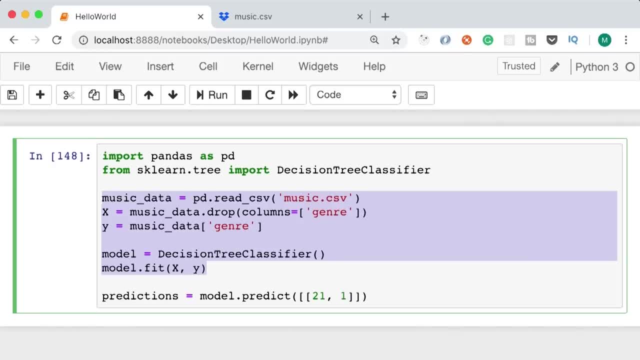 we build and train our model and then we'll save it to a file. Now, next time we want to make predictions, we simply load the model from the file and ask it to make predictions. That model is already trained, We don't need to retrain it. It's like an intelligent person. 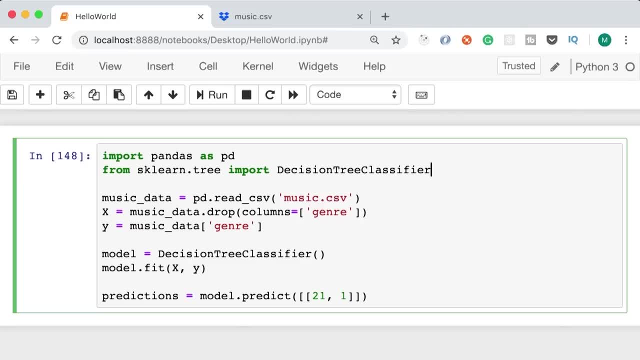 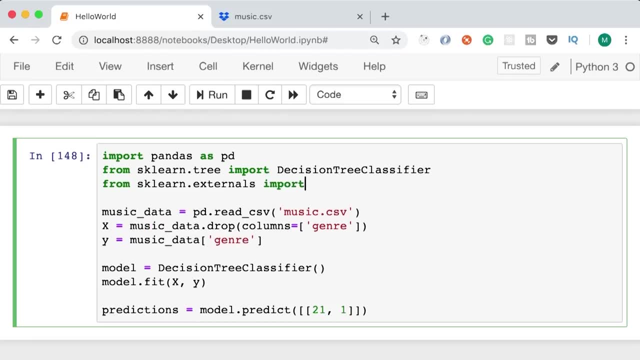 So let me show you how to do this. It's very, very easy. On the top from sklearnexternals module, we import joblib. This joblib object has methods for saving and loading models. So after we train our model, 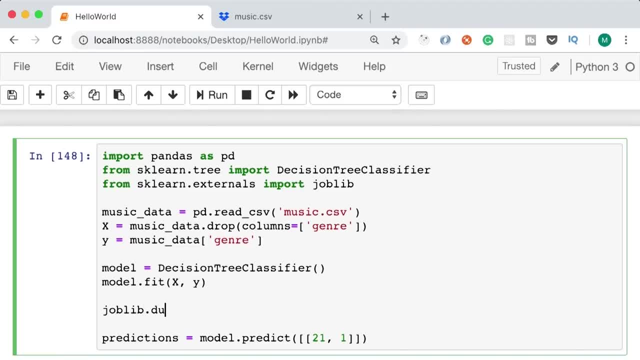 we simply call joblibdump and give it two arguments: Our model and the name of the file in which we want to store this model. Let's call that music-recommenderjoblib. That's all we have to do Now, temporarily. 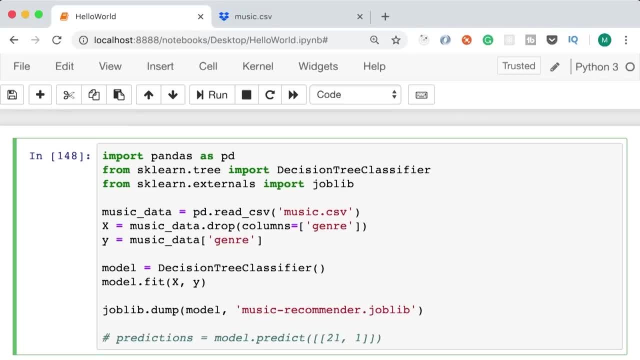 I'm going to comment out this line. We don't want to make any predictions, we just want to store our trained model in a file. So let's run the cell with control and slash. Okay, look in the output we have an array that contains the name of our model file. 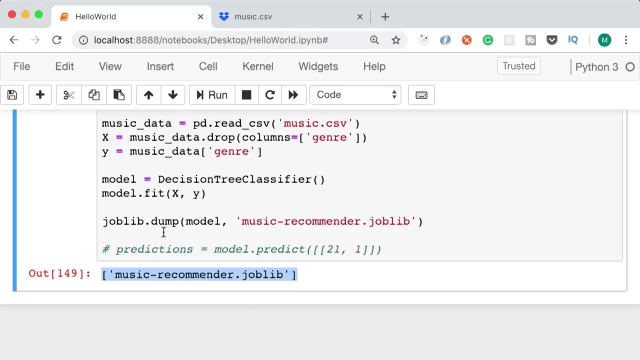 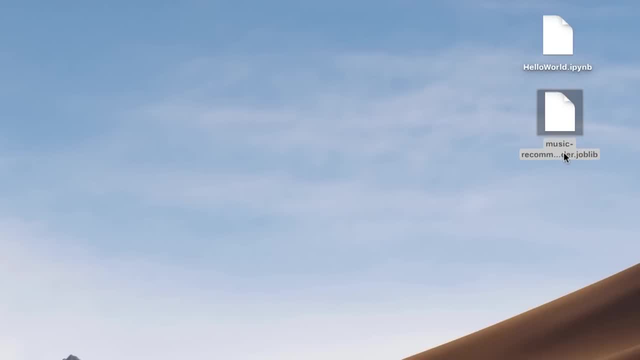 So this is the return value of the dump method. Now back to our desktop. right next to my notebook you can see our joblib file. this is where our model is stored. It's simply a binary file. Now back to our Jupyter notebook. As I told you before, in a real application we don't 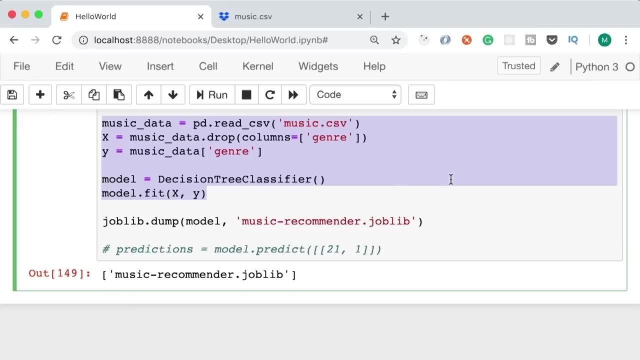 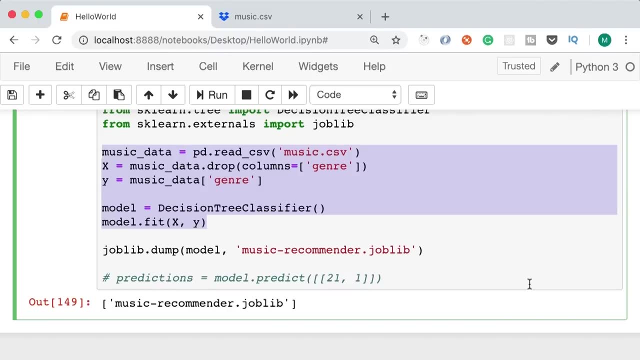 want to train a model every time. So let's comment out these few lines. So I've selected these few lines. on Mac, we can press command and slash and on Windows, control slash. Okay, these lines are commented out Now, this time, instead of. 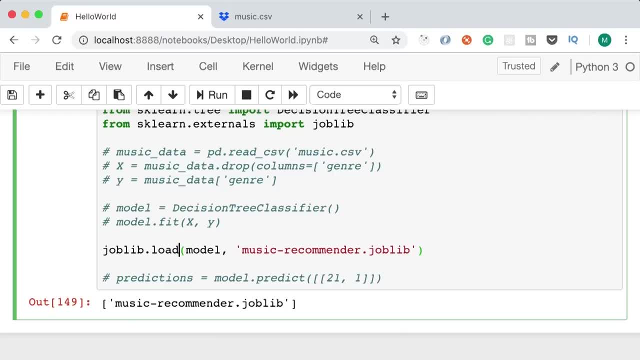 dumping our model. we're going to load it, So we call the load method. we don't have the model, we simply pass the name of our model file. This returns our trained model. Now, with these two lines, we can simply make predictions. So 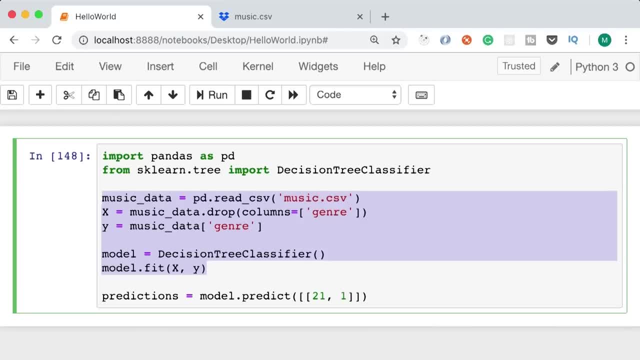 Training a model, for that might take seconds, minutes or even hours. So that is why model persistence is important. Once in a while we build and train our model, and then we'll save it to a file. Now. next time we want to make predictions, we simply load the model from the file. 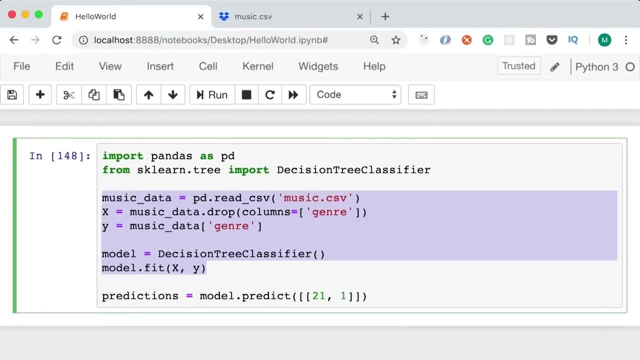 and ask it to make predictions. That model is already trained. We don't need to retrain it. It's like an intelligent person. So let me show you how to do this. It's very, very easy. On the top from sklearnexternals module. 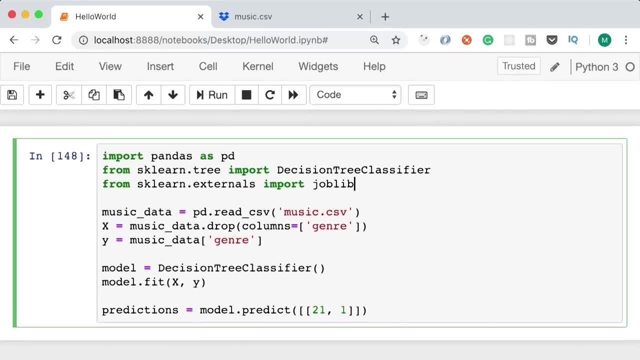 we import joblib. This joblib object has methods for saving and loading models. So after we train our model, we simply call joblibdump and give it two arguments: Our model and the name of the file in which we want to store this model. Let's call that music. 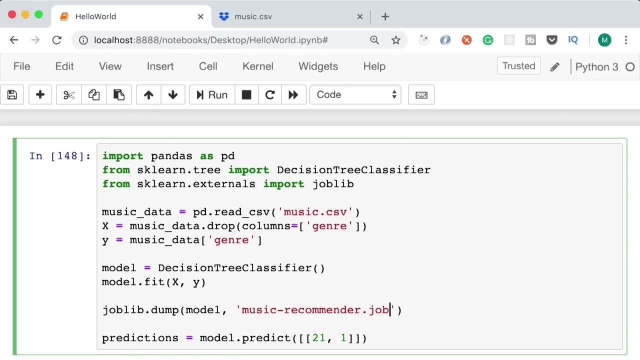 dash. recommender: dot joblib. That's all we have to do Now, temporarily. I'm going to comment out this line: we don't want to make any predictions, we just want to store our trained model in a file. So let's run the cell with control and slash. 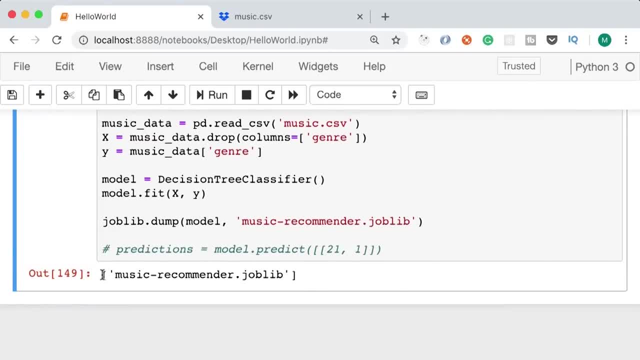 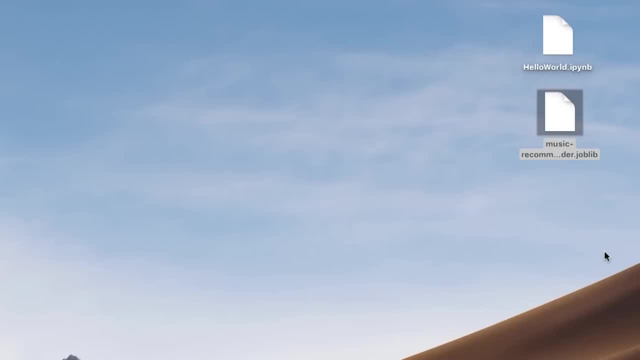 okay, look. in the output we have an array that contains the name of our model file. So this is the return value of the dump method. Now back to our desktop. right next to my notebook you can see our joblib file. this is where our model is stored. it's simply a binary file. 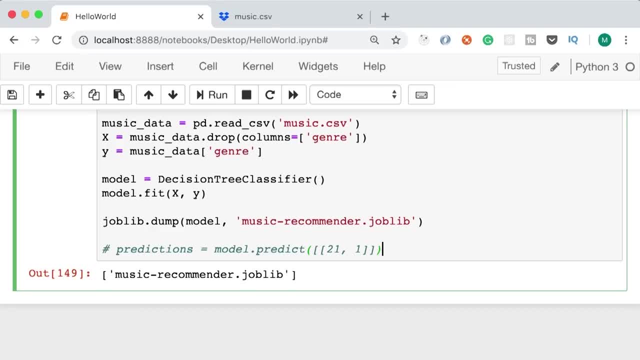 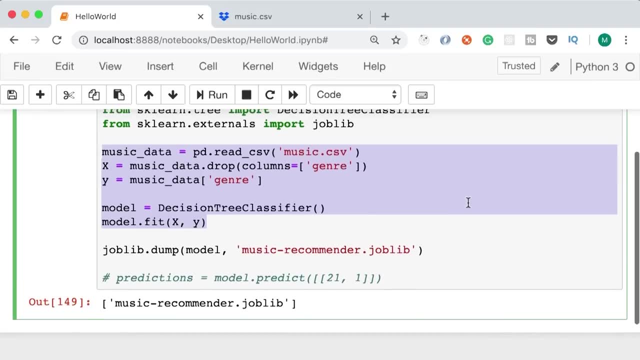 Now back to our Jupyter notebook. As I told you before, in a real application we don't want to train a model every time, So let's comment out these few lines. so I've selected these few lines. on mac, we can press, command and slash, and on windows, 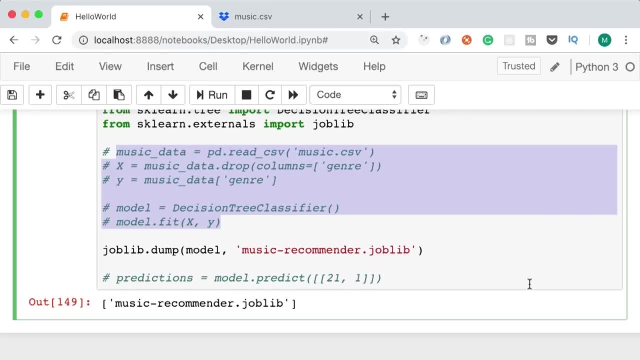 control slash. Okay, these lines are commented out now. this time, instead of dumping our model, we're going to load it, so we call the load method. we don't have the model, we simply pass the name of our model file. This returns our trained model. 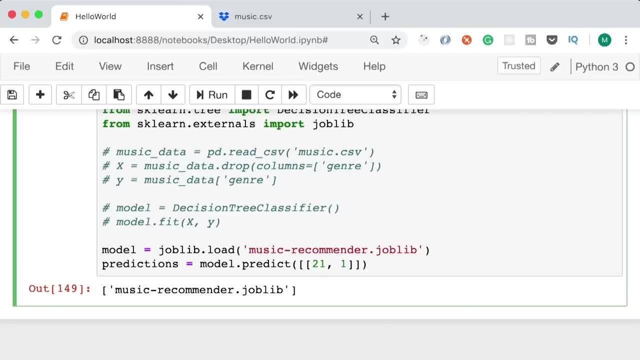 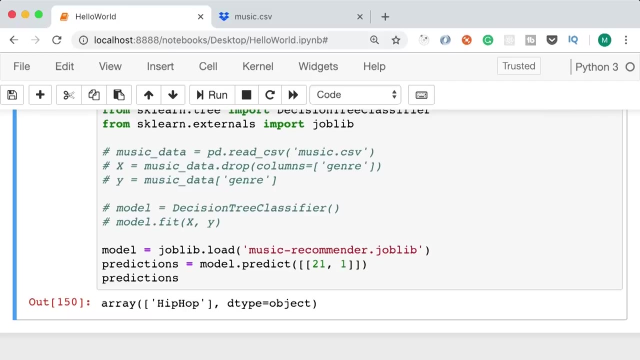 now, with these two lines, we can simply make predictions. So earlier we assumed that men between 20 and 25 like hip hop music. Let's print predictions and see if our model is behaving correctly or not. So control and enter, there you go. So this is how we persist. 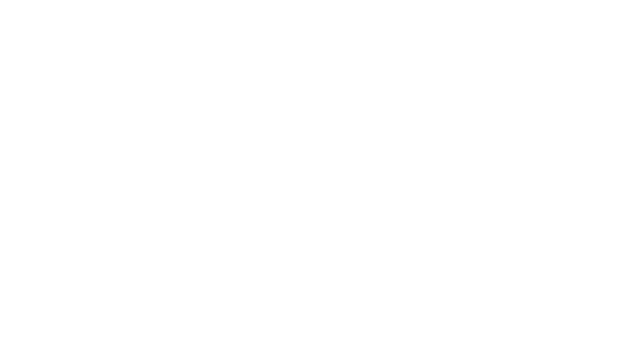 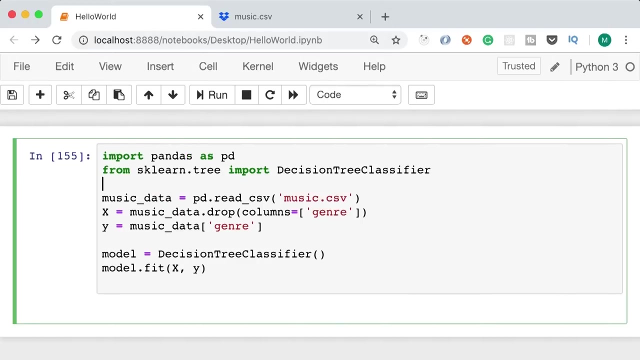 and load models. Earlier in this section, I told you that decision trees are the easiest to understand and that's why we started machine learning with decision trees. In this section, we're going to export our model in a visual format so you will see how this model makes predictions, That is. 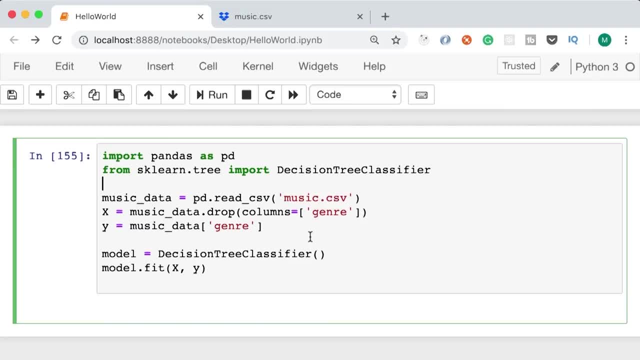 really, really cool. let me show you. So once again, I've simplified this code, so we simply import our data set, create input and output sets, create a model and train it. That's all we are doing. Now I want you to follow along with me, type everything exactly as I show you. 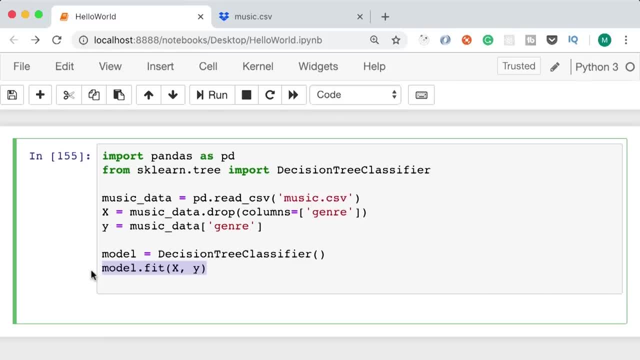 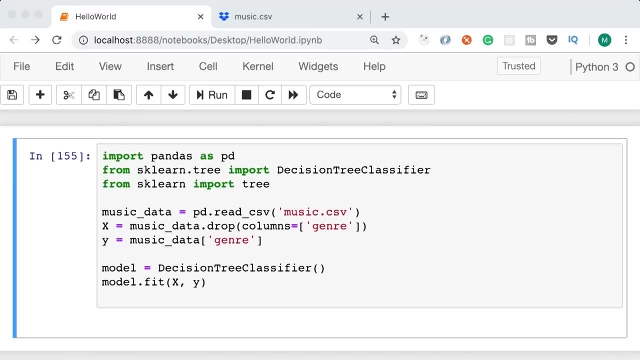 in this lecture. don't worry about what everything looks like. We're going to come back to it shortly. So on the top from sklearn import tree, This object has a method for exporting our decision tree in a graphical format. So after we train our model, 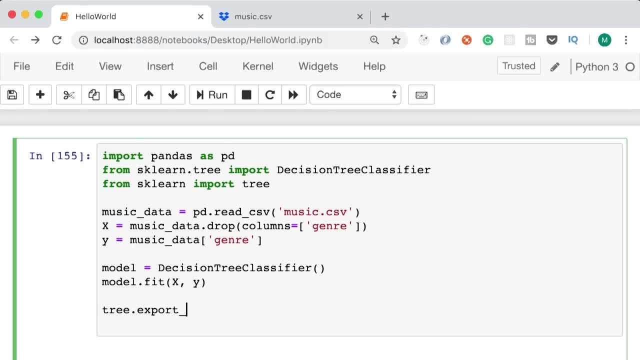 let's call treeexport. underline graph viz. Now here are a few arguments we need to pass. The first argument is our model. the second is the name of the output file. So here we're going to use the name of the output file. So here we're going to use the name of the output file. 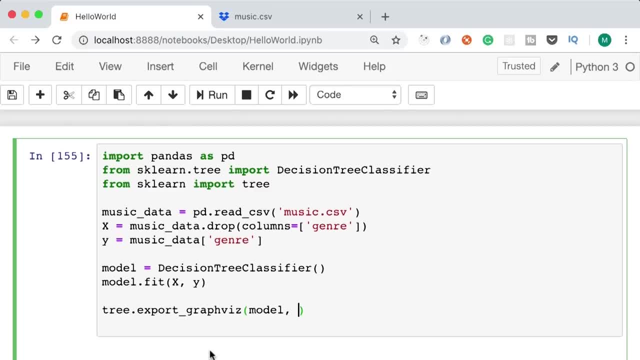 We're going to use keyword arguments because this method takes so many parameters and we want to selectively pass keyword arguments without worrying about their order. So the parameter we're going to set is out underline file. let's set this to music dash. recommender: dot dot. 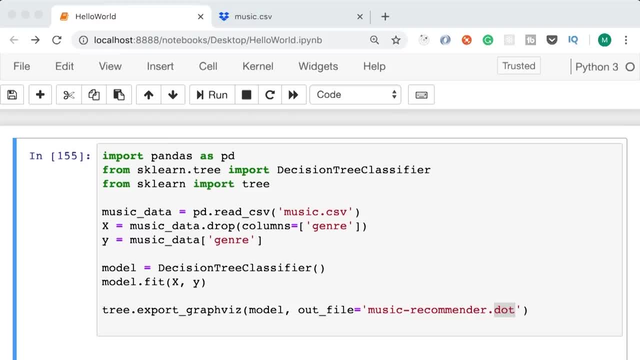 This is the dot format, which is a graph description language. you'll see that shortly Now. the other parameter we want to set is feature underline names. we set this to an array of two strings: age and gender. These are the features, or the columns of our data set. So they are. 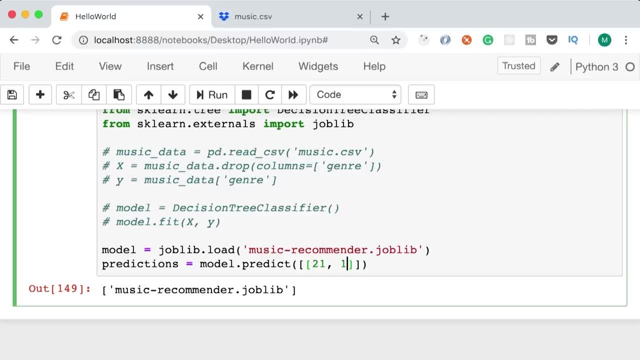 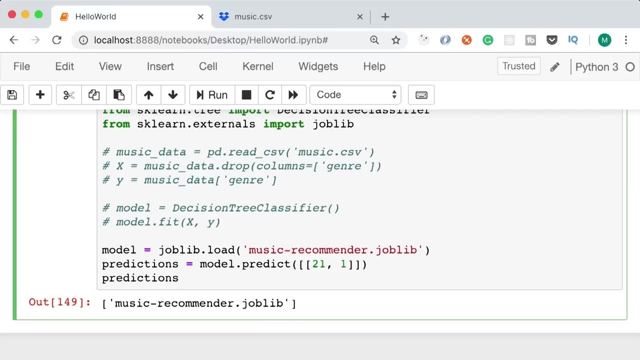 earlier we assumed that men between 20 and 25 like hip hop music. Let's print predictions and see if our model is behaving correctly or not. So control and enter. there you go. So this is how we persist and load models. 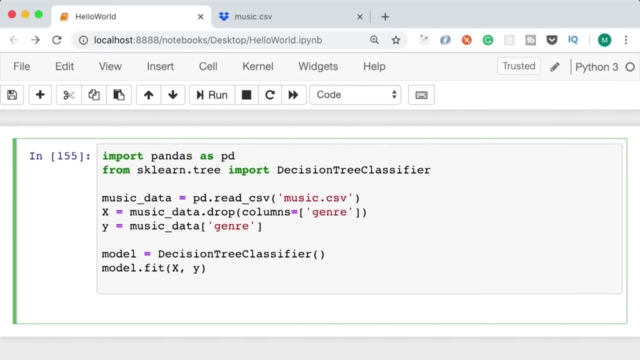 Earlier in this section, I told you that decision trees are the easiest to understand and that's why we started machine learning with decision trees. In this section, we're going to export our model in a visual format, So you will see how this model makes predictions. 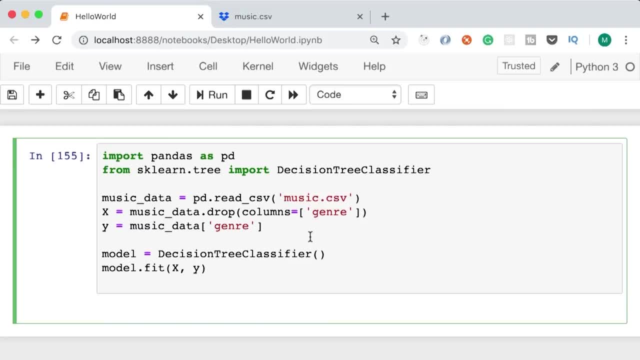 That is really, really cool. Let me show you So once again, I've simplified this code, so we simply import our data set, create input and output sets, create a model and train it. That's all we are doing. 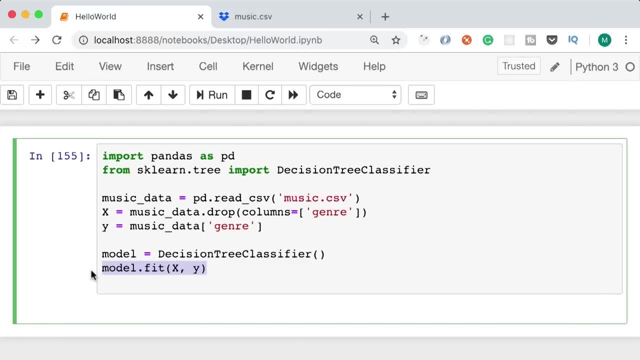 Now I want you to follow along with me. type everything exactly as I show you in this lecture. Don't worry about what everything means. we're going to come back to it shortly. So on the top we have our model, and on the bottom 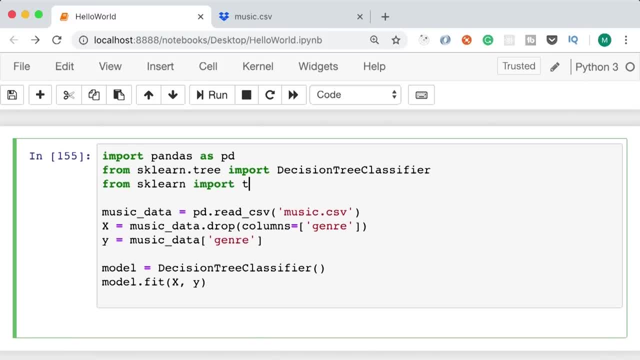 from sklearn import tree. This object has a method for exporting our decision tree in a graphical format. So after we train our model, let's call treeexport underline graph viz. Now here are a few arguments we need to pass. 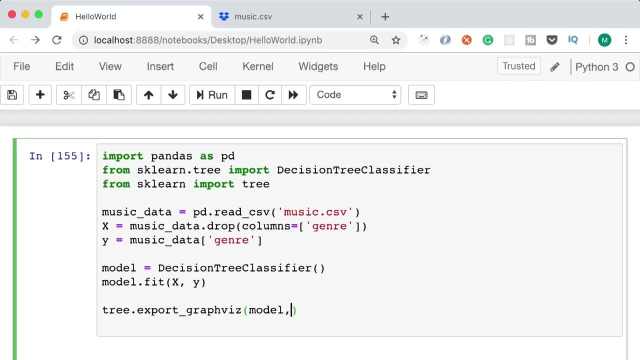 The first argument is our model, the second is the name of the output file. So here we're going to use keyword arguments because this method takes so many parameters. so we're going to call it tree And we want to selectively pass keyword arguments without worrying about their order. 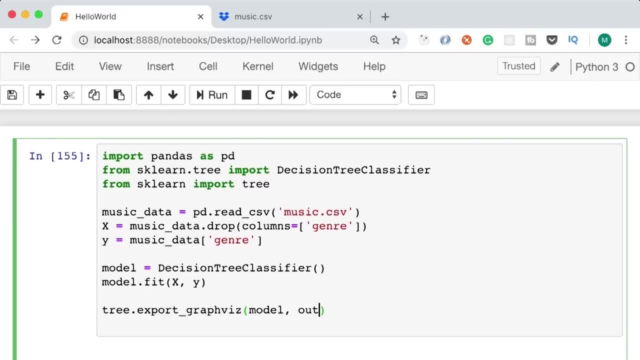 So the parameter we're going to set is out underline file. let's set this to music dash. recommender- dot- dot. This is the dot format, which is a graph description language. You'll see that shortly Now. the other parameter we want to set is: 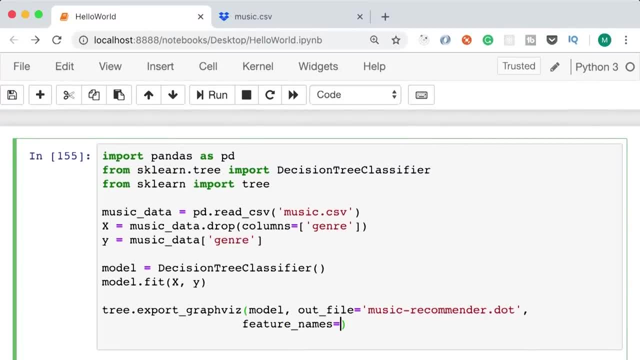 feature underline names. we set this to an array of two strings: age and gender. These are the features or the columns of our data set, So they are the properties or features of our data. The other parameter is class names. so class underline names. 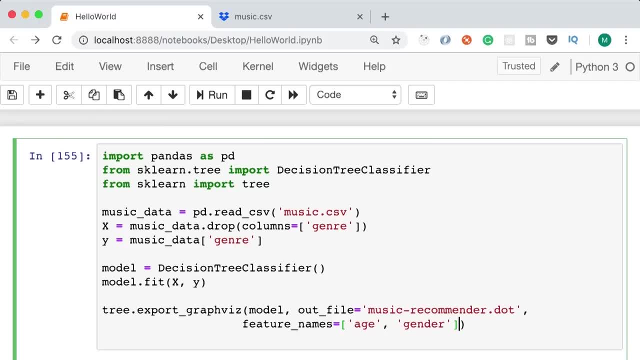 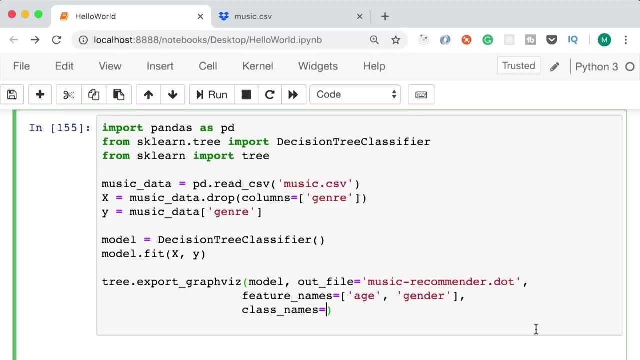 the properties or features of our data. The other parameter is class names, so class underline names. We should set this to the list of classes or labels we have in our output data set like hip hop, jazz, classical and so on. So this y data set includes: 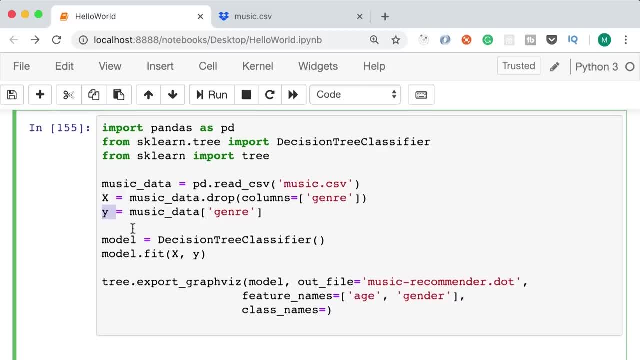 all the genres or all the classes of our data, but they are repeated a few times in this data set. So here we call y dot unique. this returns the unique list of classes. now we should sort this alphabetically, so we call the sorted function. 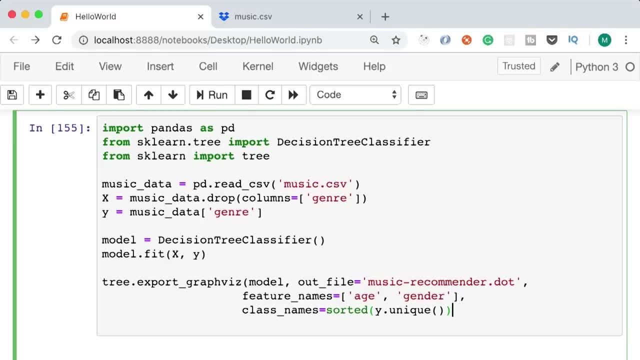 and pass the result of y dot unique. The next parameter is label. we set this to a string, all once again, don't worry about the details of these parameters. we're going to come back to this shortly. So set label to all, then rounded. 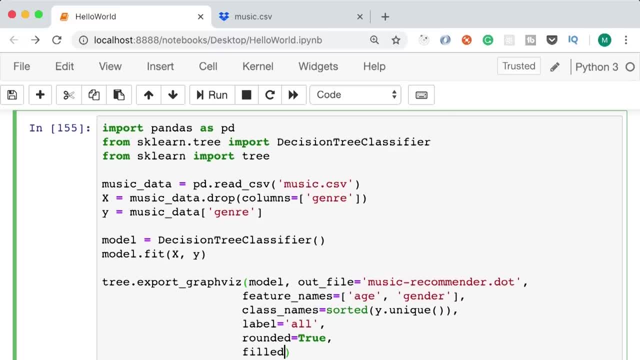 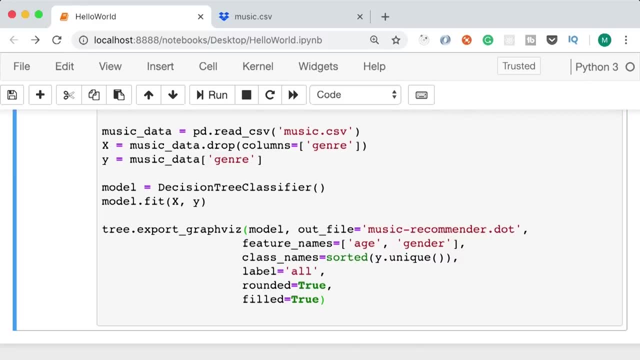 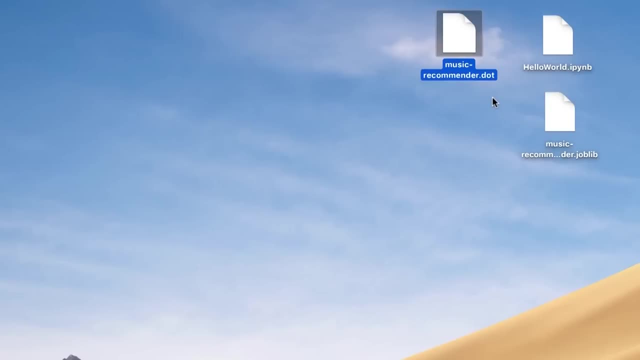 to true and finally filled to true. So this is the end result. Now let's run this cell using control and enter: Okay, Here we have a new file music recommender: dot dot. that's a little bit funny. 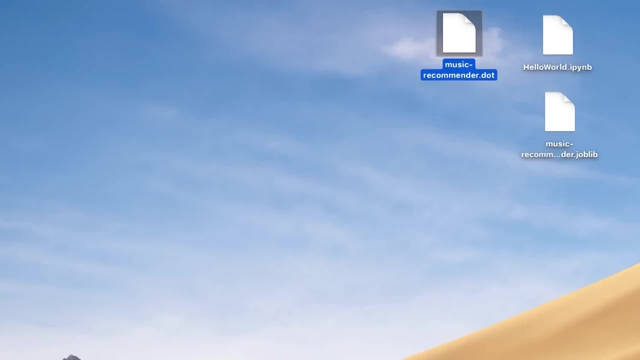 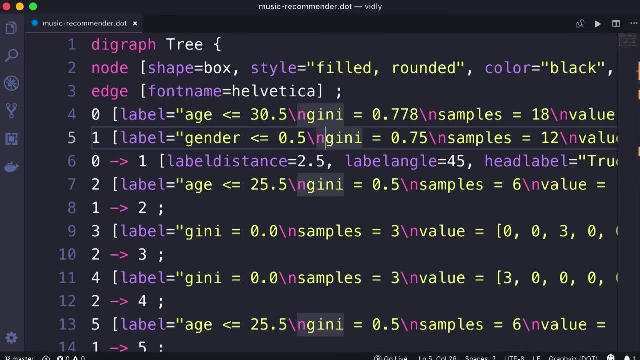 So we want to open this file with vs code. So drag and drop this into a vs code window. Okay, Here is the dot format. It's a textual language for describing graphs. Now, to visualize this graph, we need to install an extension in vs code. So on the left: 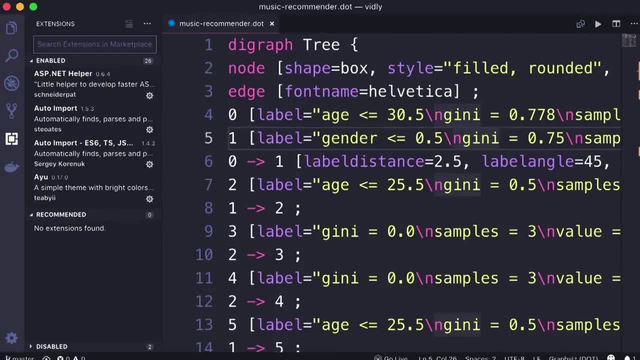 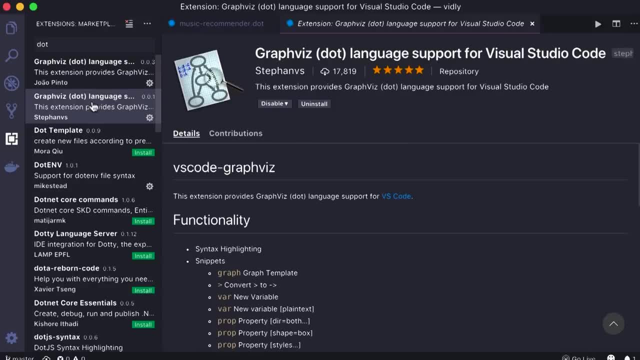 side. click the extensions panel and search for dot- dot. Look at this second extension here, Graphvis or dot language by Stefan vs. Go ahead and install this extension and then reload vs code. Once you do that, you can visualize this dot file. 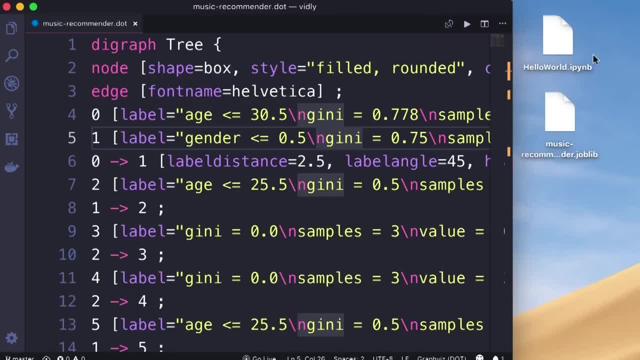 So let me close this tab. Alright, Look at this dot dot dot here on the right side. Click this. you should have a new menu Open preview to the site. So click that, Alright. here is the visualization of our decision tree. 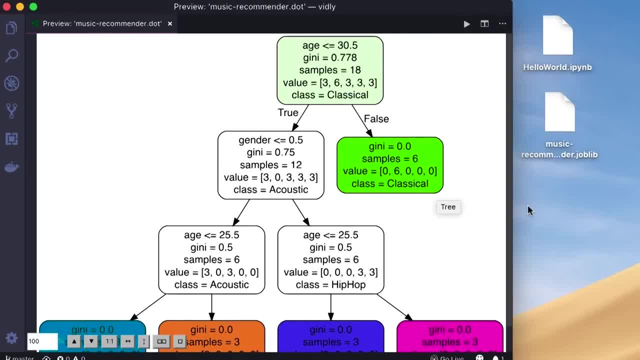 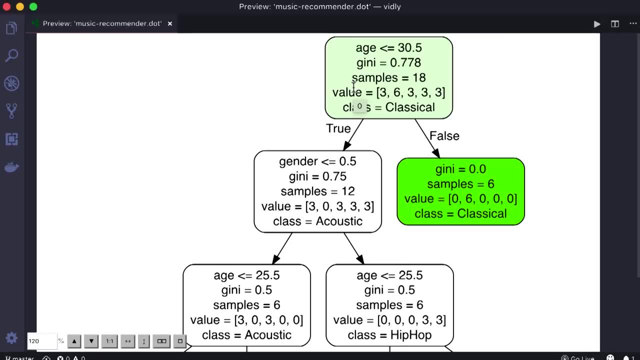 Let's close the dot file. There you go. This is exactly how our model makes predictions. So we have this binary tree, which means every node can have a maximum of two children On top of each node. we have a condition. If this condition is, 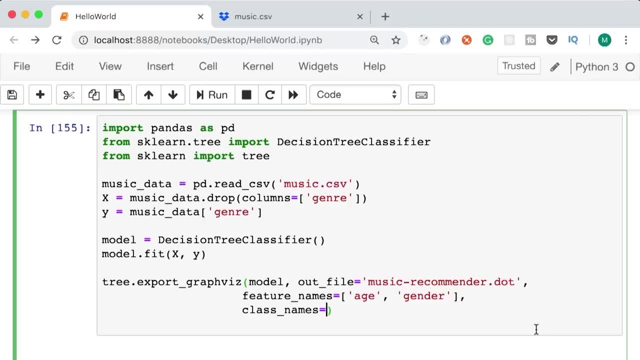 We should set this to the list of classes or labels we have in our output data set, like hip hop, jazz, classical and so on. So this y data set includes all the genres or all the classes of our data, but they are repeated a few times in this data set. So here we call. 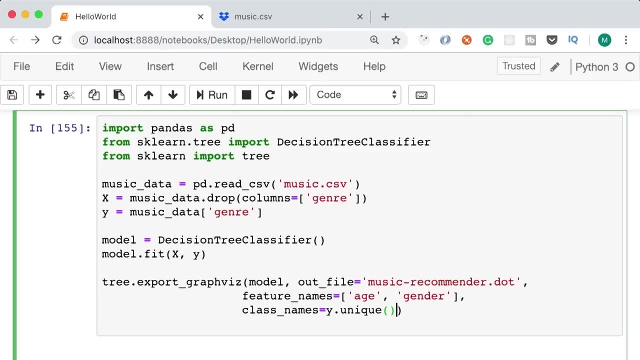 y dot unique. this returns the unique list of classes. now we should sort this alphabetically, so we call the sorted function and pass the result of y dot unique. The next parameter is label. we set this to a string all. once again, don't worry about the details of these parameters. we're going to come back. 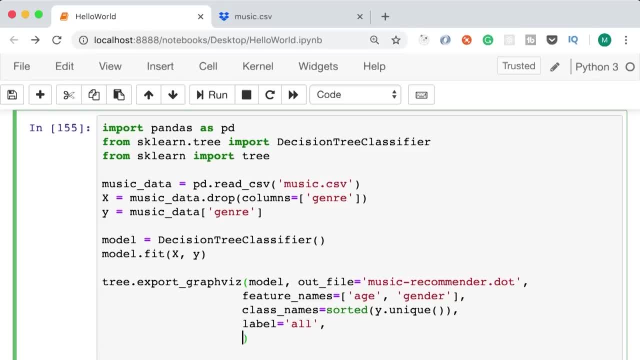 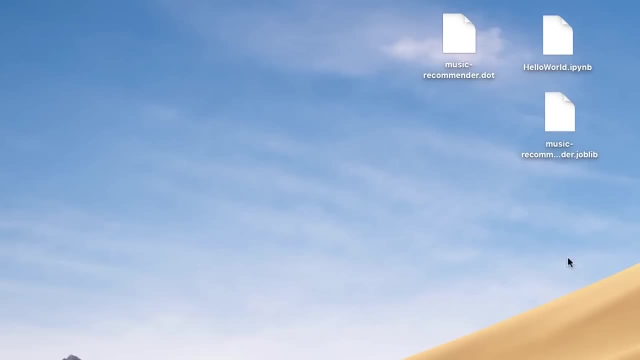 to this shortly. So set label to all, then rounded to true and finally filled to true. So this is the end result. Now let's run this cell using control and enter. Okay, here we have a new file. music recommender. 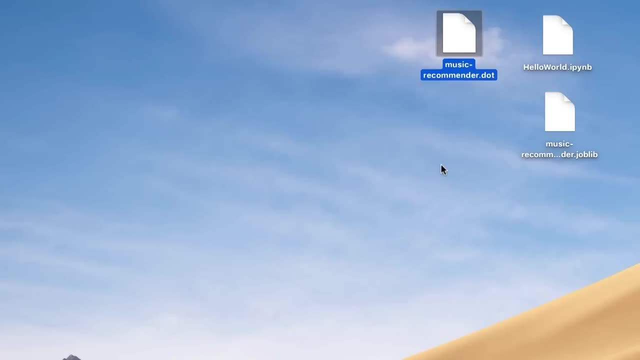 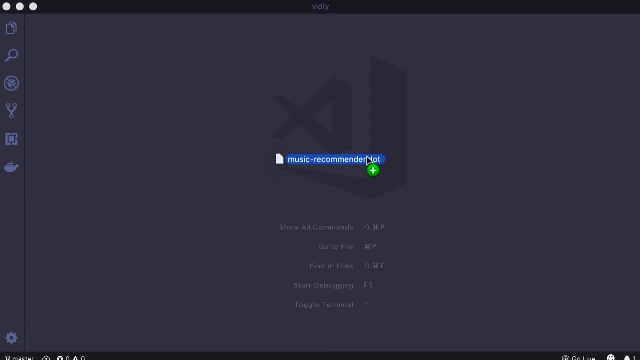 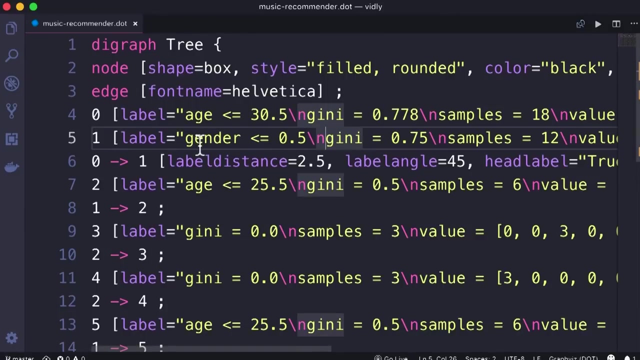 dot dot. that's a little bit funny. so we want to open this file with vs code. So drag and drop this into a vs code window. Okay, here's the dot format. it's a textual language for describing graphs. Now, to visualize this graph, we need to install an extension. 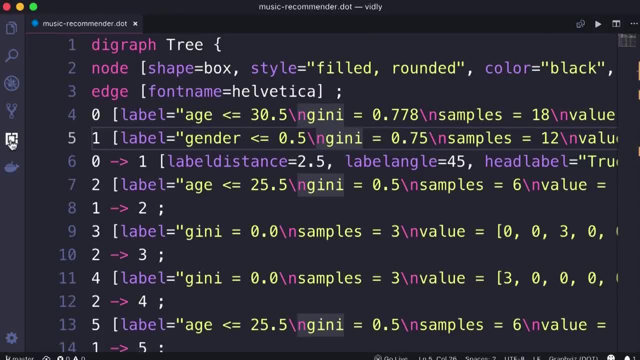 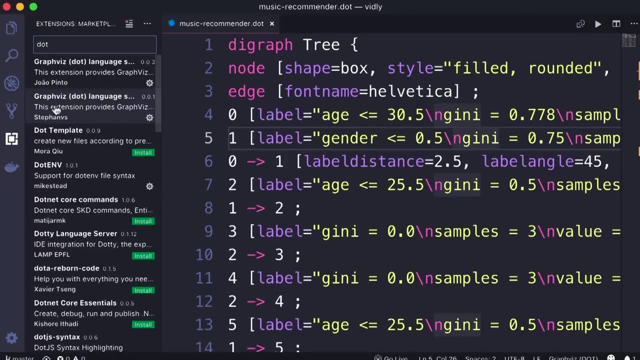 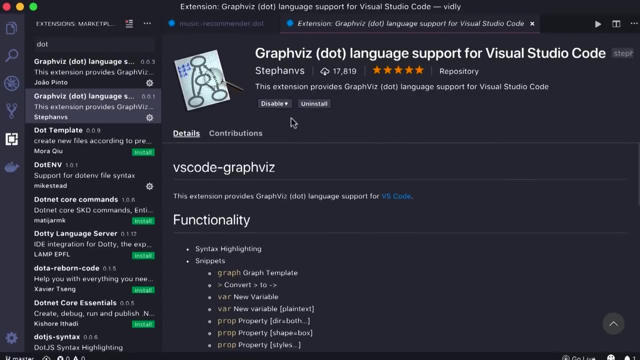 in vs code. So on the left side, click the extensions panel and search for dot d-o-t. Look at this second extension here, graph viz or dot language by a step of a finger. Go ahead and install this extension and then reload. 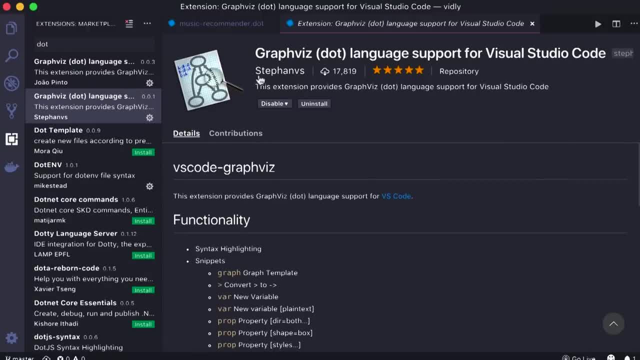 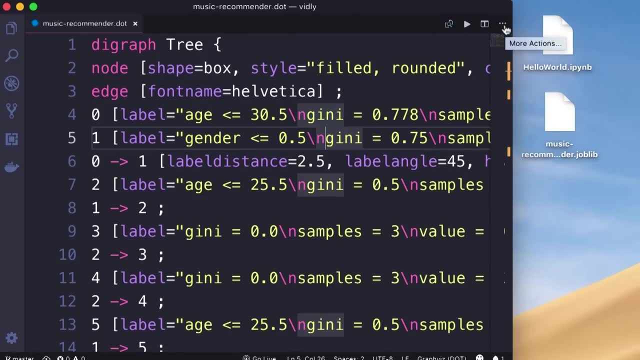 vs code. Once you do that, you can visualize this dot file, So let me close this tab. alright, Look at this dot dot dot here on the right side. click this. you should have a new menu open preview to the site, So click that. 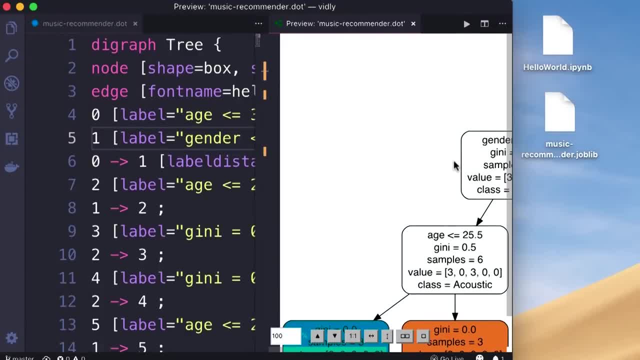 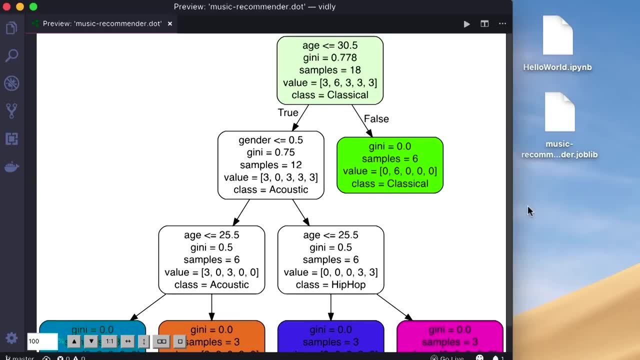 alright, here's the visualization of our decision tree. let's close the dot file. there you go. This is exactly how our model makes predictions. So we have this binary tree, which means every node can have a maximum of two children. 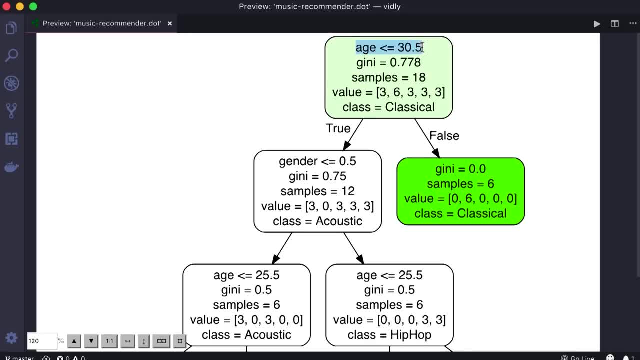 On top of each node we have a condition. if this condition is true, we go to the child node on the left side. otherwise, we go to the child node on the right side. So let's see what's happening here. The first condition: 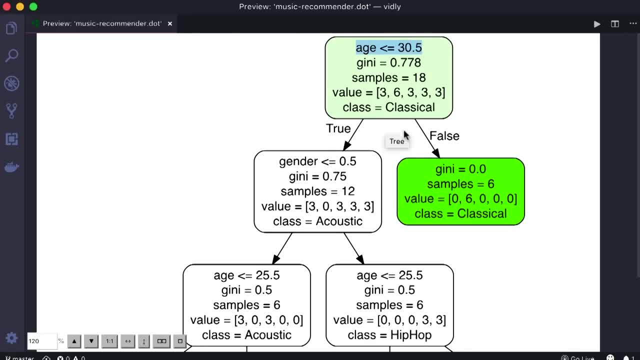 true, we go to the child node on the left side. otherwise we go to the child node on the right side. So let's see what's happening here. The first condition is age less than or equal to 30.5.. If this: 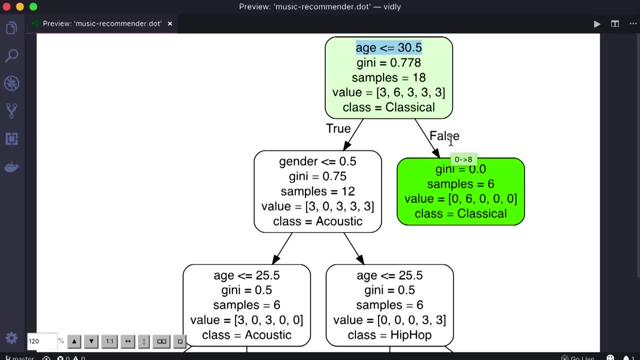 condition is false. that means that user is 30 years or older, So the genre of the music that they're interested in is classical. So here we're classifying people based on their profile. That is the reason we have the word class here. So a user who is 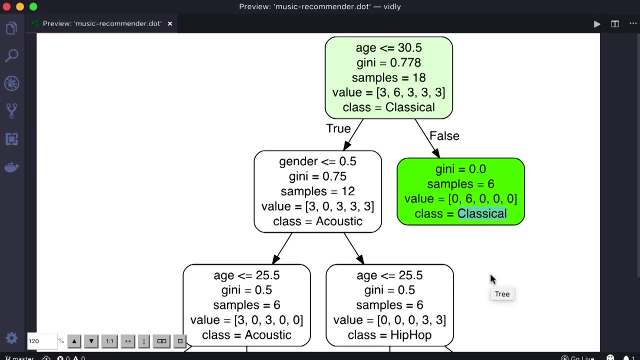 30 years or older belongs to the class of classical, Or people who like classical music. Now what if this condition is true? That means that user is younger than 30. So now we check the gender: If it's less than 0.5,. 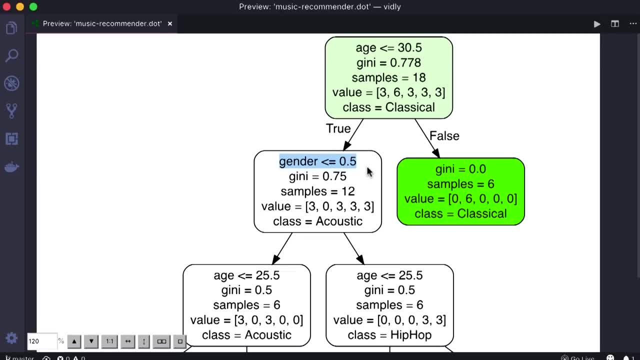 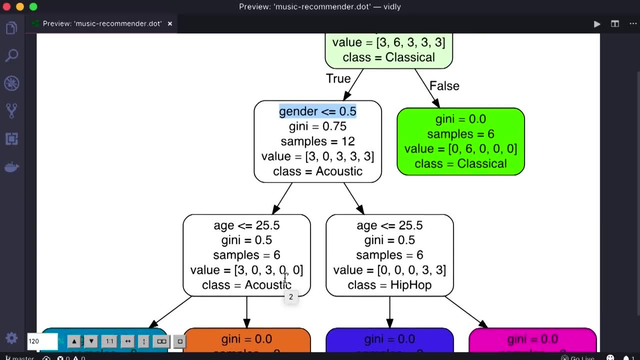 which basically means, if it equals to 0, then we're dealing with a female. So we go to the child node here. Now, once again, we have another condition. So we're dealing with a female who is younger than 30.. 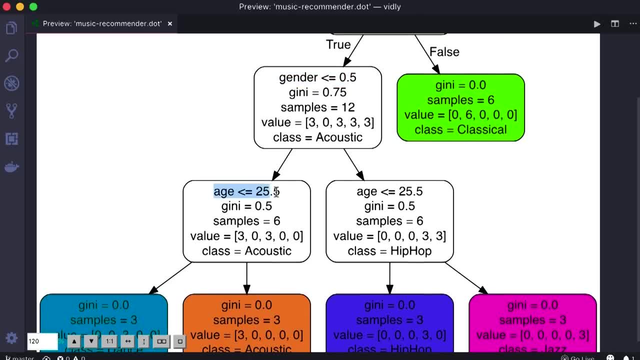 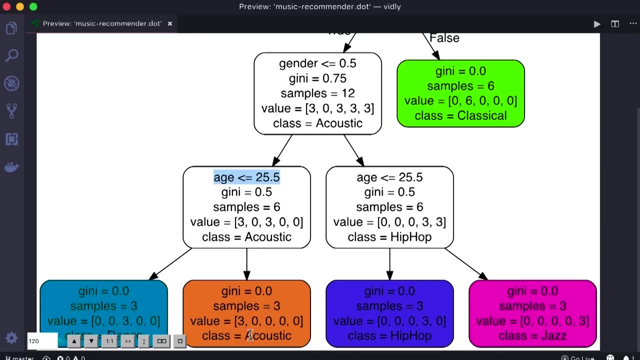 Once again, we need to check their age. So is the age less than 25.5?? If that's the case, then that user likes dance music. otherwise they like acoustic music. So this is the decision tree That our model uses to make predictions. Now, if you're wondering why, 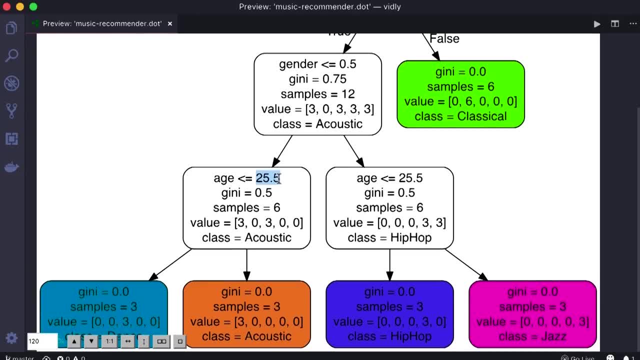 we have these floating point numbers like 25.5,. these are basically the rules that our model generates based on the patterns that it finds in our data set. As we give our model more data, these rules will change, so they're not always the same. Also, the more columns- 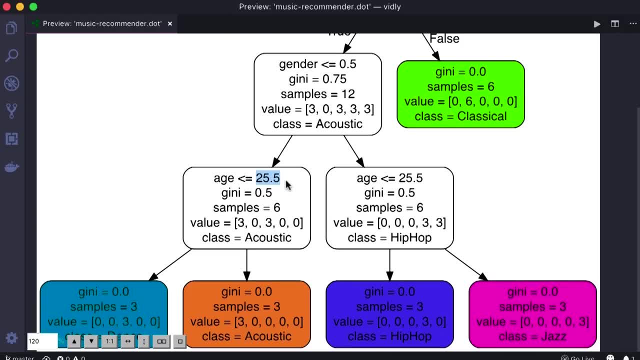 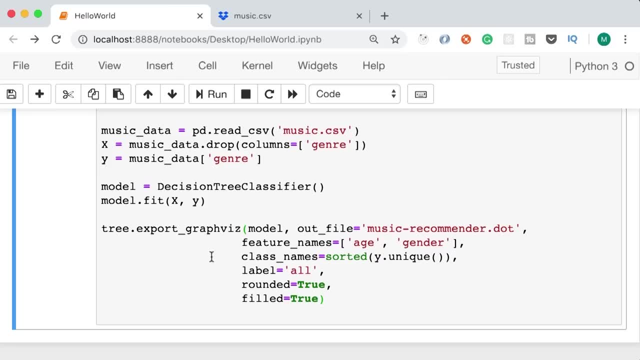 or more features we have. our decision tree is going to get more complex. Currently we have only two features: age and gender. Now back to our code. let me quickly explain the meaning of all these parameters We set filled to true, so each box or each node is filled with a color. 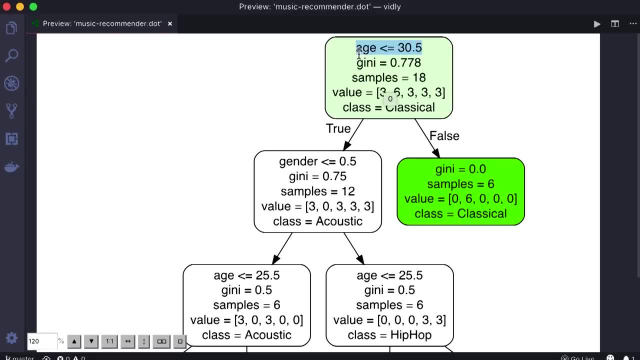 is age less than or equal to 30.5.. If this condition is false, that means that user is 30 years or older. so the genre of the music that they're interested in is classical. So here we're classifying people based on their profile. 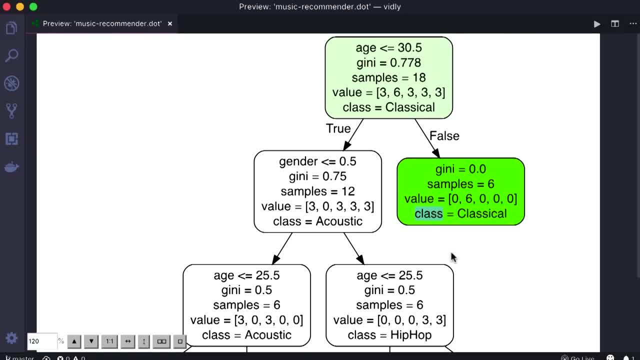 That is the reason we have the word class here. So a user who is 30 years or older belongs to the class of classical Or people who like classical music. Now what if this condition is true? that means that user is younger than 30.. 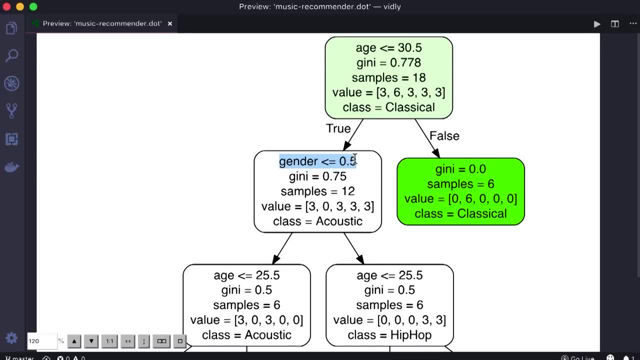 So now we check the gender. if it's less than 0.5, which basically means that user is older than 30, means if it equals to 0, then we're dealing with a female. So we go to the child node here. now, once again, we have another condition. 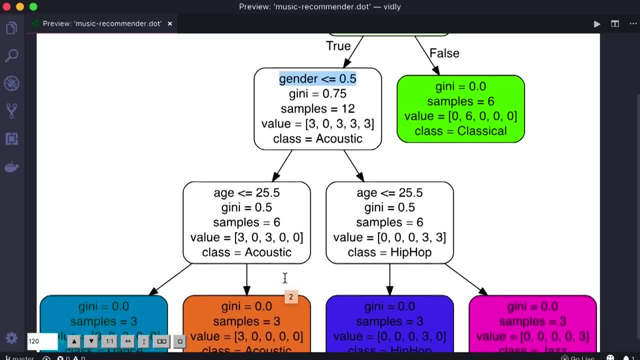 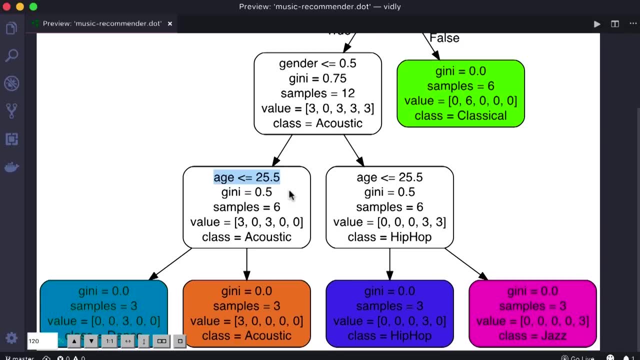 so we're dealing with a female who is younger than 30. Once again, we need to check their age. So is the age less than 25.5?? If that's the case, then that user likes dance music. otherwise they like acoustic music. So this is the. 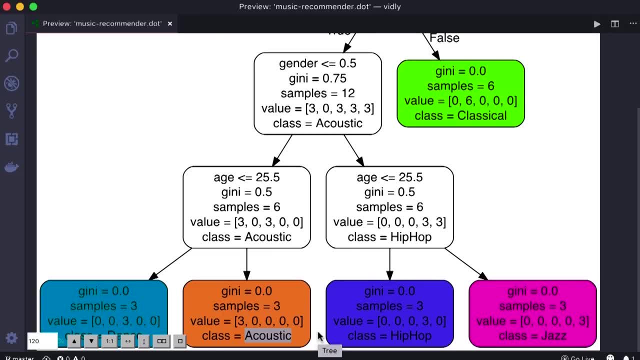 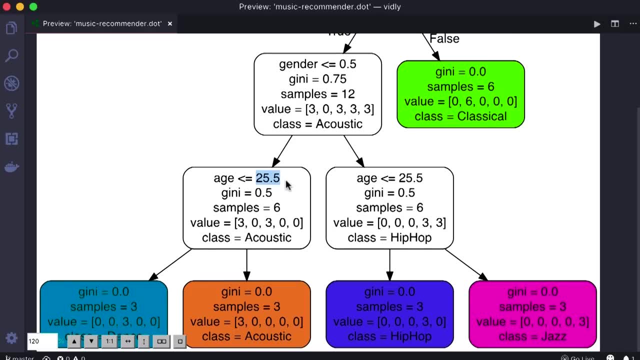 decision tree that our model uses to make predictions. Now, if you're wondering why we have these floating point numbers like 25.5, these are basically the rules that our model generates based on the patterns that it finds in our data set. As we give our model more data, 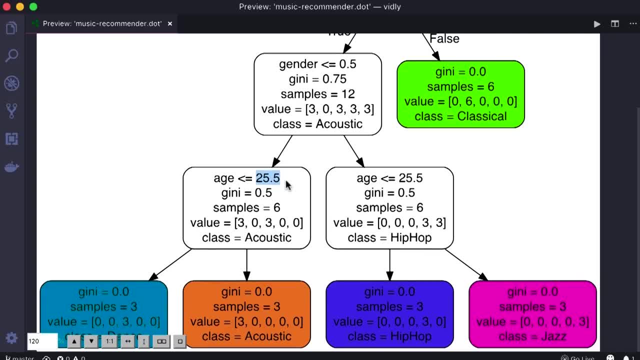 these rules will change, so they're not always the same. Also, the more columns or more features we have, our decision tree is going to get more complex. Currently, we have only two features: age and gender. Now back to our code. let me quickly explain the meaning of all these parameters. 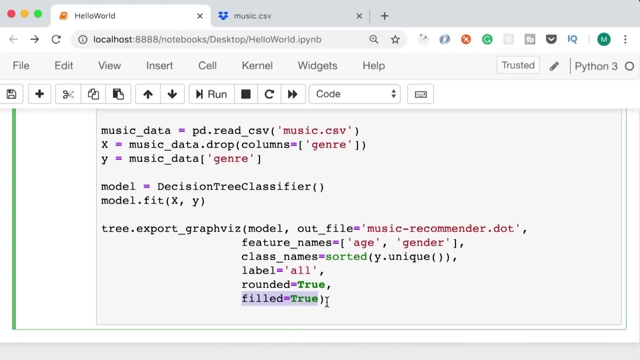 We set filled to true, so each box or each node is filled with a color. We set rounded to true, so they have rounded corners. We set label to all, so every node has labels that we can read. We set class names to the. 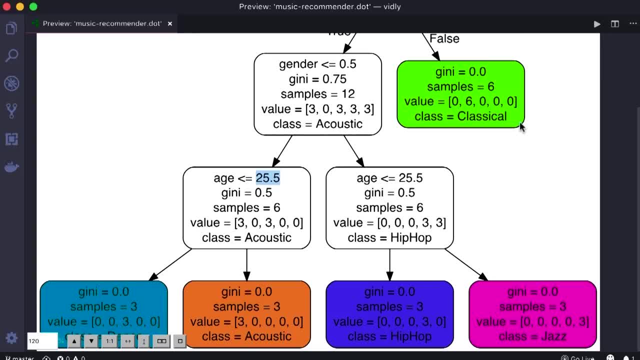 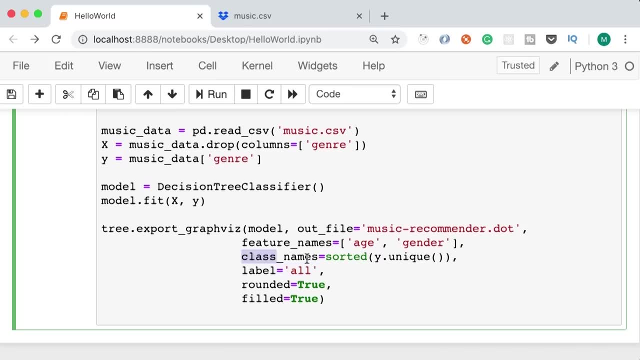 We set rounded to true, so they have rounded corners. We set label to all, so every node has labels that we can read. We set class names to the unique list of genres and that's for displaying the class for each node, right here. 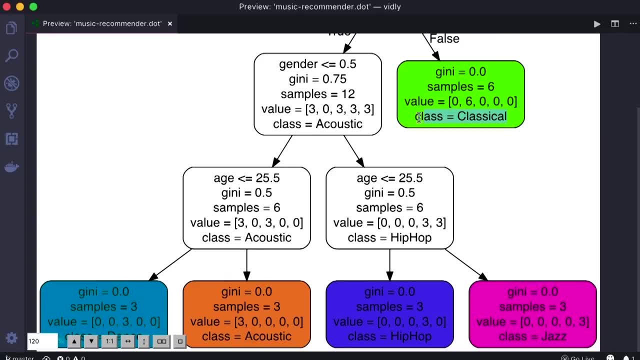 unique list of genres and that's for displaying the class for each node right here, And we set feature names to age and gender so we can see the rules in our nodes. Hey, thank you for watching my tutorial. I hope you learned a lot and you're excited to learn more.